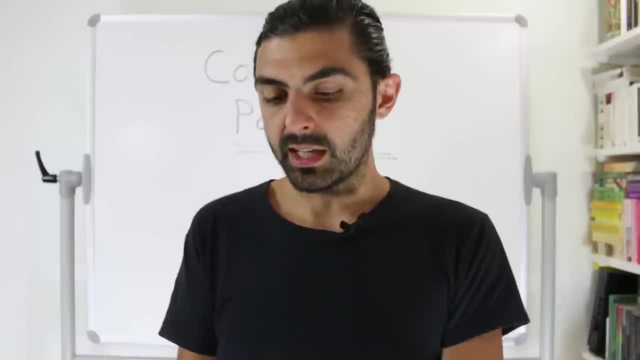 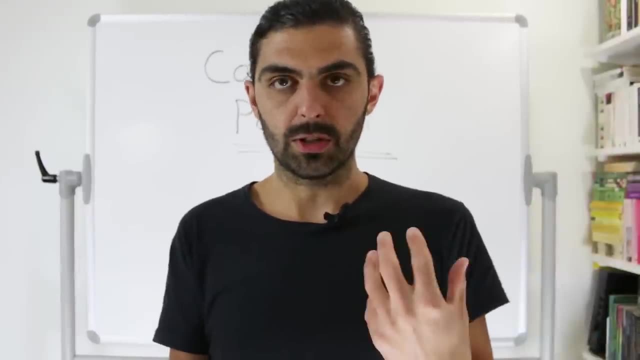 other objects with these command objects. So you can now have things that are sets of commands, So you can have a list of commands that you're about to execute, or you can have a collection of commands that you execute when you press different buttons, And this 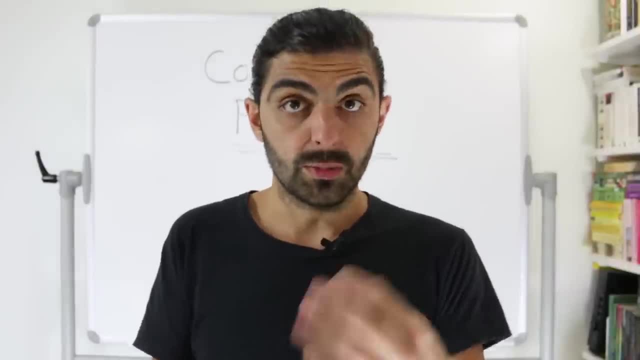 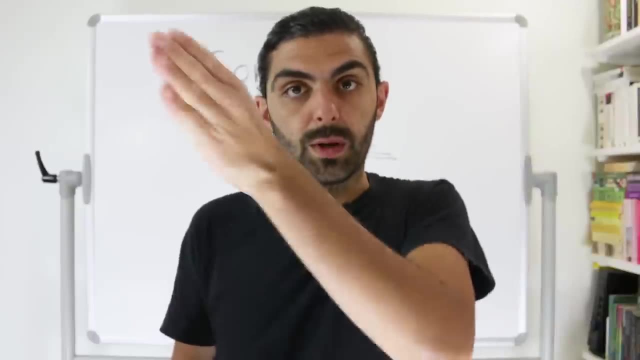 is kind of what we'll talk about later. And when they talk about queue here, I assume that then they mean this thing about a list. So you take a bunch of commands and you put them in a list and then you invoke the commands one by one, by one, by one, right? So then you have a queue of commands that you execute. 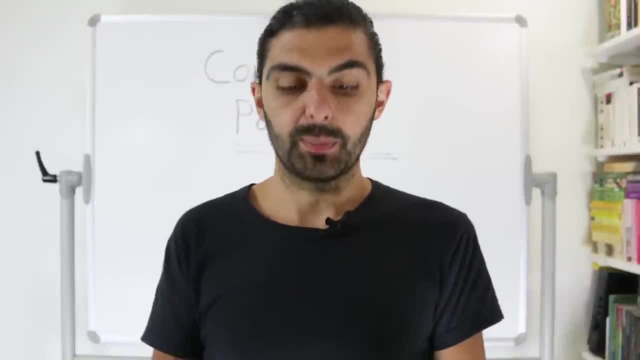 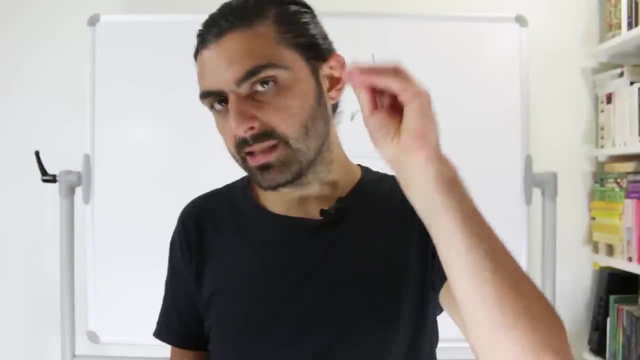 Or we haven't talked about composite pattern yet, but with composite pattern you could even make like a batch command, So you can have a command that contains multiple commands, such that when you execute this sort of batch command or this macro command, that macro command simply executes. 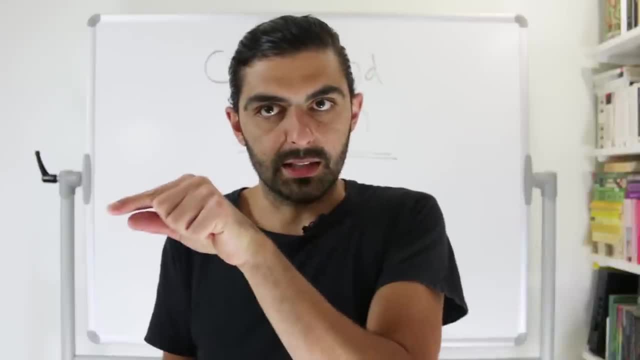 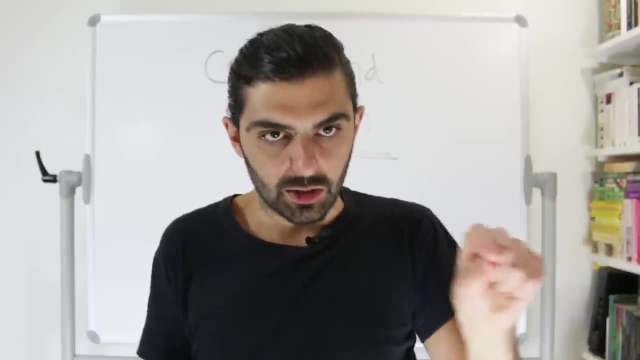 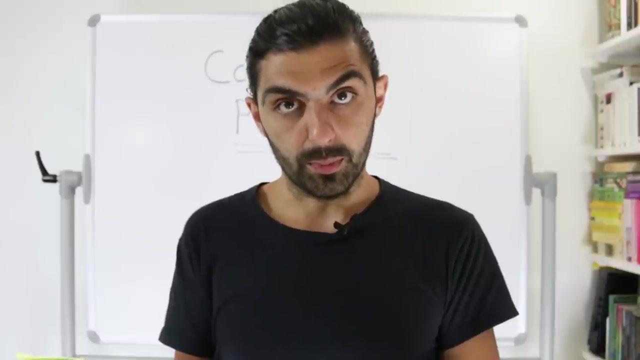 a bunch of different smaller commands. So you have many commands that's owned by a larger macro command And when you say execute on that macro command, that macro command executes all of the smaller commands. But we're getting totally ahead of ourselves. The last portion of this definition was: and support undoable operations. 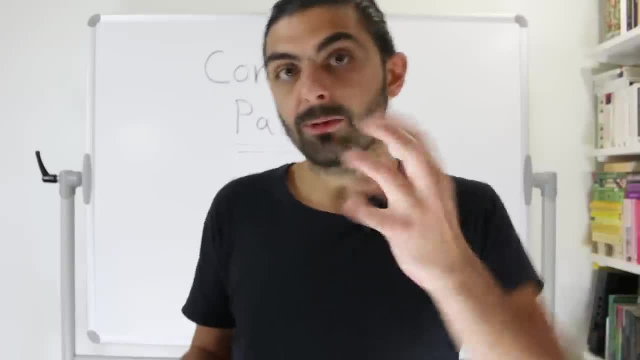 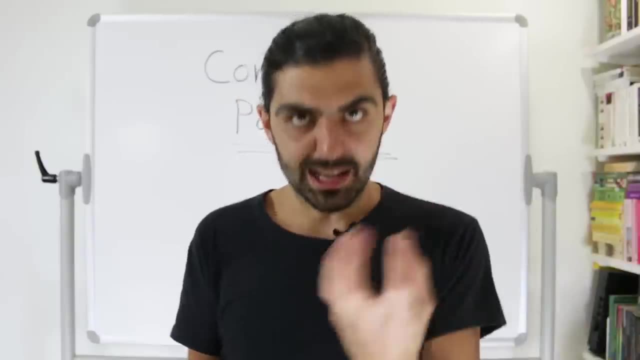 So if you think about it, if you have a command that does something, the inverse of that command, the anti thing of that command, is an undo right. So if I say I have a command that adds one, then the inverse of that has to be that the undo 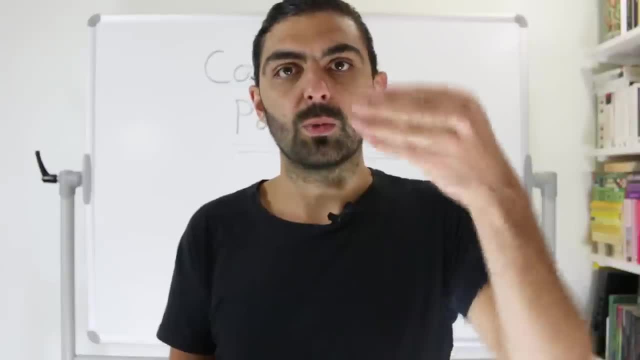 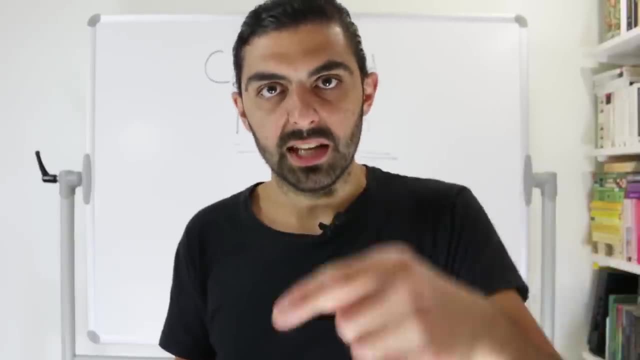 do. a definition of that command is that you subtract one. so if i have then a command that can, that does something, and it also supports an undo, which is the inverse of itself, then i can very simply call the command and then undo the operation by calling undo on that command. right. 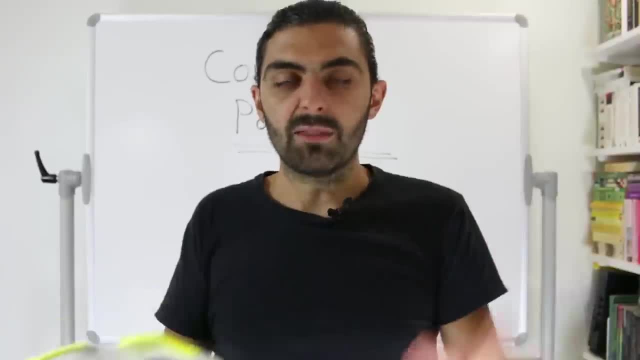 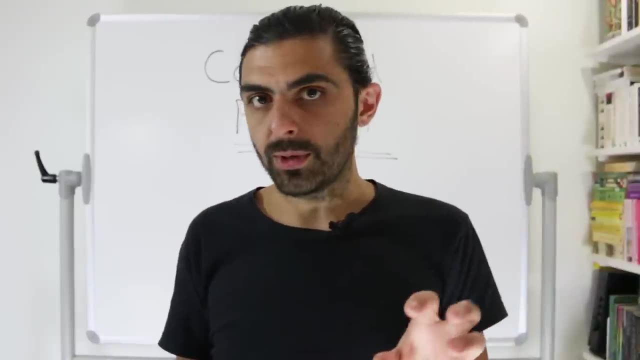 i added one and then i subtract back and if you have a bunch of different commands that have encapsulated different actions and all of them follow this logic that they, all of them have these undo operations, then it's very simple to to implement, uh, very complex undo operations because 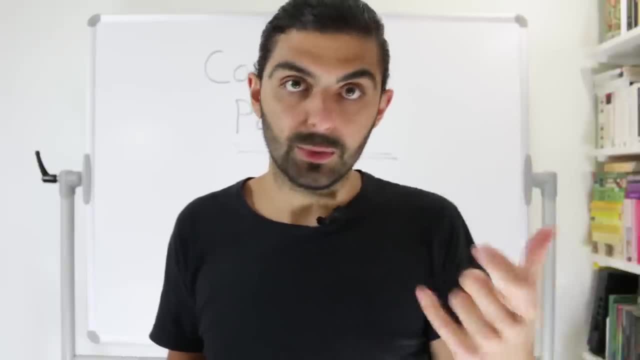 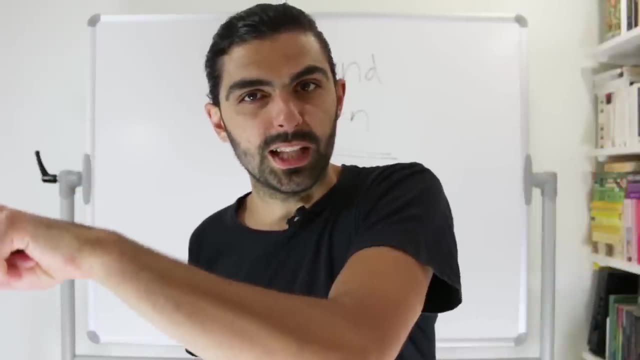 all of the different actions, all of the different commands are responsible for undoing themselves. so, even if you have a queue of actions, even if you have a queue of commands that you execute in in series, you can undo backwards because if you, if you undo them in the opposite order of which of 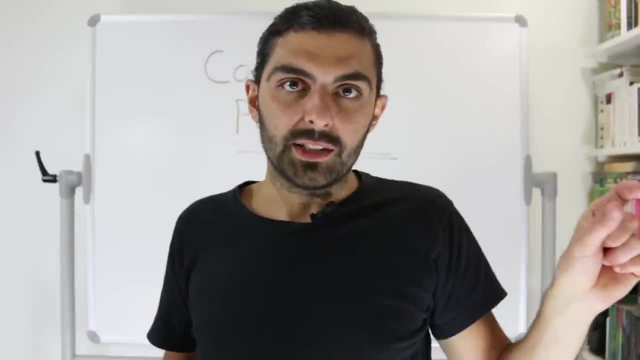 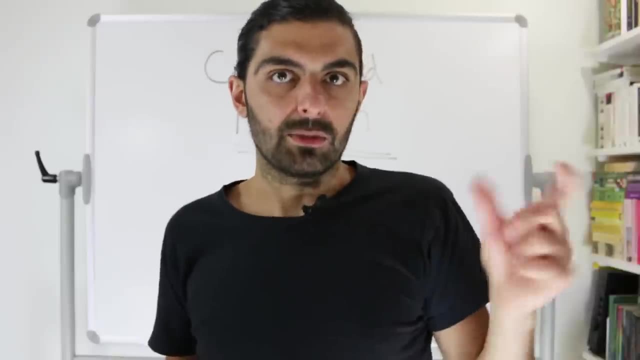 the order in which you executed them, then you would end up at the start, right? so you have this series of commands, you have this list of commands that you're executing one by one, by one, by one. so like, let's think about math, right, let's say that you have something which is like: okay, add one at 10. 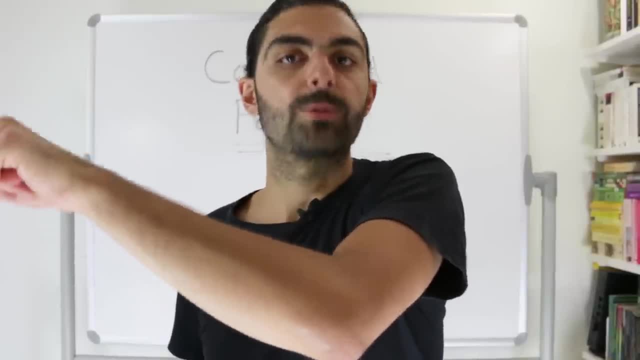 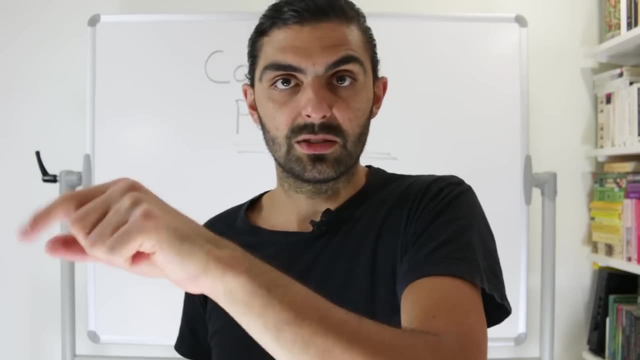 at 20, at 40, etc. and then you have undo versions of that right. so every command has its own implementation of what it means to undo itself. so then would be like subtract 40, subtract 30- i can't remember what i said about the other numbers- but like the inverse of that. but again, 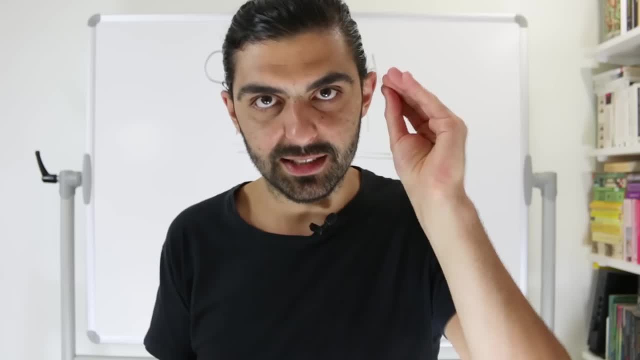 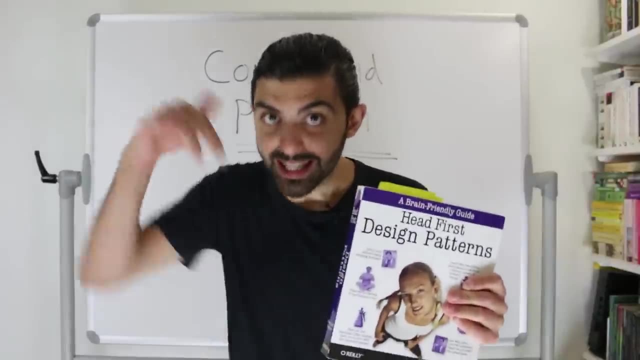 we're getting super ahead of ourselves. so so, so let's stop here and and let's dig into it, and then let's get back to these points. now, if you're new to this channel or playlist, i just want to say that what we're doing in this playlist is that we're walking through all of the patterns in this. 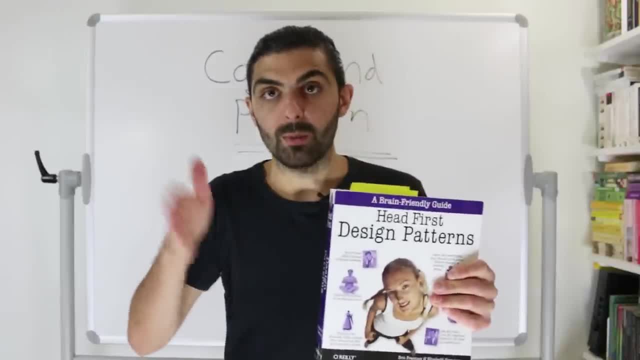 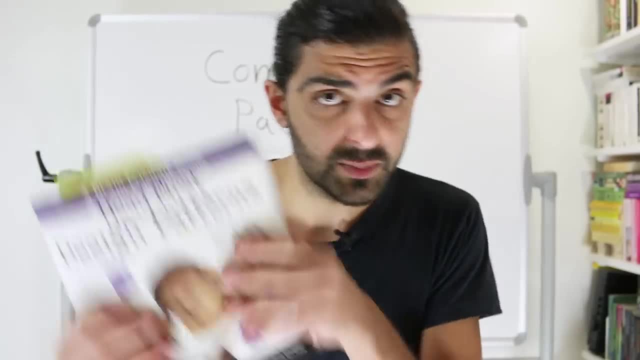 book headfirst design patterns one by one, by one by one. so if you're not already subscribed now, it's a super good time to subscribe so that you won't miss the next pattern. beyond that, this book headfirst is a super good book if you're new to design patterns, so i highly recommend that. 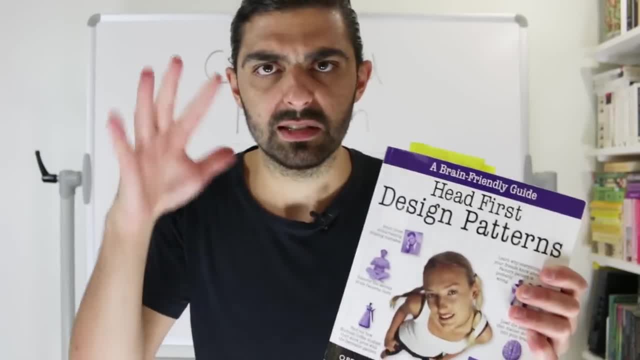 you get it if you're studying design patterns. it has tons of images and silly examples and all of that. so it's not just a single pattern, but it's a ton of images and silly examples and all of that. so it's not just like a dictionary. it actually tries to help you understand these patterns by giving you some 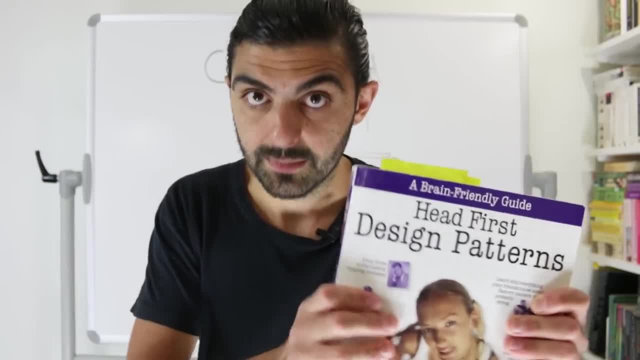 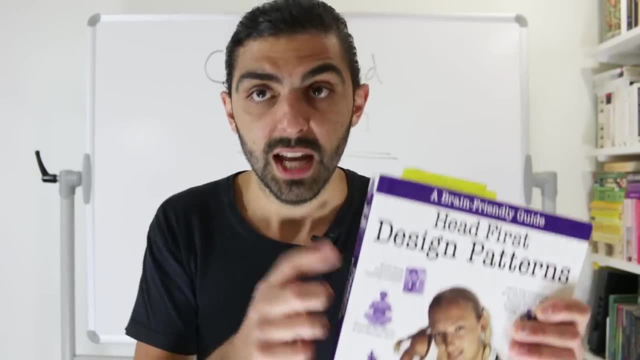 context and rationale and like narrative, so highly recommend it. however, if you're not new to design patterns and you're more looking for like a reference book or like a dictionary of design patterns, i wouldn't recommend this book. instead, i'd recommend this book: design patterns- elements. 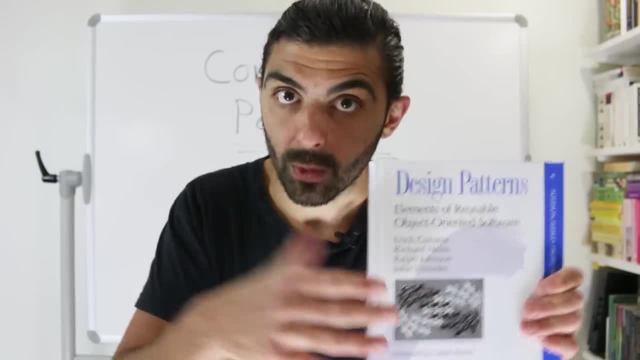 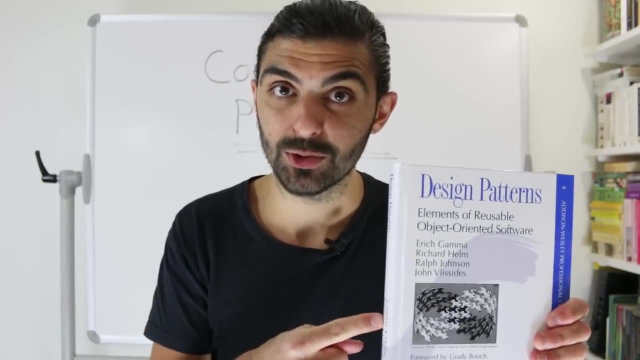 of reusable object-oriented software by gang of four. so this is like the de facto classic design patterns book. so if nothing else, this is something that's really good to put on your bookshelf for the future so you can go back and refer to this. super good, i use this as a reference book. but 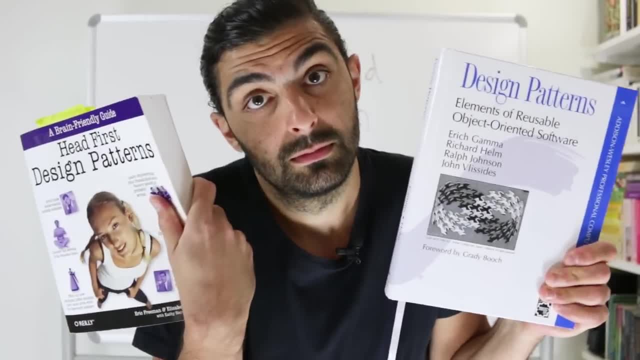 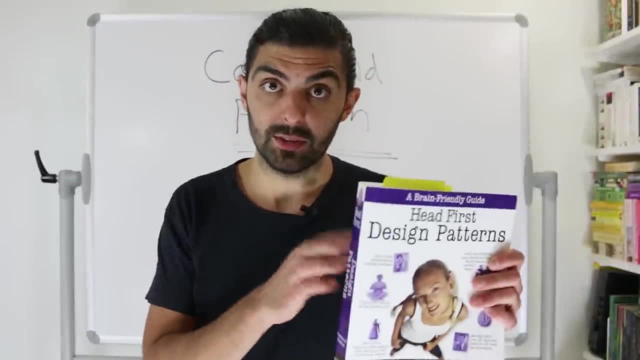 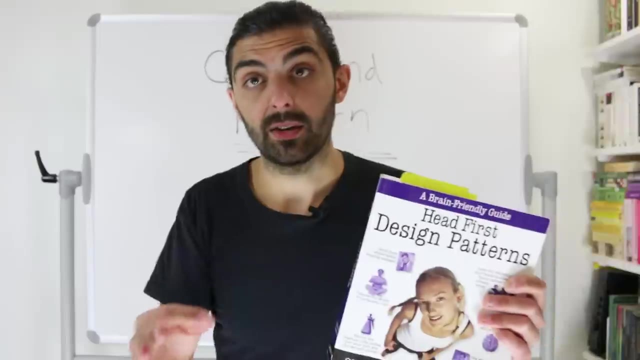 if you're like me, i mean get both. but now let's get into the command pattern. so if you've seen my other videos, you know that i've got some varying opinions about the examples from this book. some of them are superb and some of them not so much. the example for command pattern: i actually find extremely suitable and and it's not something like you should be using. for example, if you're using a modern book layout or a monogram layout, for example, you're starting with your book layout, and if you're using your book layout, for example, you're starting with a modern work layout or you're. 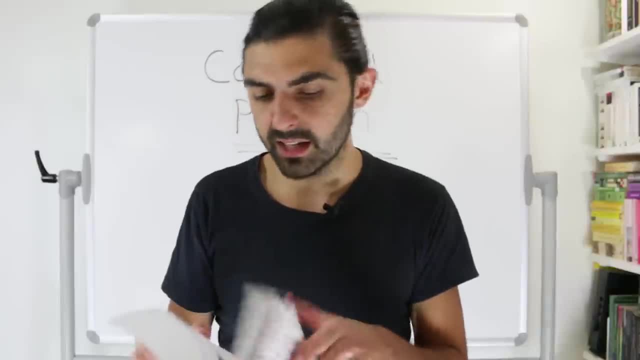 gonna start with a modern book layout, or you're going to start with a modern book layout or you're, And kind of logical, I mean, it kind of makes sense. And actually I mean I don't know when this book was written, like probably more than a few years ago. 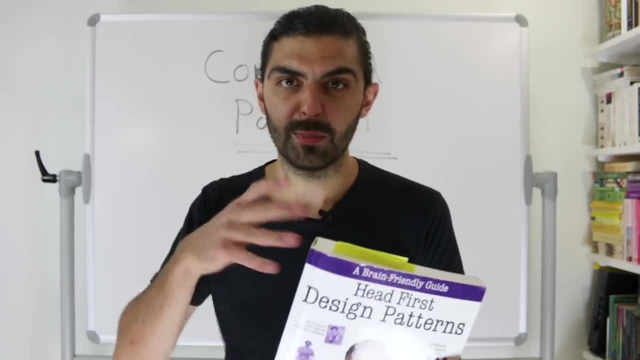 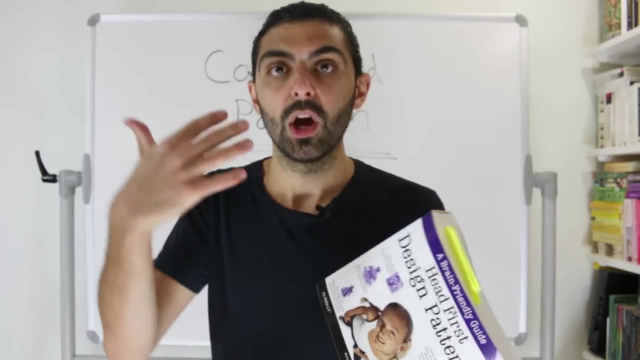 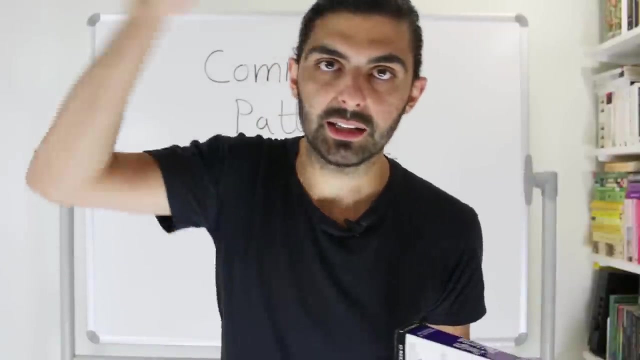 But I would actually say that this example kind of becomes more and more relevant. Maybe the pictures are a bit outdated, but the example is super relevant. So what they talk about is: they talk about smart homes, They talk about home automation. So think about like you have Wi-Fi-connected light bulbs and a Wi-Fi-connected coffee machine. 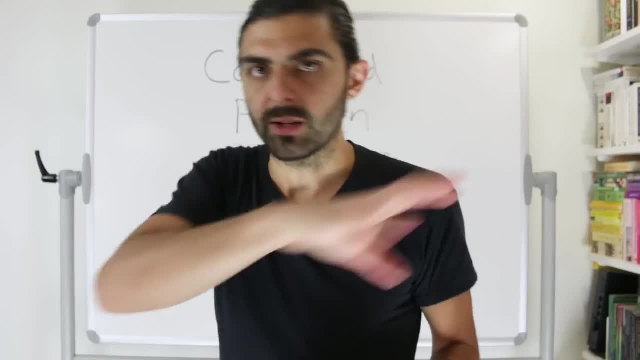 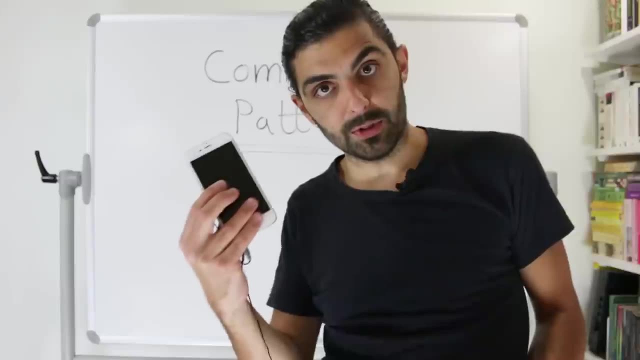 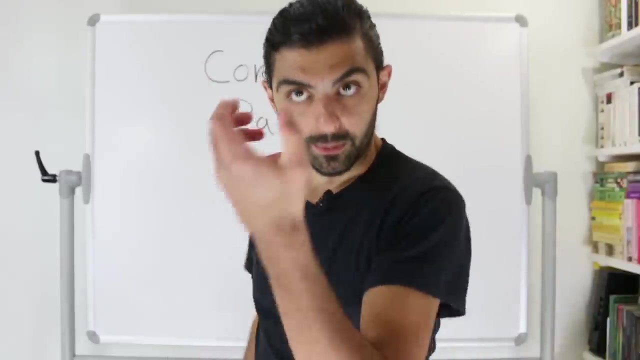 And your thermostat is connected and like all of this stuff right. More and more of the appliances in your home become smart devices that you can control from your smartphone or from some other device. Essentially, you put them all on your network and you can control them remotely, either from your home via your own Wi-Fi or via the Internet back to your home. 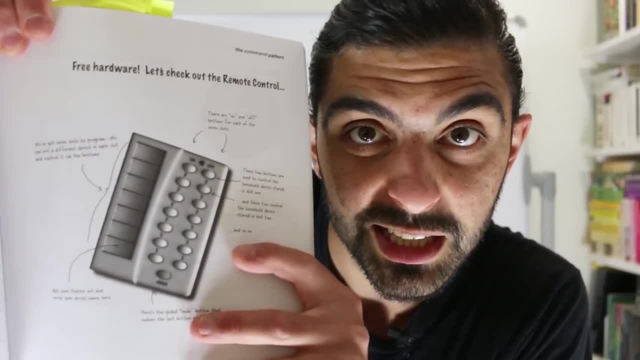 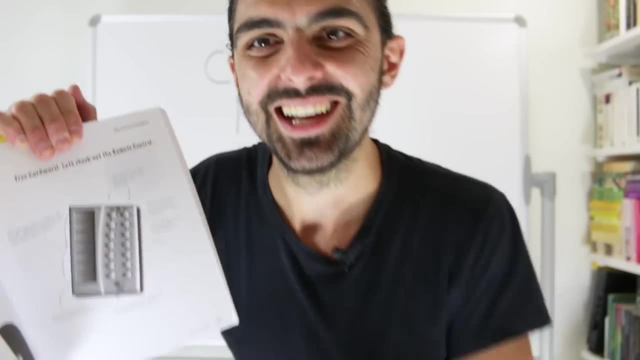 So they've got this example of this remote control that looks, I mean, completely like 1990s, 1980s, I don't know, like super old, right, But anyway I mean let's follow the same example. 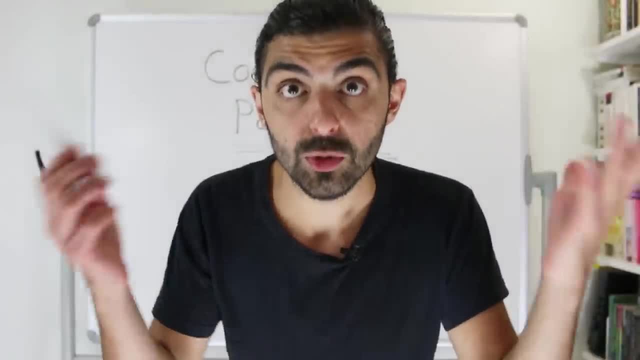 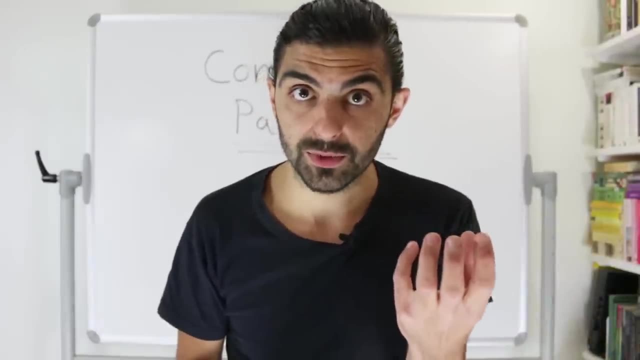 Let's try to modernize. So in my home I've got Philips Hue lights. You're probably already familiar with Philips Hue or some equivalent, but it's essentially Wi-Fi-connected light bulbs, Or I don't know if it's Wi-Fi, but they connect to your router somehow. 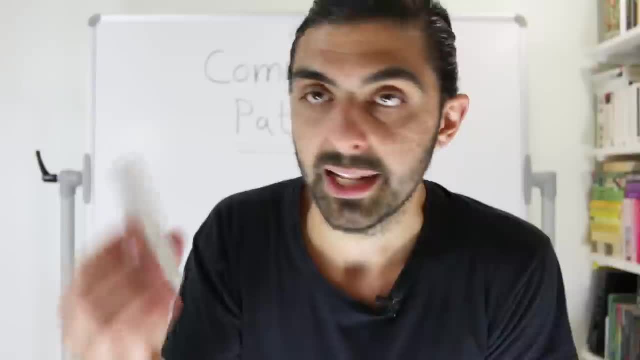 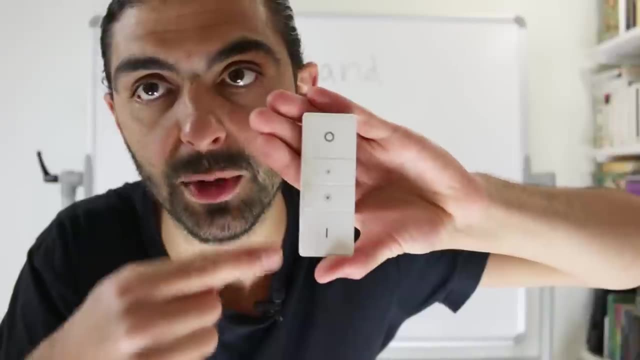 So one of the things I've got in my home is this controller, And usually it's on a wall, but I figured this makes a very good example. So if you check this out, you can see that we've got four different buttons on this. 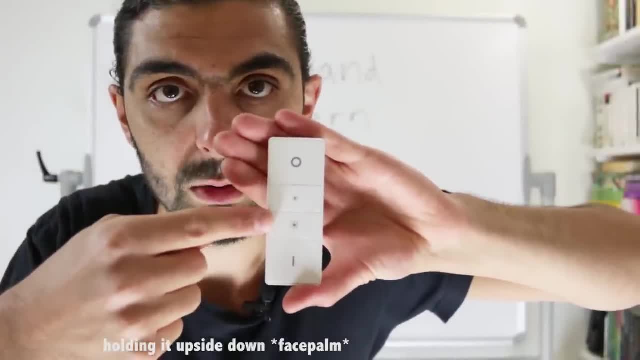 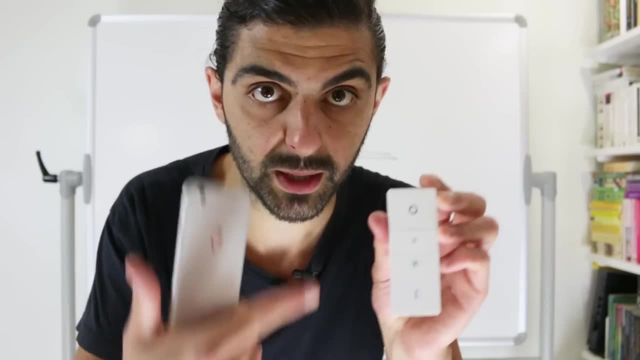 So we've got on Dim up, dim down and turn off. The thing about this controller is that, via the Philips Hue app, I program these different buttons to be connected to different lights, So let me just show you how it works. 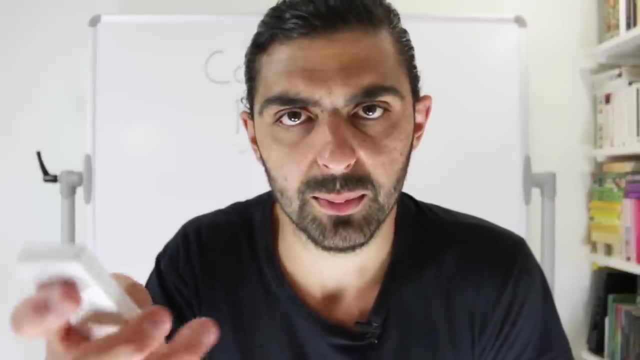 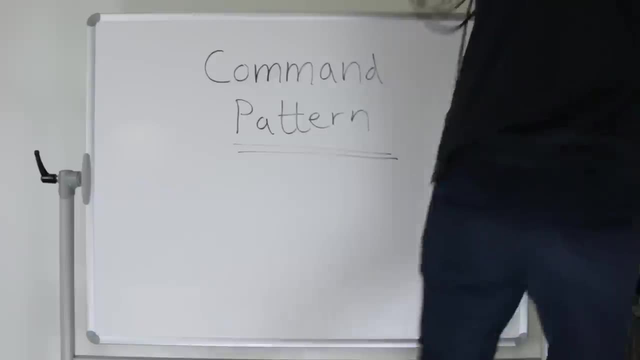 So most of the lights are on now, but I'm not sure this is going to be visible on camera. But if I press off On, Yeah, that's hardly visible. Let me do this. Wait Off On On. 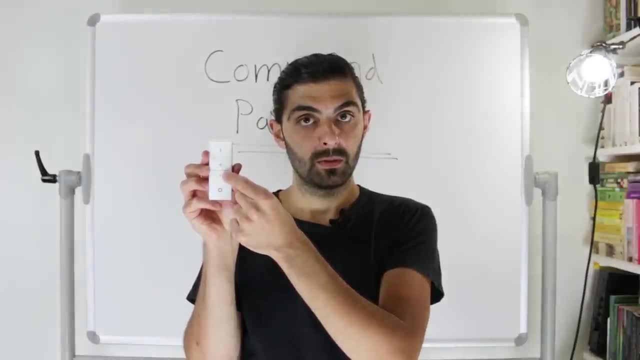 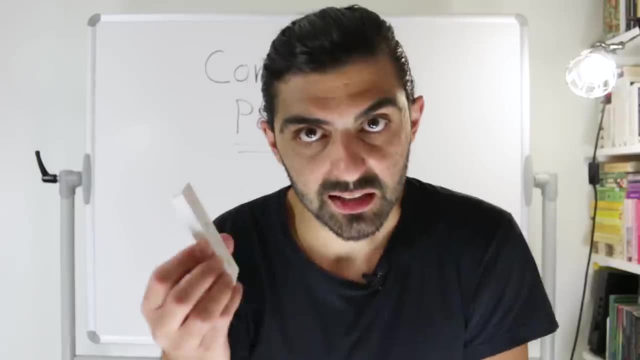 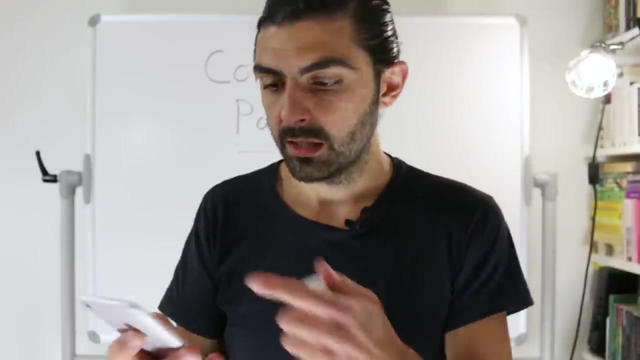 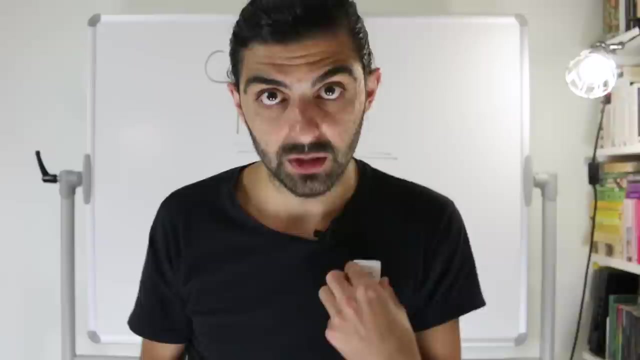 Dim Down. I think you get the point. So here's the scenario, slightly adapted from the book. Let's say you're running a company and you are tasked with building the smartphone app that users like me use to program this device. In other words, when I press on here, I might want a different thing to happen than when you press on on your device. 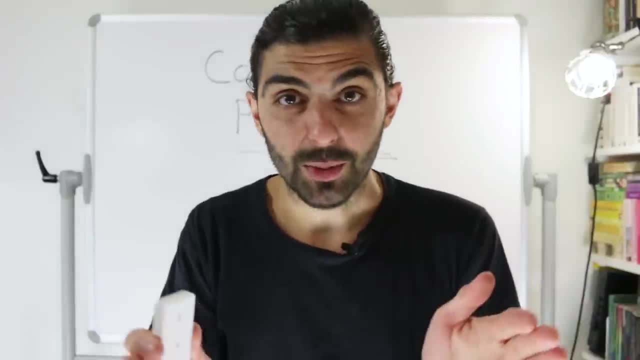 By the way, let me just mention that Philips Hue- This is not at all a paid endorsement, but if you've got the money to spend, it's totally awesome. But that's completely out of context for this video. so let's move on. 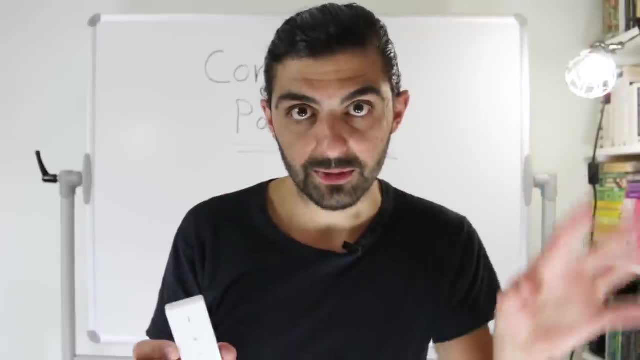 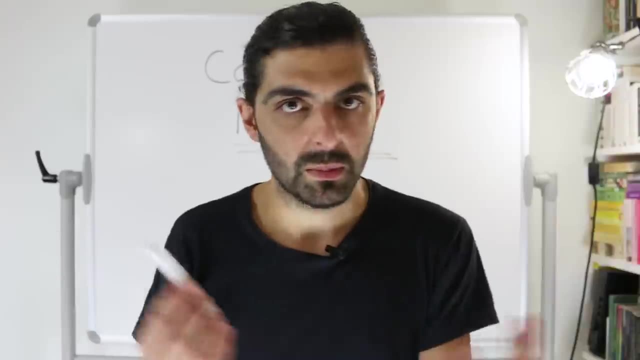 You can think about it this way, for example. So I have lots of different Philips Hue bulbs in my home, and some of them are light strips. some of them are in different rooms, some of them have color, some of them don't have color. 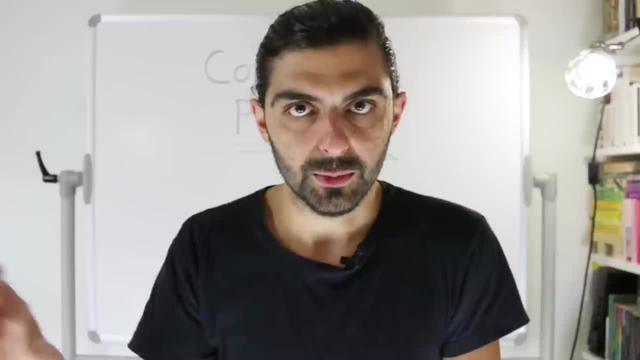 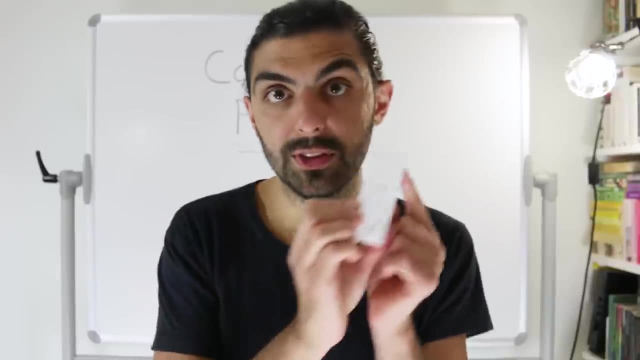 And if I buy multiple of these controllers and then put them in different rooms? one way of thinking about this would be that I would want the on button to turn on lights per the room that they're in, Turn on the lights of the room in which this particular controller is in. 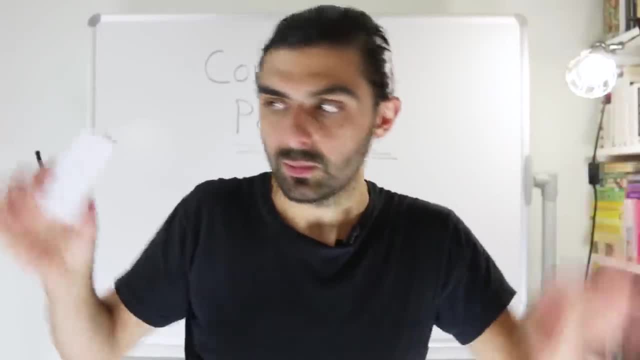 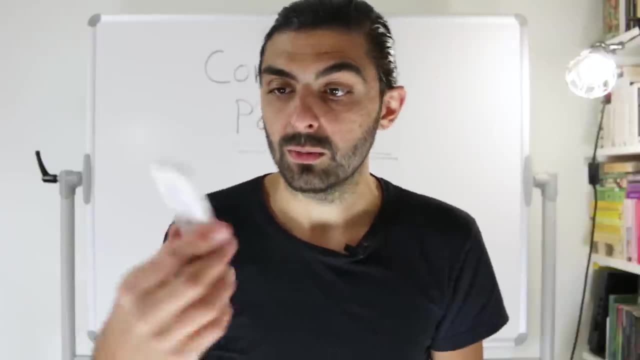 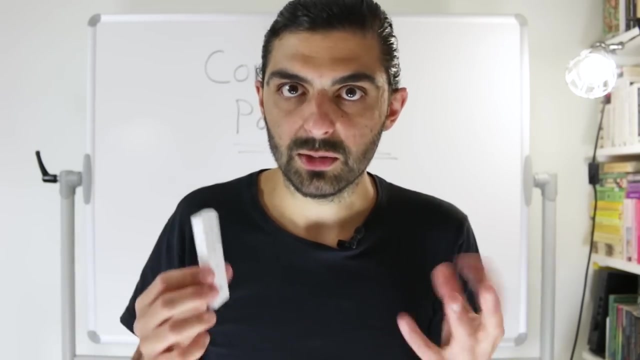 But it could also be that I have like two sections in one room, so I would want to have one controller for half of the room and another controller for the other half of the room, Or now I'm going beyond what's actually supported by this particular control, but I'm just thinking like if we would design this application from scratch, these kind of things would probably make sense. 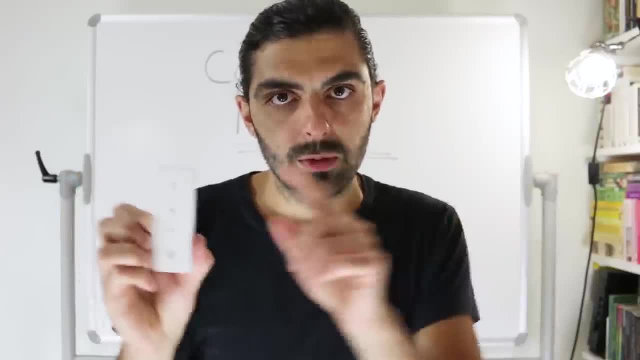 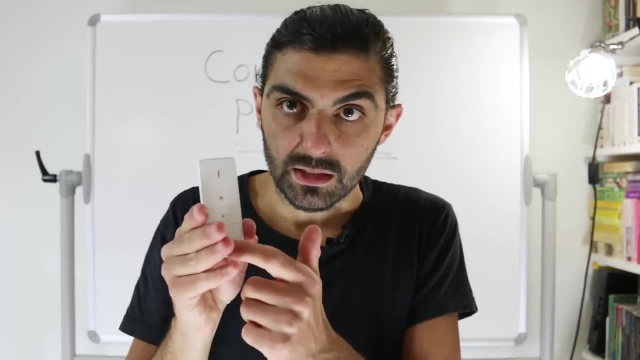 Or potentially I would want it this way. I would want like I have two controllers. the on button of one controller controls half of the room. The on button of the other controller controls the other half of the room, But the off button controls turns off the lights in the whole room, right. 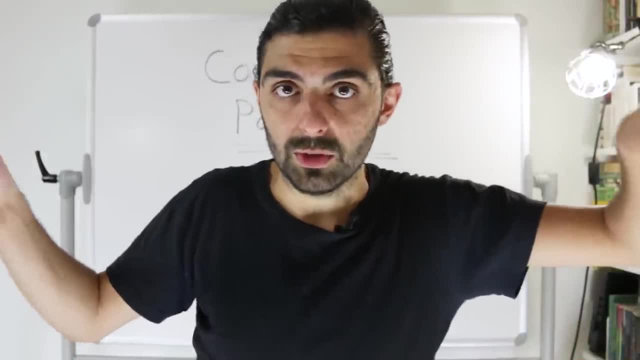 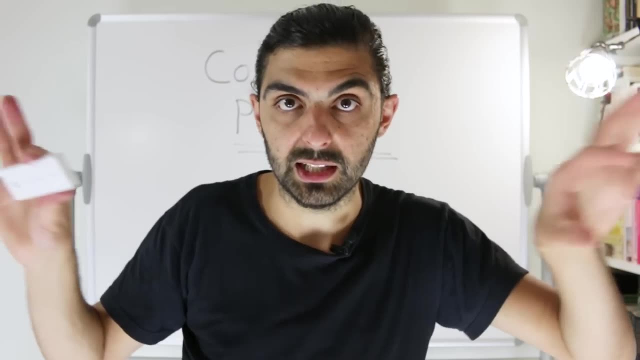 That scenario also makes a lot of sense, right? It's like, wherever you are in the room, you want to be able to turn off the lights because you're leaving, but there are two physical portions and you want to be able to control them separately. 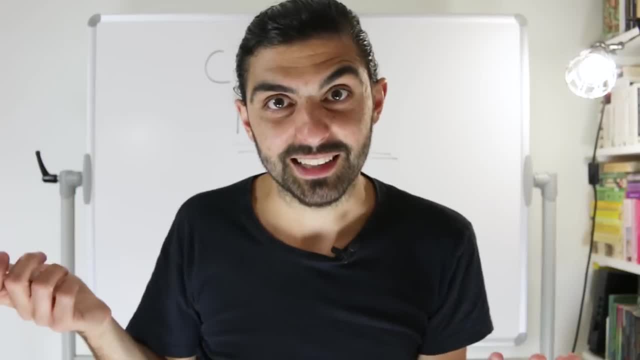 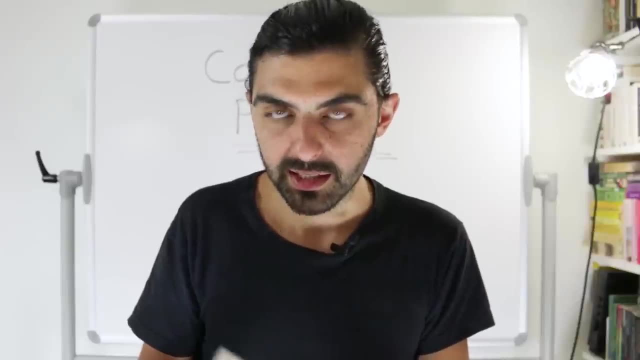 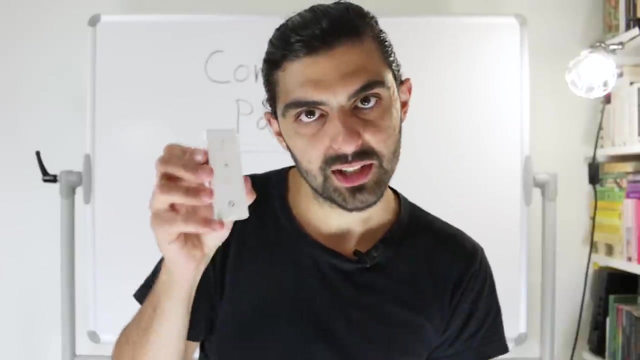 Let's say like one is the office part and one is the leisure part, or something like that. So when you're building this kind of application, the word dependency injection should really come to mind, right, Because we're saying that the actions of any particular button here can't be hard coded into the class representing this control. 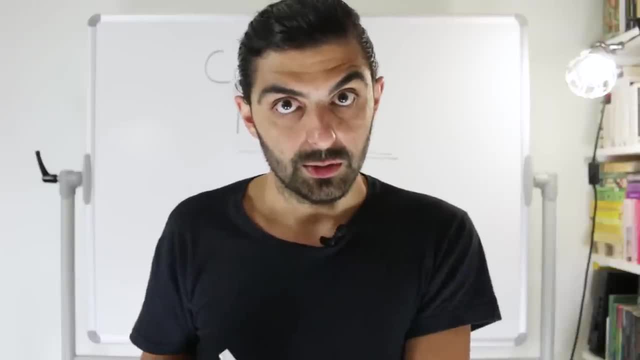 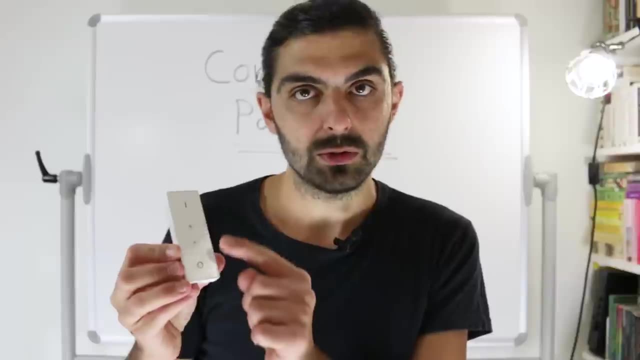 Or I should start to say invoker, because this is the terminology that they're using in the book. So this is the invoker. it invokes commands, right? So this invoker. we can't hardcode commands onto these particular buttons, because we want users to be able to design that themselves. 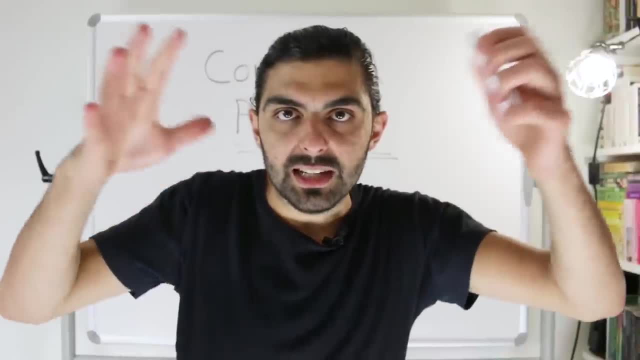 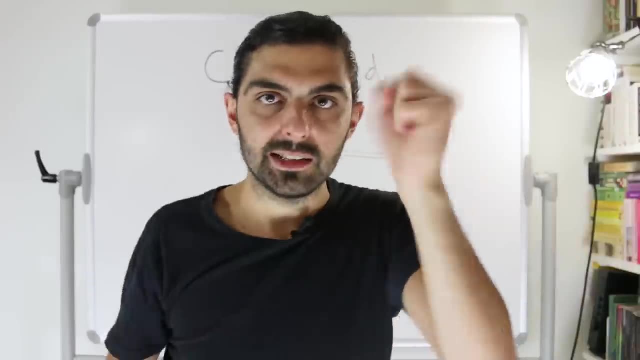 So this is why we want to have the notion of a command, We want to have a set of commands. right, Let's say, a command is light on and then you can attach a light to to an instance of that. turn light on command and then 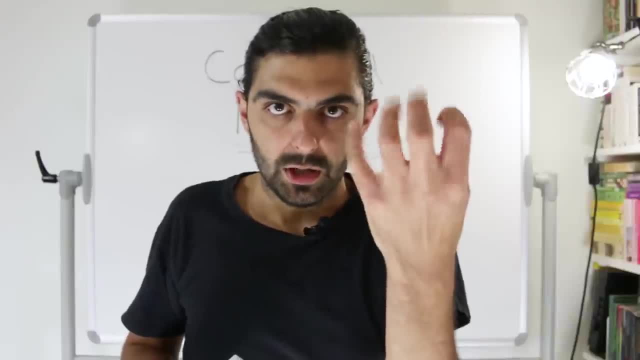 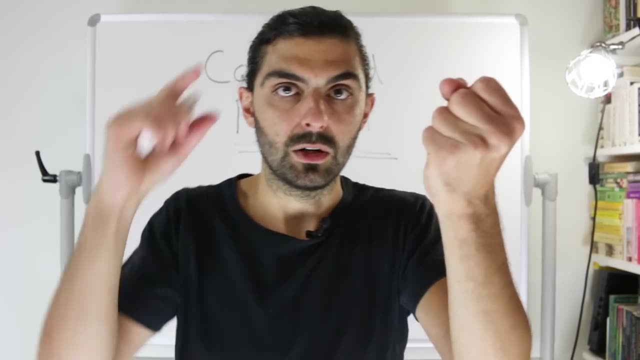 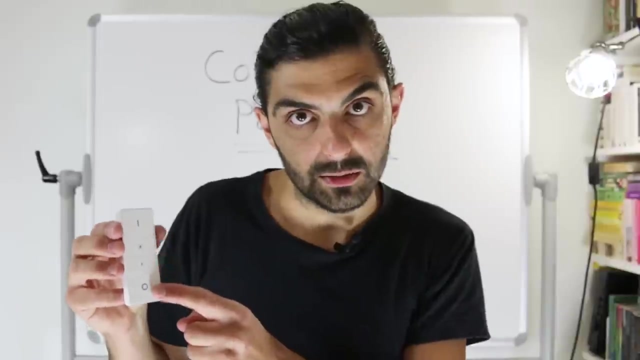 you put that command on this particular location. maybe another command is: turn room on right, turn all lights in room on, and then that to that command you pass a room id and then you attach that command to a particular button, so on and so forth for these other buttons. so this would be. 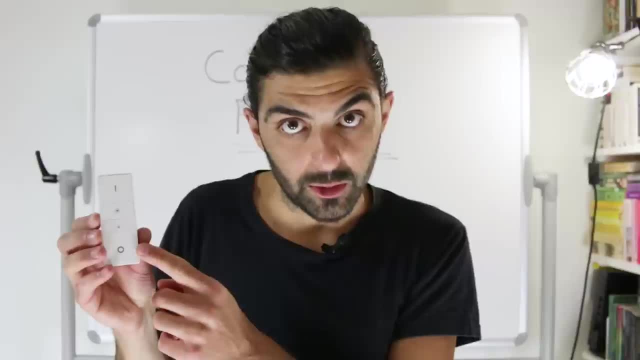 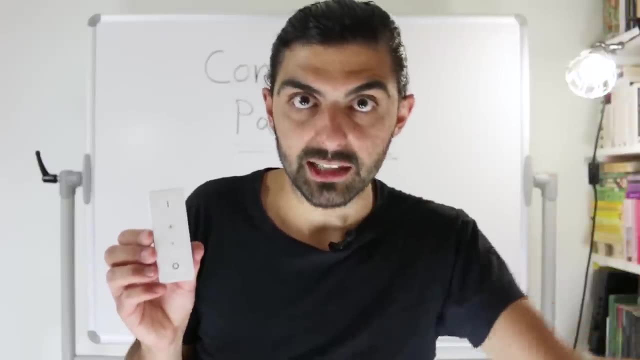 a dim up command, for example, and this would be like a turn off command, where this turn off command is either maybe a turn off all lights in room command, or turn off collection of lights or turn off light, for example. right, we're just thinking about a bunch of different applications potentially. 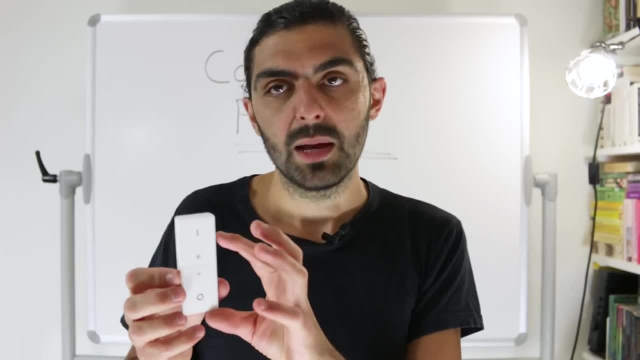 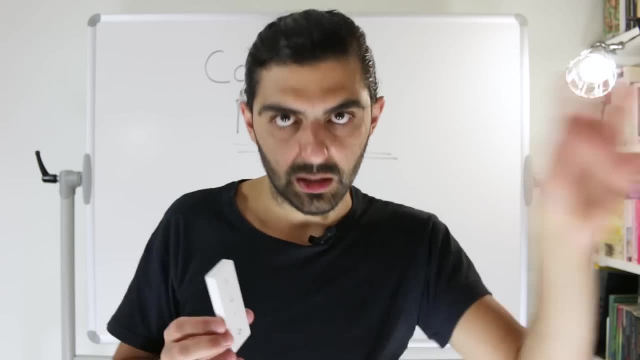 i mean you have to try to think a bit outside the box, like maybe my. maybe my example is too simple, because, since all of this is focused on lights, maybe you would have a single on command and a single off command, where the single on command would take an array of lights, for example, where 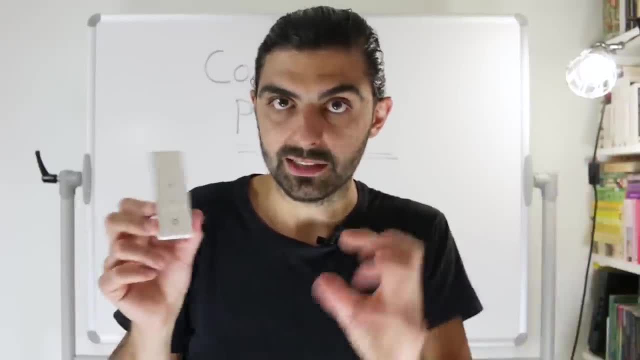 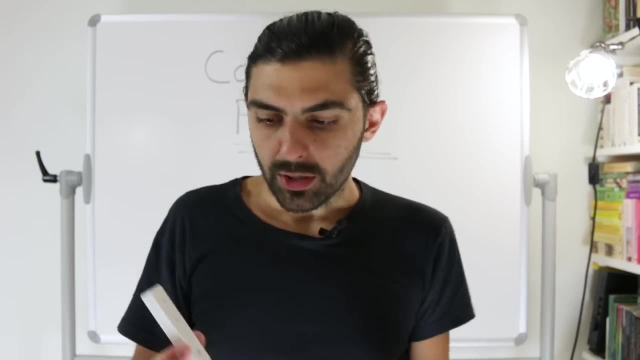 if that array only contains a single light, you would have a single on command and a single off command, where the single on command would take, well then it's a single light turn on, a single light command. and if it contains multiple lights, well then it's a multiple light command. that would kind of make sense architecturally. but if you think, 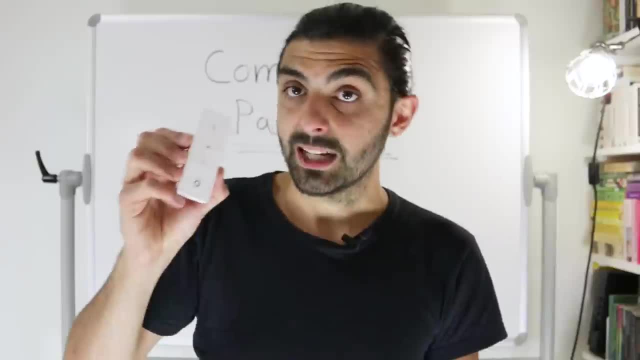 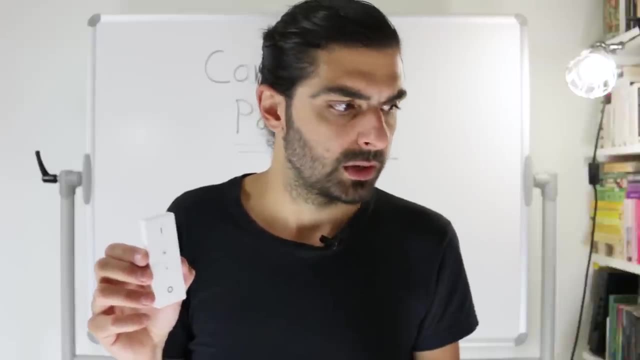 about it if this controller is not only a philips hue controller but like a universal controller, a smart home controller where i can attach lights from different manufacturers- i think there's another brand called lifex or lifx or something like that- so you would be able to connect those lights onto. 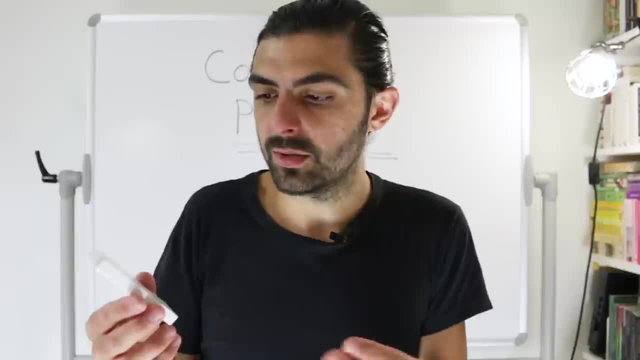 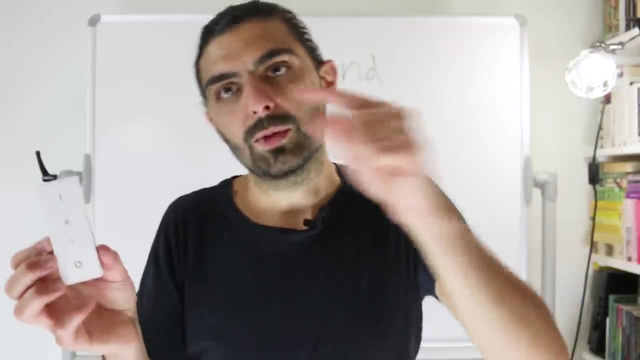 this controller as well, or maybe you have a nest thermostat or like there may be some some it's called wemo, the on and off switches. anyways, like you, you have a bunch of other smart things in your home and you want to be able to control those with the same controller. and if you think about it that way, you 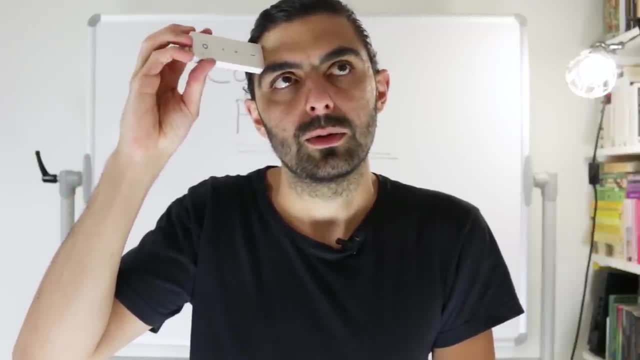 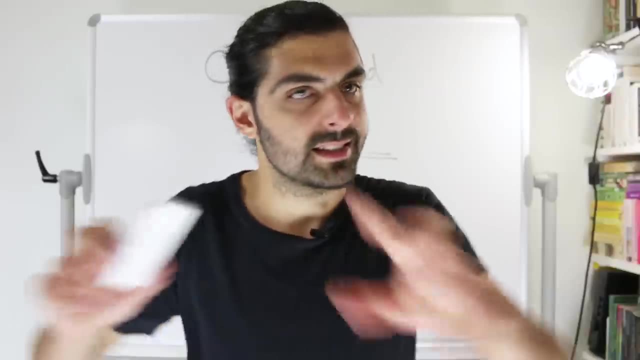 can see that, ah, like, the same architecture can actually be used. regardless of which thing i'm plugging in right, because the the one, let's think about it. the one thing that's that's the same across all of the things that we're talking about is that we want to press a button, want to send a. 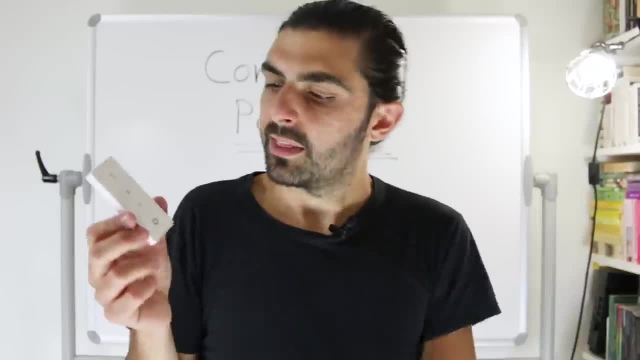 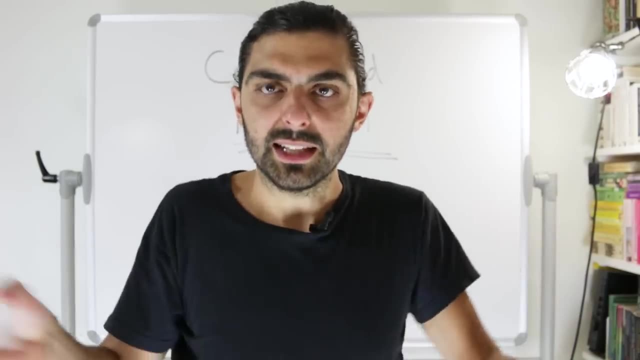 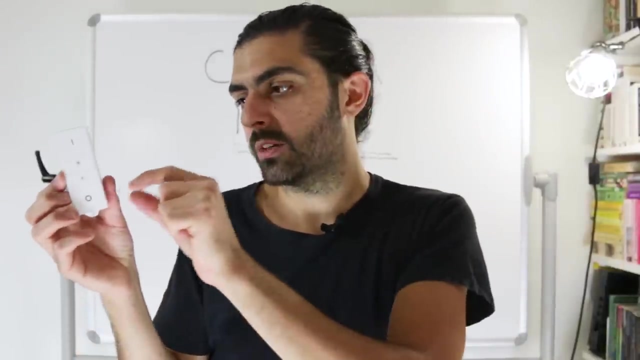 command to a particular device that does a particular thing. and this, this whole notion about attaching the command to the button and then sending the the command whenever we press the button. that that's completely the same thing across the board. we construct the command, we inject that command into the invoker and whenever the invoker is pressed, then we send that command. 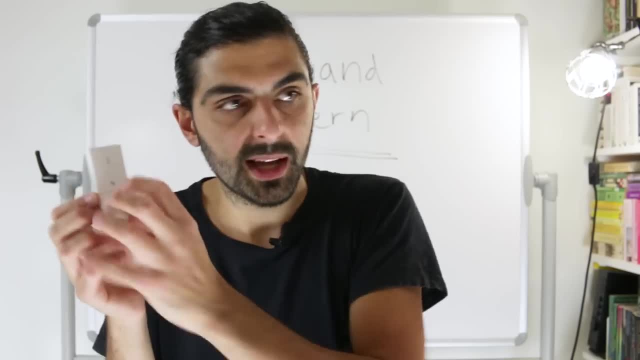 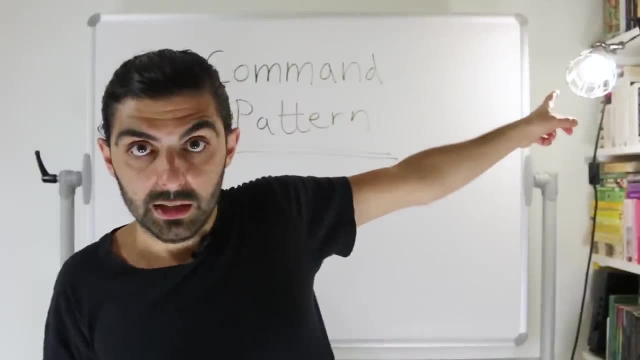 off or we execute- sorry, we execute that command and that command might do something to something else, and in the book they call this, this, something else. they call it a receiver. so the light here that's a receiver. so, invoker, we attach the button to the button and then we send the command off. 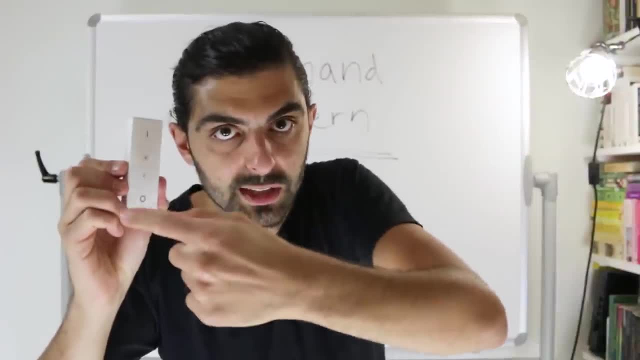 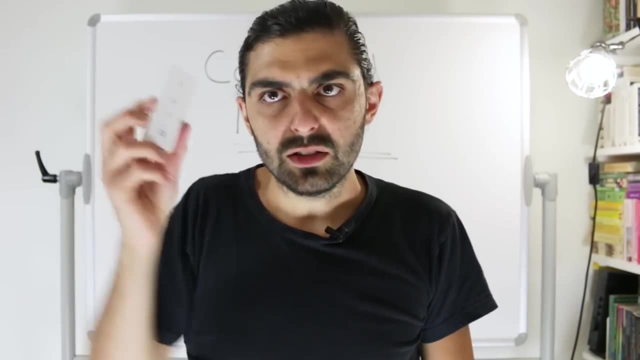 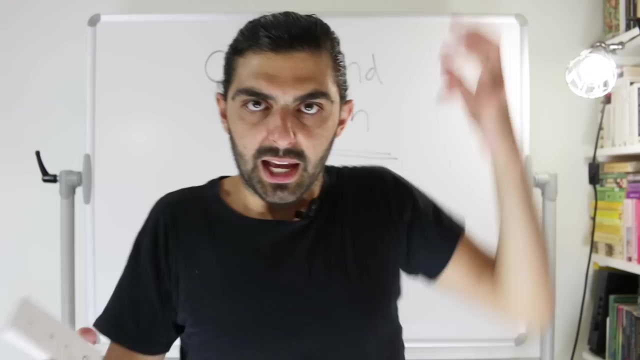 to the invoker and the command, when it's executed, actually does something to a receiver. probably you can realize how massively powerful this is. you can have tons of invokers that just couple to command. any command can do anything it wants to any particular receiver it wants, and if you're 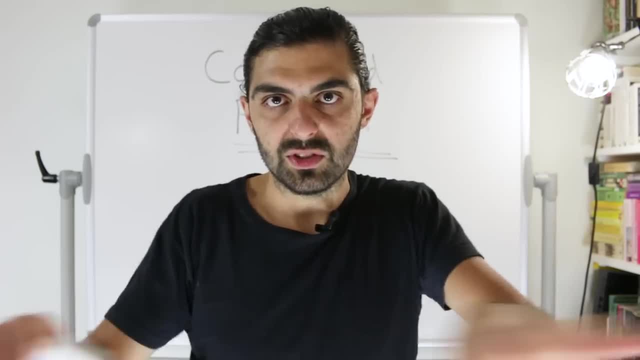 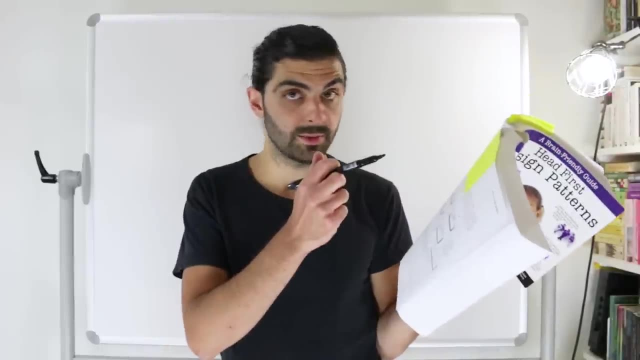 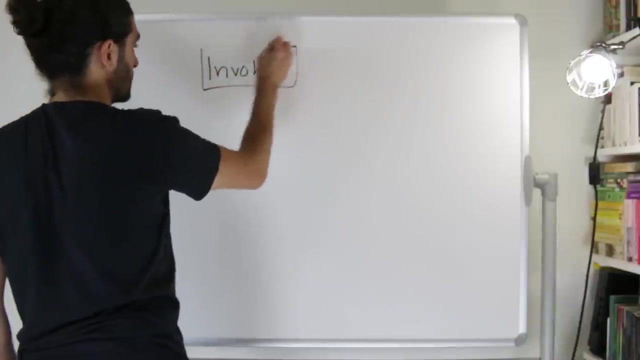 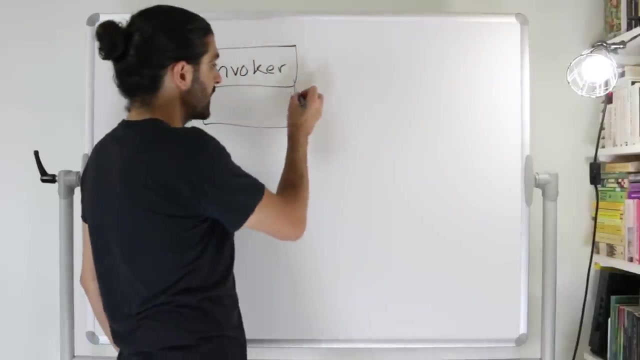 sharing interfaces with receivers. maybe you could even use the same receiver for multiple commands, but that's a different story. so let's now actually look at some uml. okay, so here's what we've got. we've got, as we were saying before, an invoker- this is, as discussed before, this thing, the, the remote control, and the invoker has 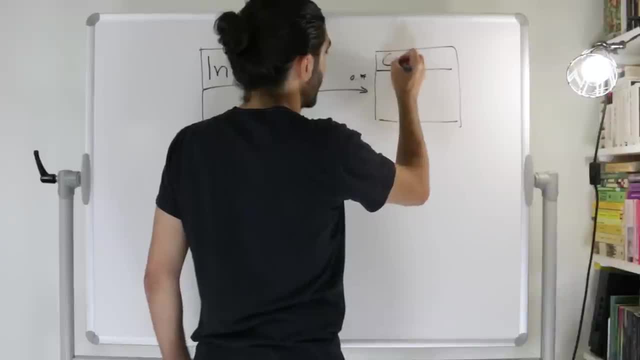 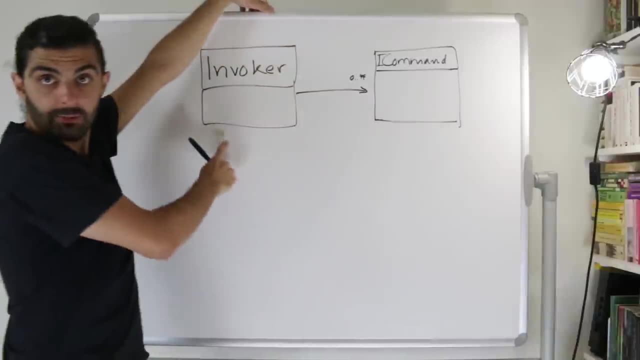 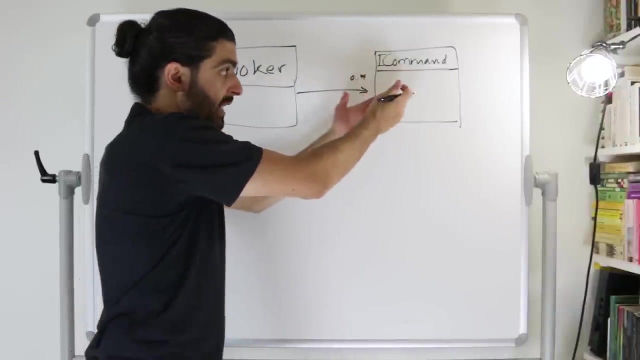 let me put zero to many command, and this is an interface, so let me put i here to say i command. so the invoker has zero to many commands but not concrete commands. it couples to the interface by command. the interface i command then of course has a number of implementations. 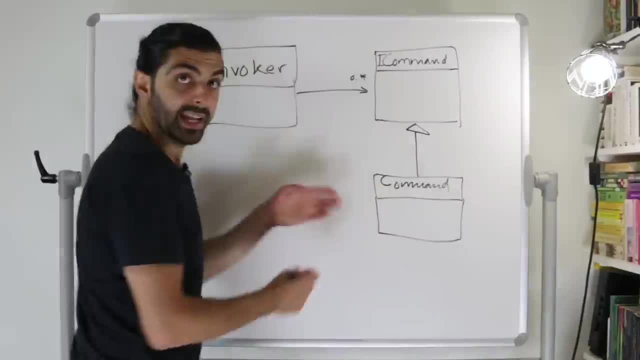 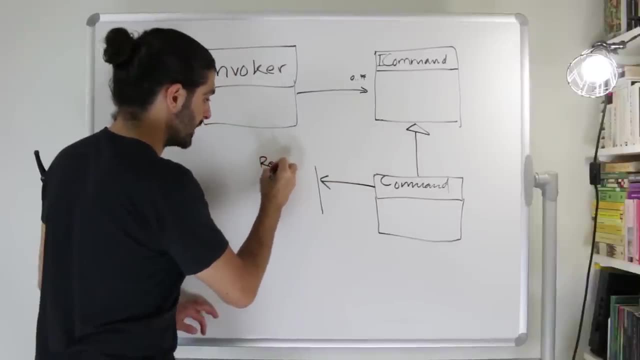 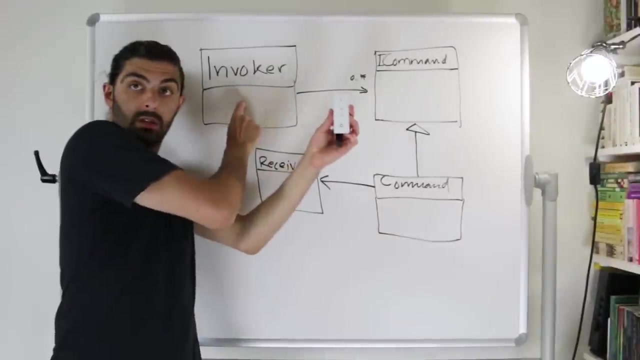 and these we call command, and any particular command acts upon ie has a receiver, re, and the receiver is the lamp. so the invoker, the control, the remote control, is loaded with its buttons, are loaded with command, with command and the receiver, so the receiver is the lamp. so the invoker, the control, the remote control, is loaded with its buttons, are loaded with command, and, as you can see, five controls and the only difference is the light. Mor54, EMP, свою excel, här�� uhs met viverие répond". 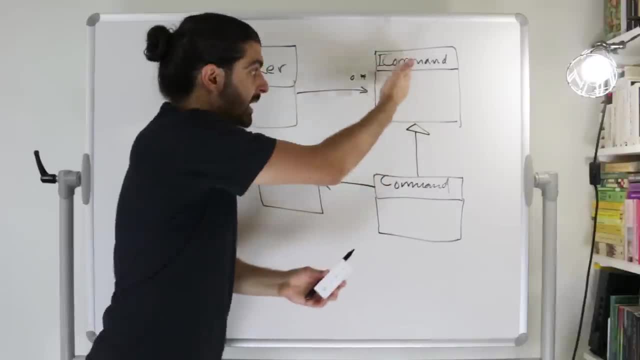 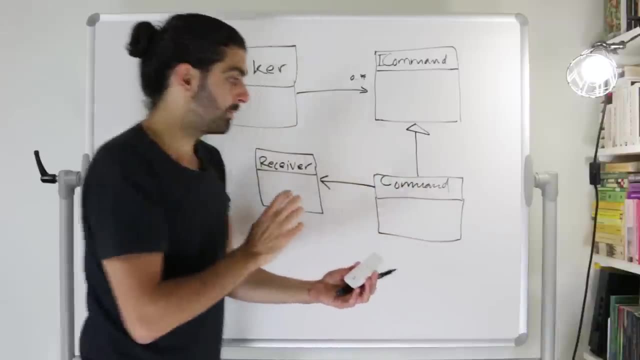 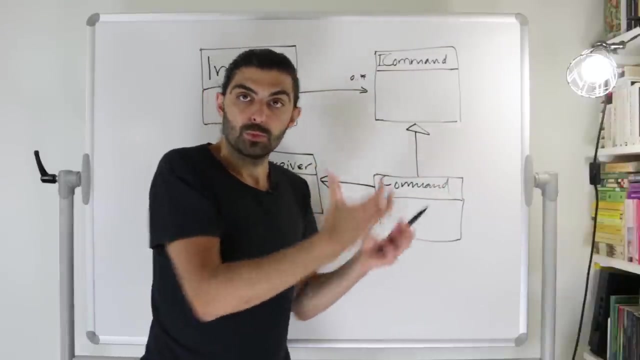 I commands. we define these as I commands and because the I command is an interface, it needs to be implemented by something and it's implemented by any particular concrete command and this command could be like a turn on light command, or turn on all lights in room command, or set color of light command. 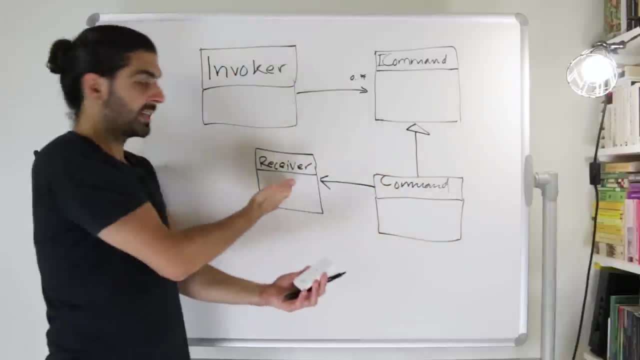 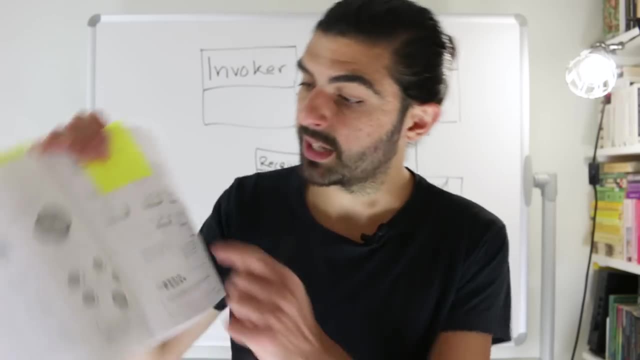 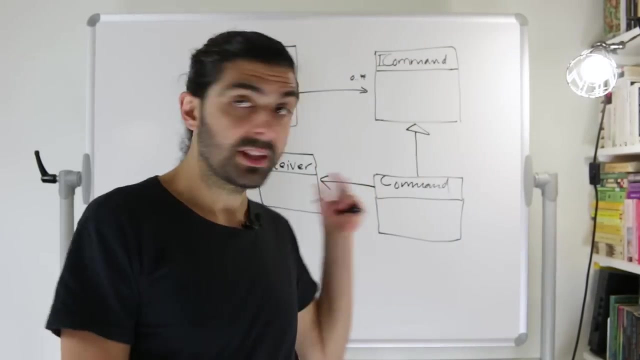 and that command acts upon some particular receiver. in this case, since we're talking about lights, a receiver would be something like this light. so in the headfirst book they've got another portion which is the, the client, which is essentially the thing using this pattern. but I think this is really the main. 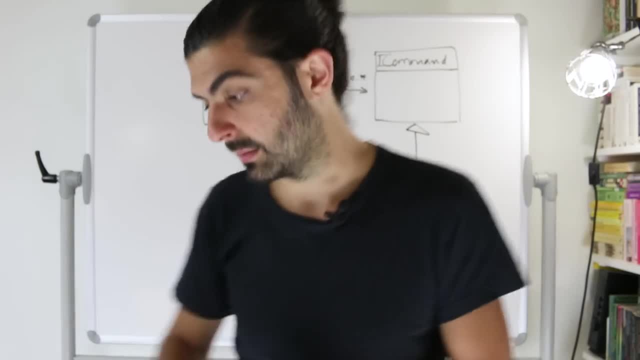 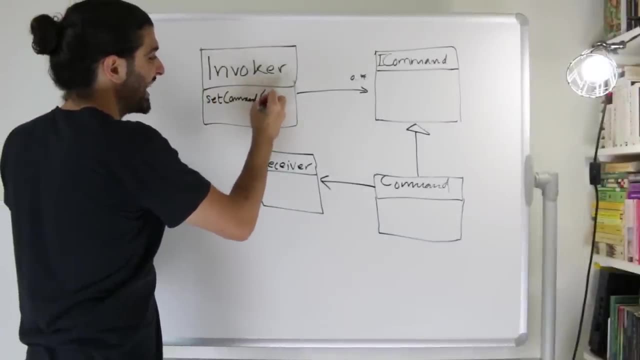 portion of the pattern, so let's stick to this portion and we'll talk about how to use it. so let's now add the methods as well. so the methods they add is that the invoker has a set command method that takes an I command serve for the lack of. 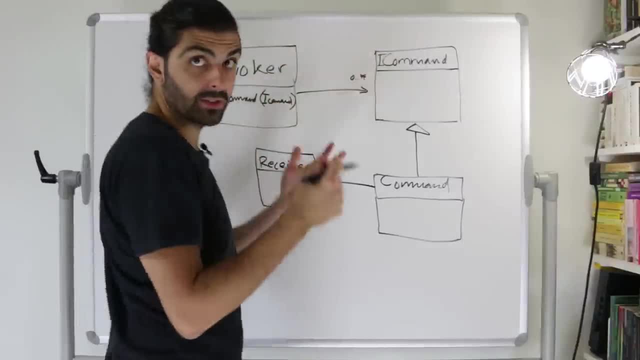 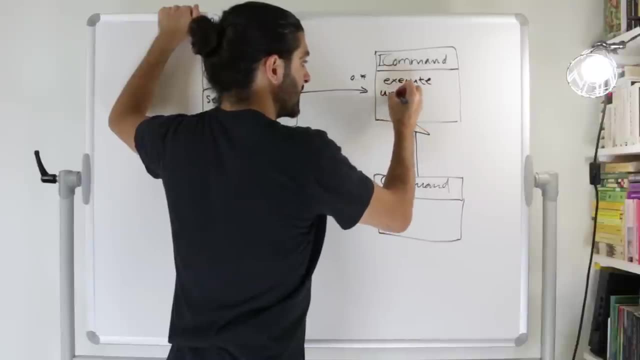 space, but the set command method takes an I command as an argument. the invoker has a set command method that takes an I command as an argument. the I command, the interface command, has two methods: one is execute and one is un-execute. so remember this is what we talked about, with the inverse, like 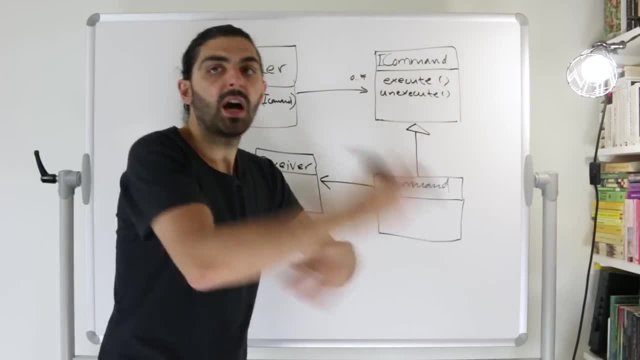 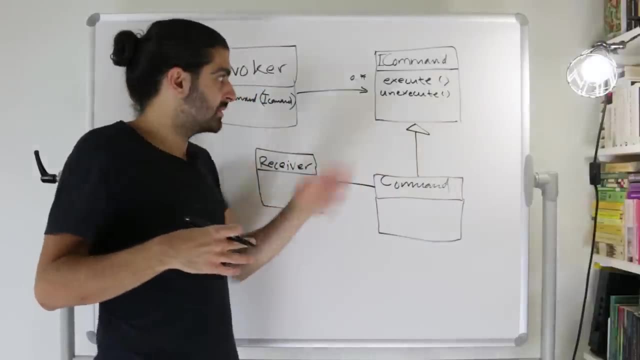 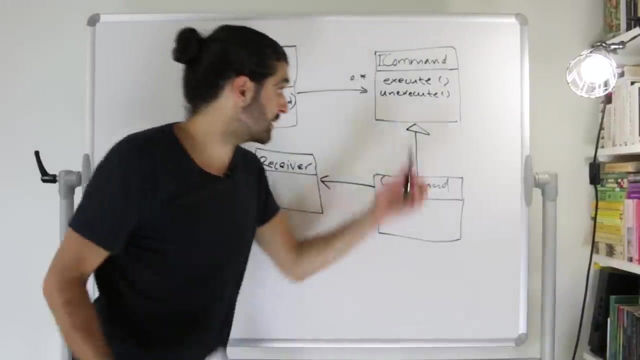 execute does the thing and un-execute undoes the thing right. execute performs some action and un-execute unrolls that action right. so it's like do and undo, and actually in the book they call it undo, but I just think it makes sense, kind of like as in this book, to actually talk about it as un-execute. 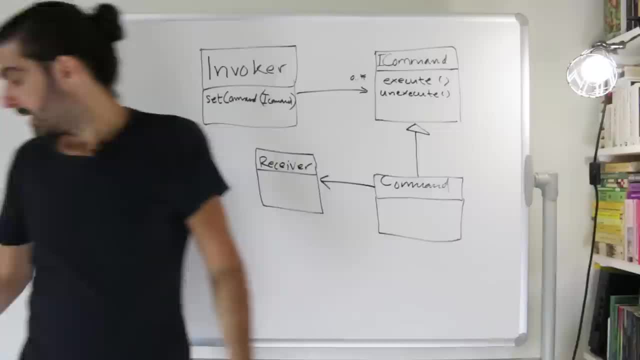 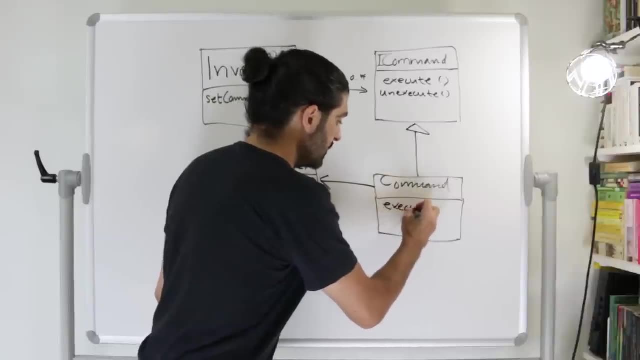 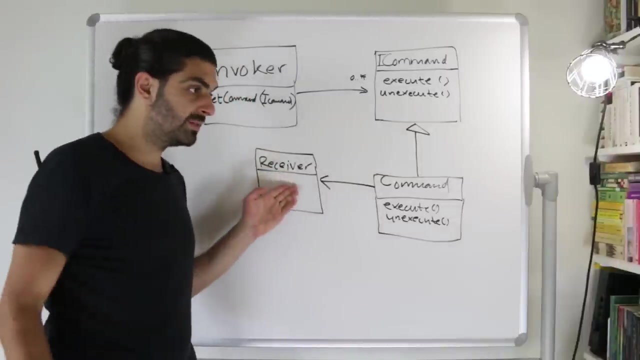 because it's the un-execution of the execution anyways. and then, of course, any concrete command needs to implement these two, so it needs to implement execute and un-execute. and the receiver we completely don't know, right, because the receiver could be absolutely anything. in our case it happens to be a. 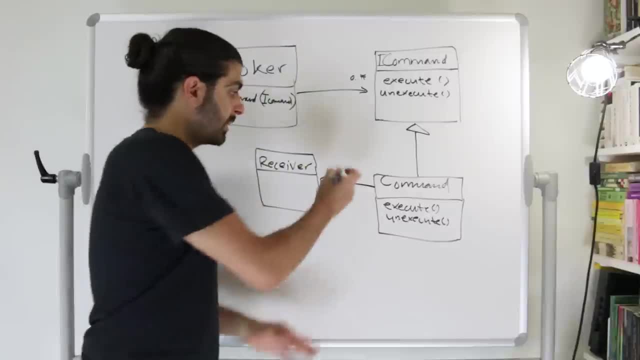 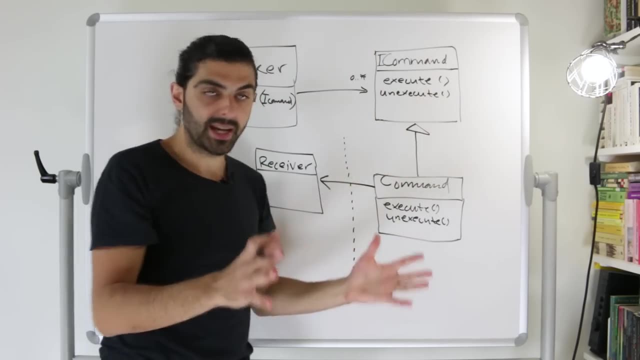 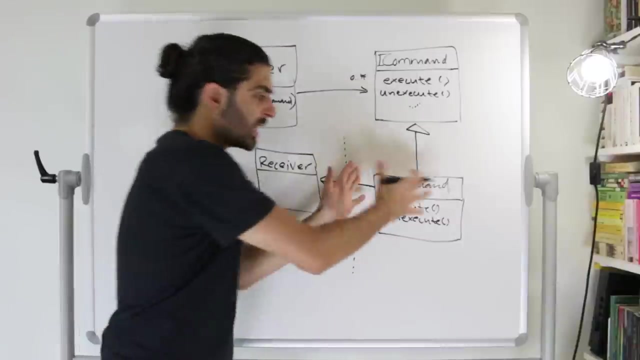 light. but there's no shared interface here, so you can think about it as like here is like an artificial boundary where this would be the same for every thing. like you have, you have a pattern, you have a system that makes use of the command pattern, so all commands follow this particular interface, but any 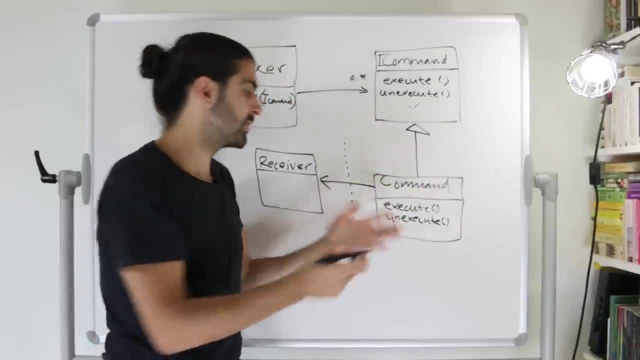 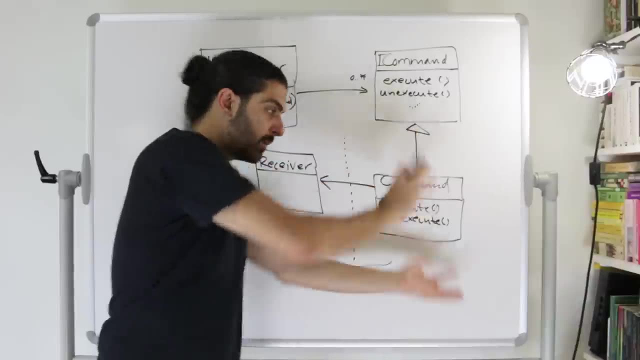 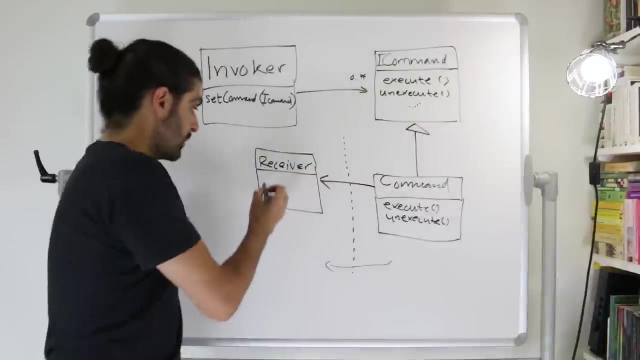 concrete command can have any particular concrete implementation, and that concrete implementation can sort of cross this boundary of of the generalizable- all all that stuff that's the same- into this very specific hard-coded land where you have any particular receivers such as this particular light. so in the book, 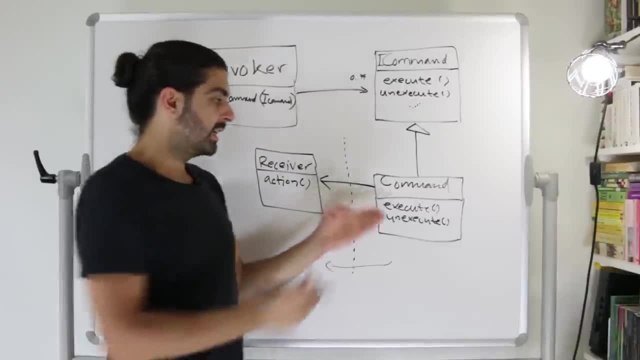 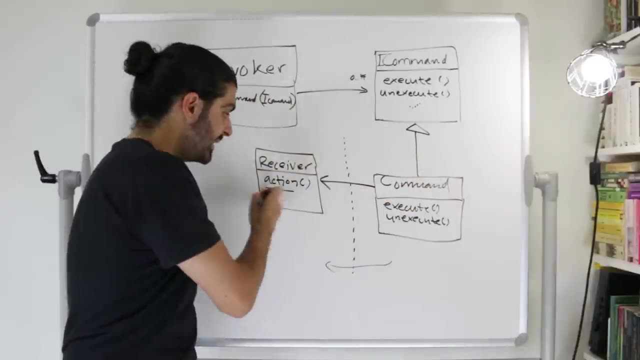 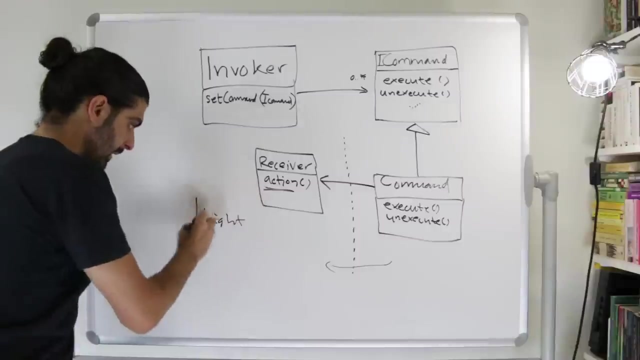 they just put action here, just to show that the execute method of the command would probably invoke a method which performs some action on the receiver. but this completely depends on your scenario. so maybe here we would have our receiver would be a light that has a on and off. 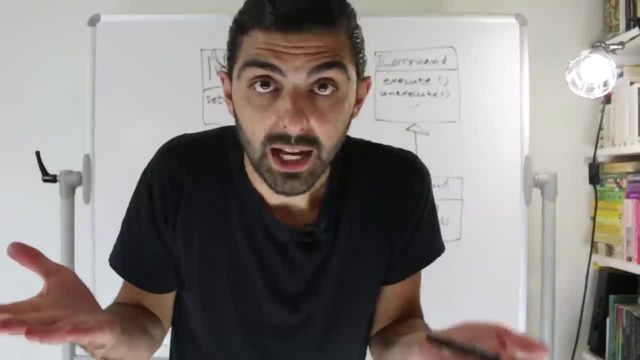 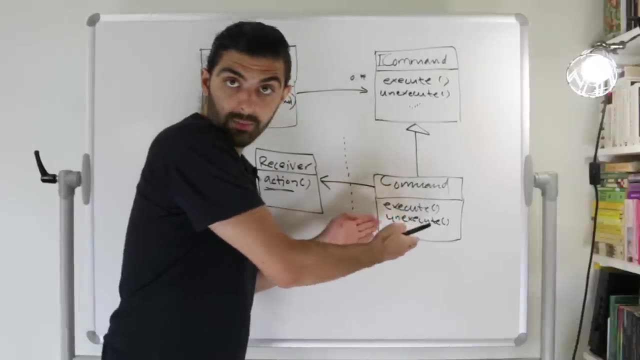 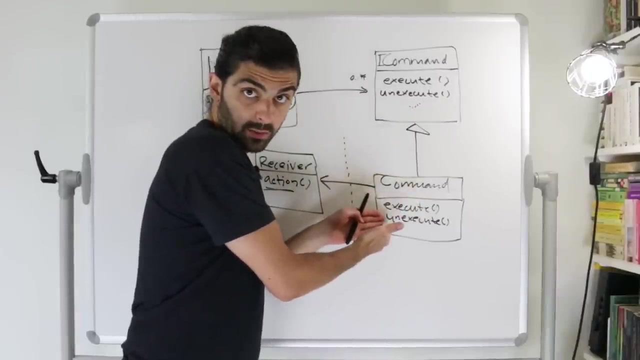 method, for example. and this is really it. this is the gist of the pattern. so let's walk through how this works. so you construct a bunch of concrete commands. let's say, Turn on light and the turn off light. These two have methods that are execute and un-execute. 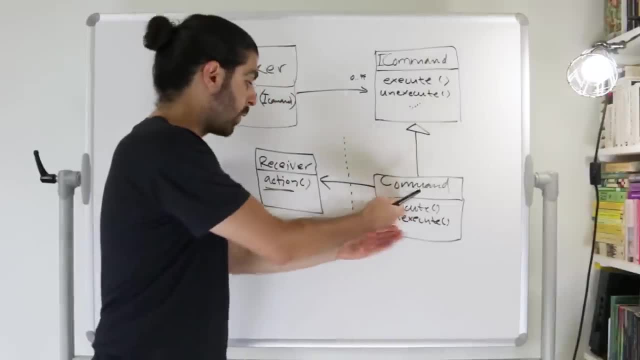 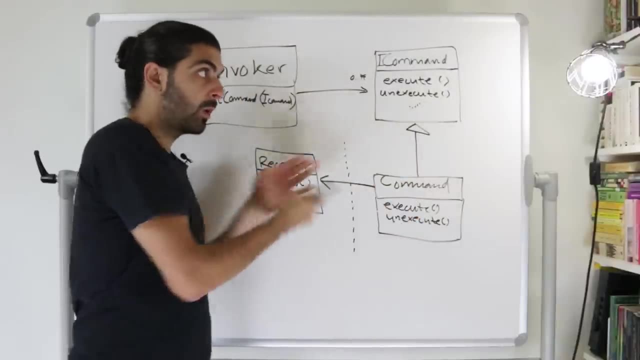 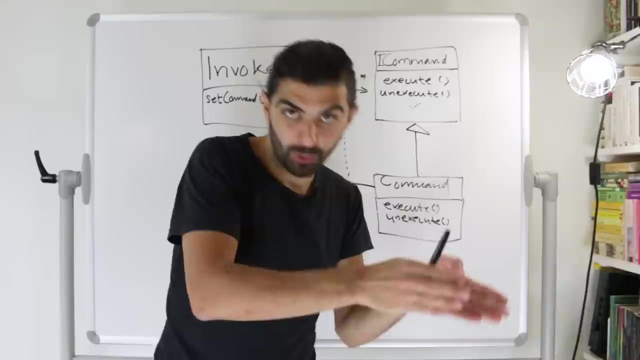 So execute of turn on light would probably be to call on on a particular light. Execute on the turn off light would probably be turn off on the particular light And un-execute of turn on would probably be turn off and un-execute of turn off would probably be turn on. So remember the direction of 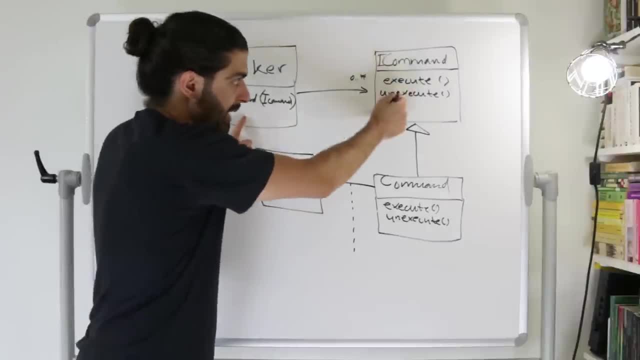 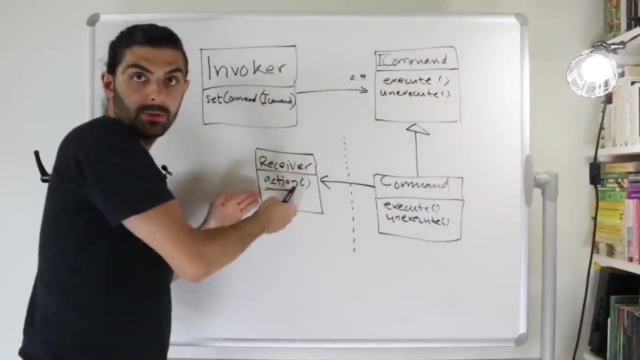 this arrow. We're saying that the invoker has many I commands. Any particular I command is a command and any particular command can act upon a receiver. So, by proxy, if you unroll the statement, this means that the invoker acts on. 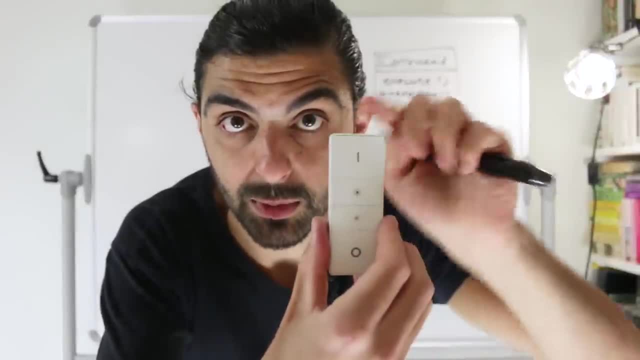 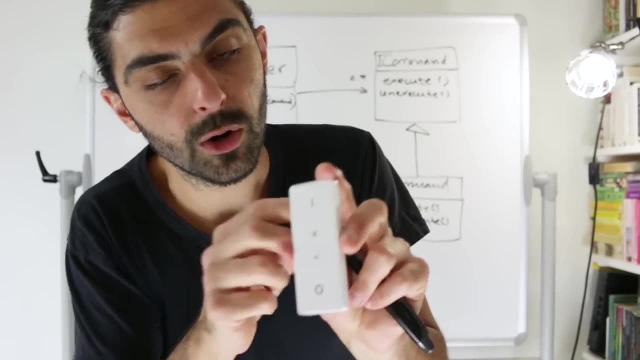 receivers. That's the end goal. We have this thing and we want this thing, to act upon these things. But because we want to do it in a general manner, we don't want to hard code, we don't want to say that when I press. 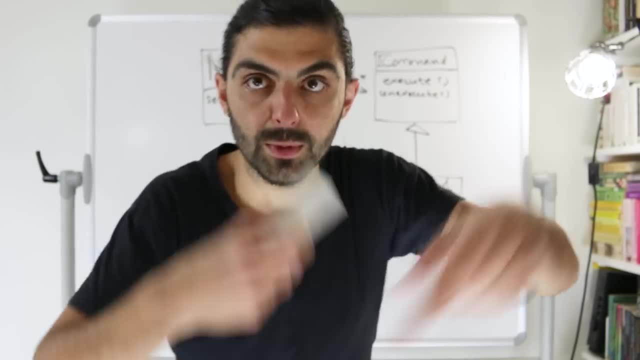 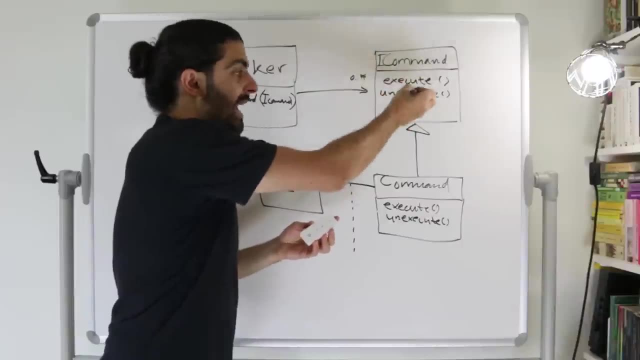 this button, the invoker will go in the other direction. So we have to get an this button, find this particular lamp and turn it on right. we want to do it by proxy. we want to say that this invoker is loaded with a bunch of different commands. we refer to them as i commands. 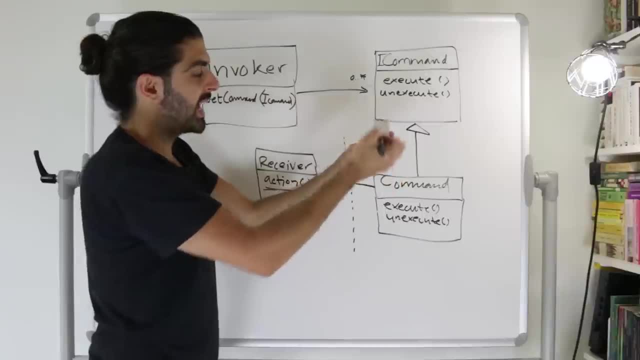 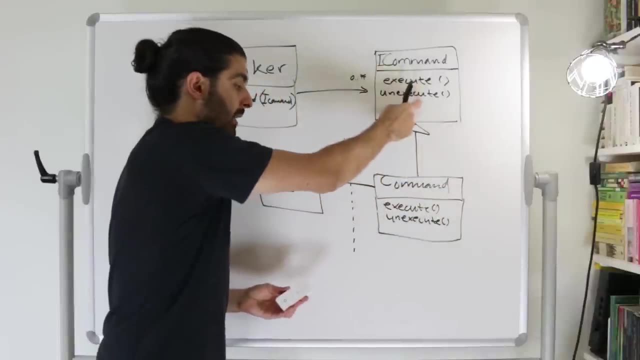 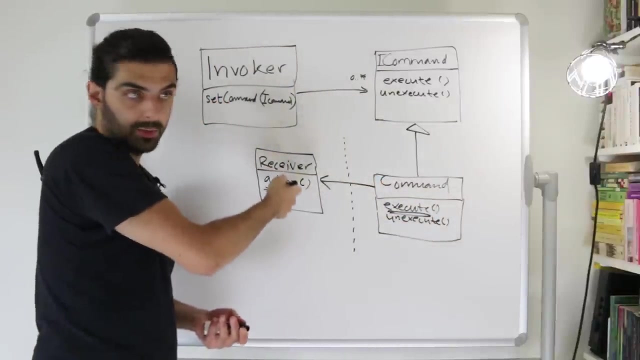 the type is i command. so we load any of these buttons with any particular concrete implementation of an i command and that concrete implementation is a command which follows the interface of i command and whenever that command is executed it performs some particular action on some particular receiver which is completely specific to that command. probably you can now also see how undo 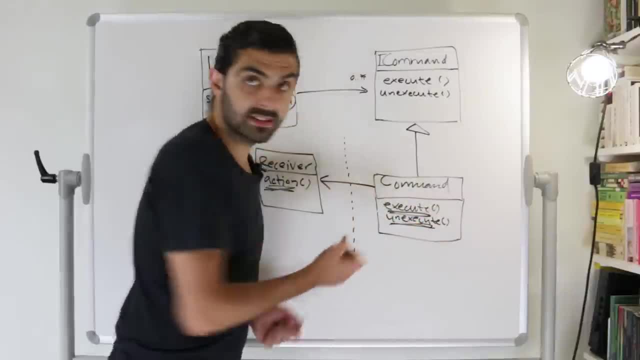 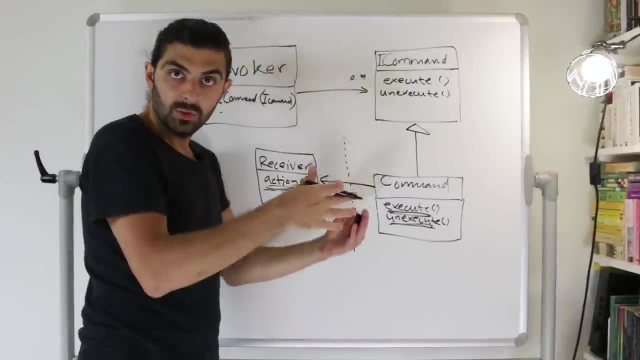 comes into play. so you have, if any command has an unexecute, that means that the invoker, if it keeps track of its commands, then it can actually unexecute a whole series of commands. so this kind of makes no sense in this particular use case. but let's say that we would load one of these buttons. 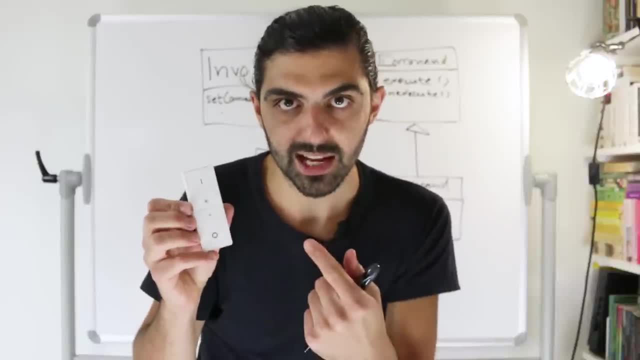 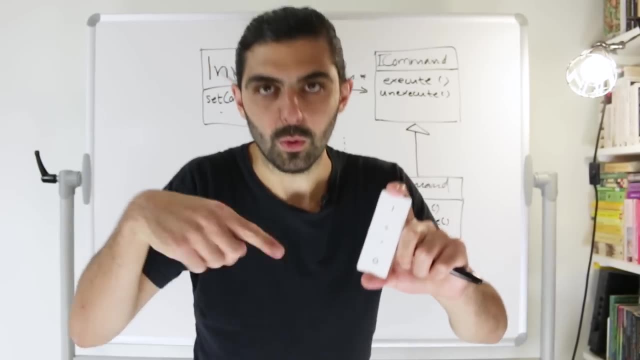 as a an undo button that unrolls every action. that means like, let's say, for 24 hours i keep track of every command that's run and when i press the undo button i sort of unroll all of those commands in sequence again, like that doesn't make any sense within this particular scenario. we'll talk about a scenario where it 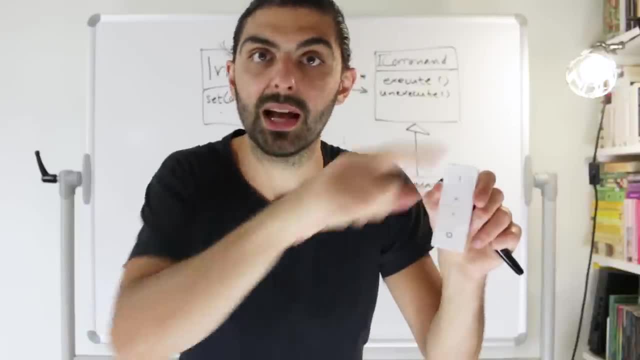 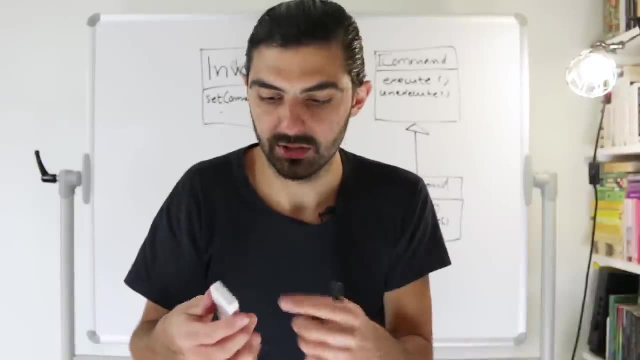 makes sense later on. but that would mean that i sort of play back a sequence of commands in the reverse order and with their inverse of their actions, so the opposite of their action. so if i had a turn on command it will act as a turn off command, because unexecute of on is to. 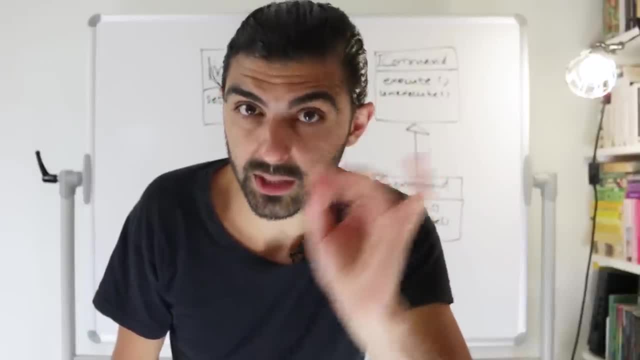 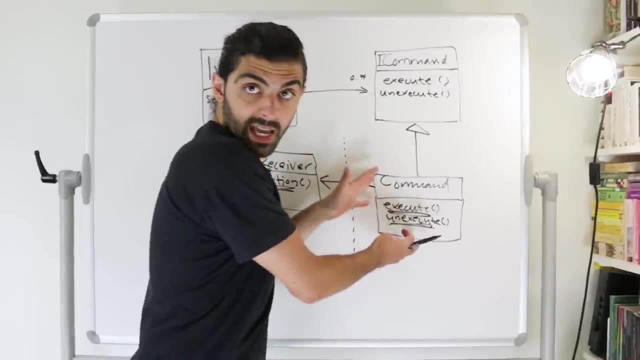 turn off. but before we talk more about undo, let's first, super shortly, look at some code. so i won't draw up the whole thing, but i want to draw two key portions, two key pieces. let's let's look at a particular command and its corresponding interface- i command- and let's look at the invoker. so what would the 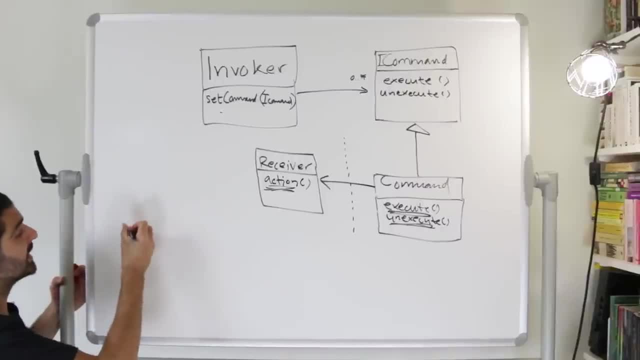 interface i command look like. so let's start in that end. so i command would be an interface called i command, and the only thing it specifies is that it says i have two methods, both return void because they perform actions. if you think about command query separation, they are commands, they are not queries, but that's a totally different discussion. they return void. 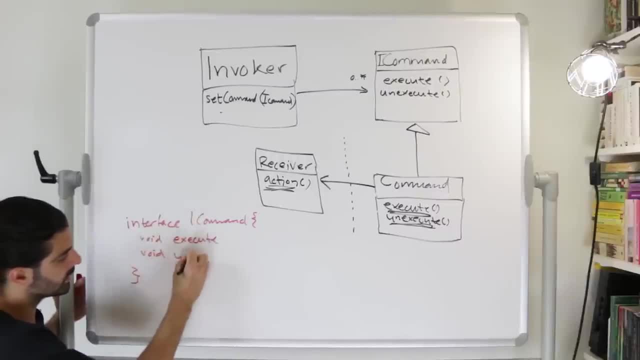 the first one is called execute and the second one is called unexecute, and they take no arguments. importantly, because the command has itself encapsulated all of the things it need to perform its duties. the command is going back to this idea that we talked about before is 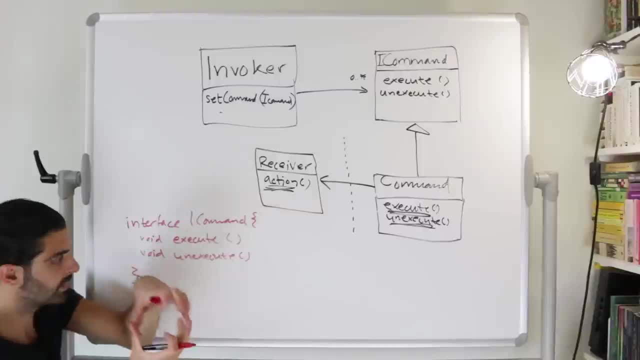 encapsulated. right, there's an action encapsulated in a command. the command doesn't require you to pass anything to it when it wants to be executed. you've already passed all of its dependencies to it upon instantiation. so the command- so the command already has access to the. 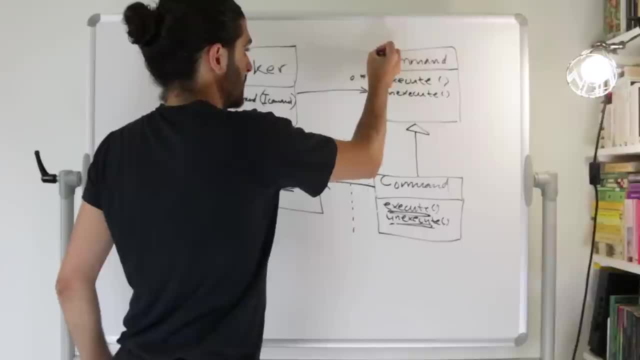 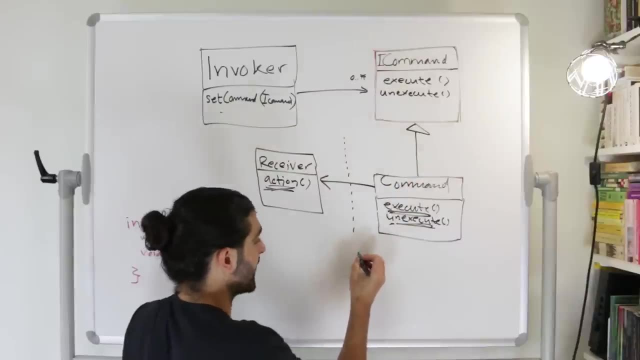 receiver that it needs to have access to, in this particular case the light. so that was i command. let's now look at any particular command. so let's say that we're building the command for this light. so then we would have a class called command that implements the interface. i command. 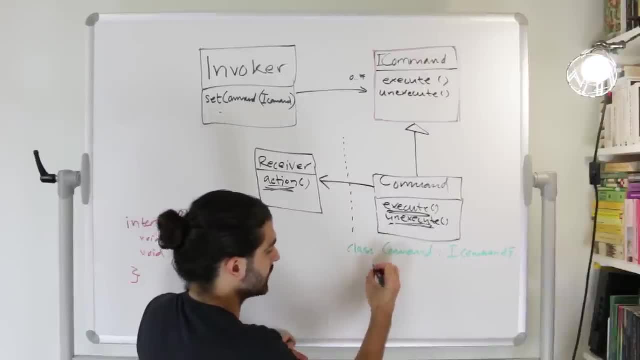 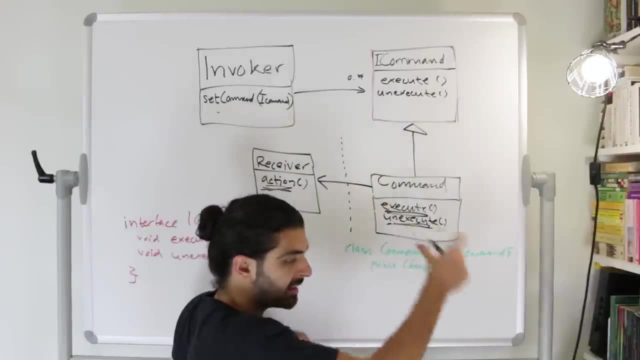 so i'm probably going to run short on space here, but what we need is that we need a constructor, so public command, and, as i was saying before, this command needs to immediately get to know about all the dependencies it needs to to perform its job. so this command needs access to the light immediately. so in the 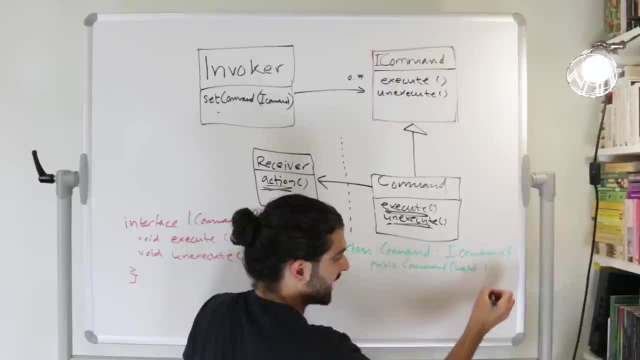 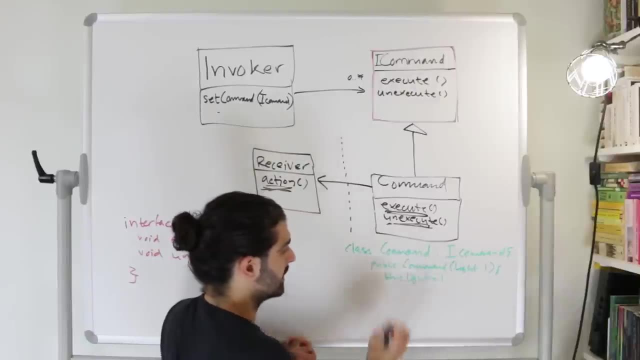 constructor. we pass a light to save space, let me just call it l. so we pass a light and then we store that internally. so we say this dot light equals the l that we passed in. and then here, okay, sorry about the space, we have a light. so there's an instance variable called light, so we save away. 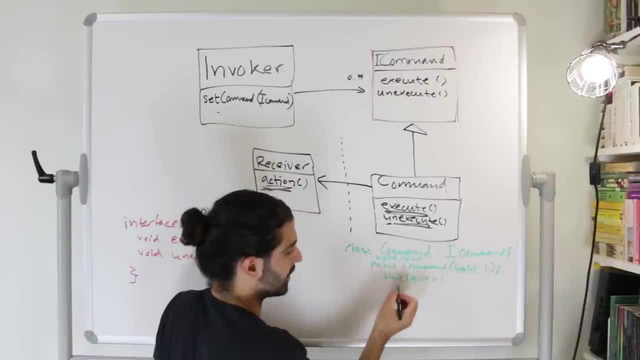 this light, that's passed in into the instance variable, which we do here. that's the constructor. then then what? then? we have a method called execute. so it's a public method. public void method called execute takes no arguments because it's following this particular interface and what it does is that. 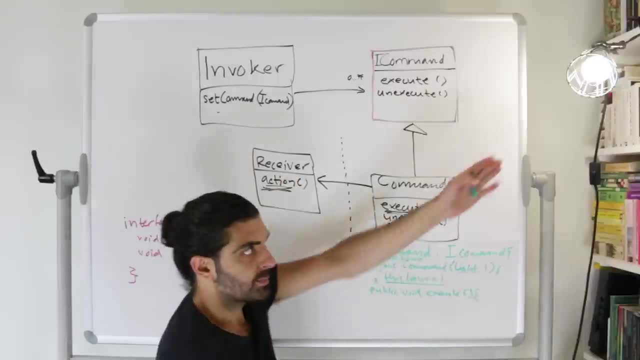 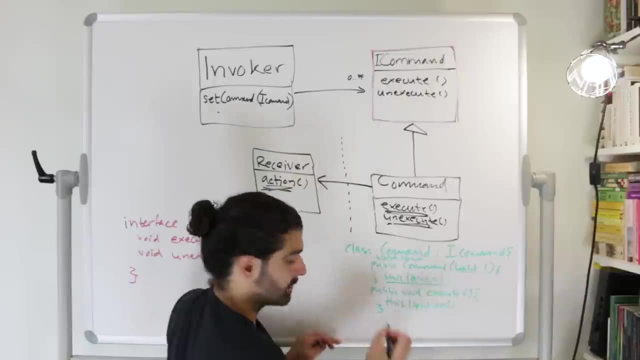 it acts upon the light, it acts upon its receiver, and let's pretend that this light, this receiver, has an on the method. so then we would say: this dot, light, dot on, simply that's it. it's not complex, that's not the point, it's not. it's. it's not that we're wrapping. 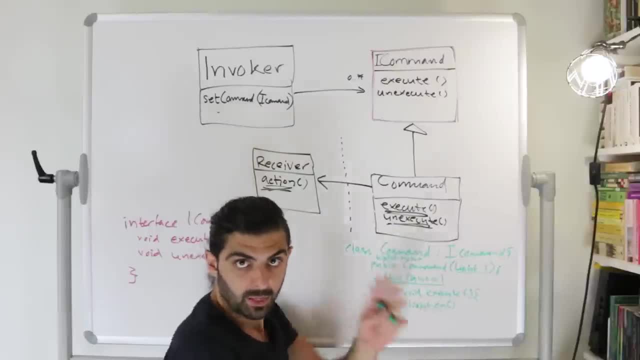 a complex action. it could be exactly this simple. the point is not that we're encapsulating something that's complex. the point is that we're encapsulating something that's potentially trivial so that we can pass it around. if you think about functional programming, functions are first-class. 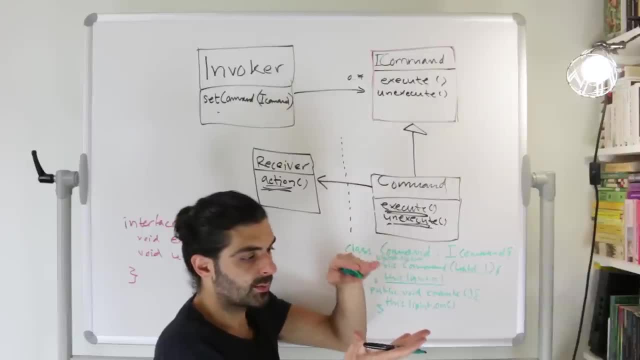 citizens. so it's trivial to take some procedure and wrap that in a function and then pass that function around. command pattern is a function. that is a function. that is a function that is a kind of gives us this flexibility in object-oriented programming. so we wrap some action that we want. 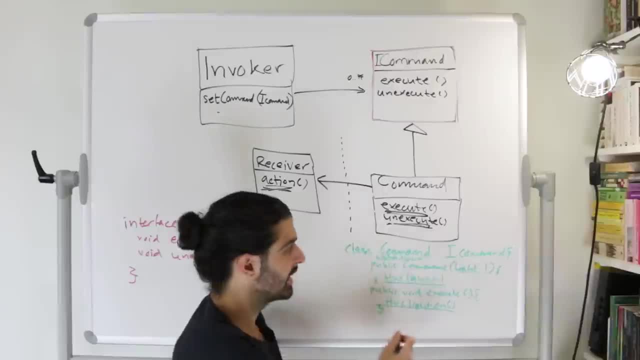 to be able to perform, which is actually just this: this dot, light dot on right, light, dot on. we have any particular instance of a light and we want to call on, so you wrap that into a class and then upon. if you instantiate that class, then you can suddenly pass around this object. you can suddenly 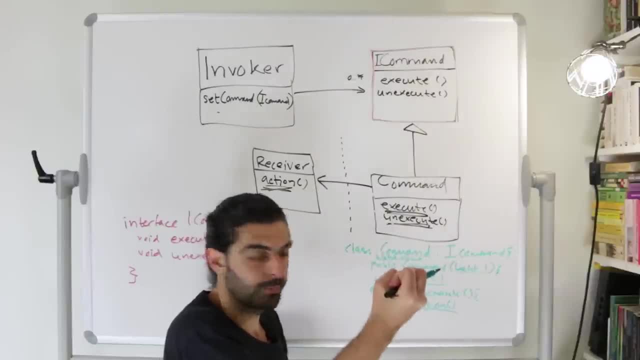 pass it around as if it was a function contained in a variable and that's the execute method. then we would have unexecute, which is essentially the inverse of this, so we would have public void unexecute and we would say the implementation would be that we would say this: 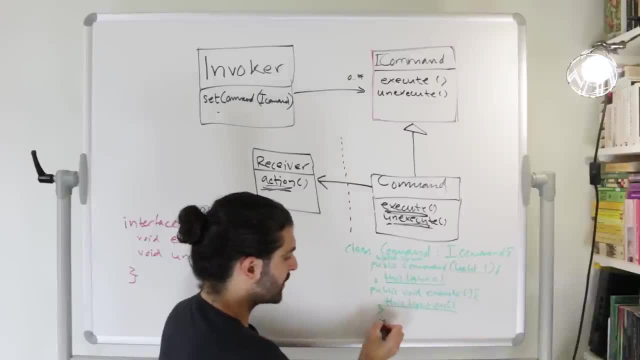 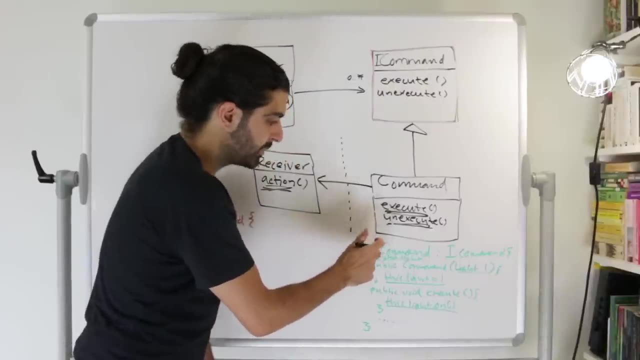 dot, light dot off, for example, for this particular command. but i'll just put dot dot dot here, because i think you can figure that out, and then we'll close the class and actually of course i call this command, but probably the name here should have been light on command, because then we would. 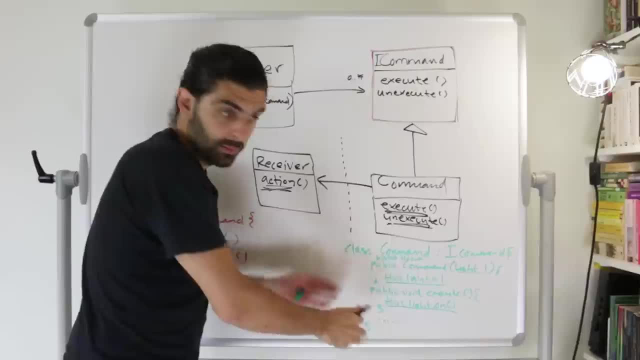 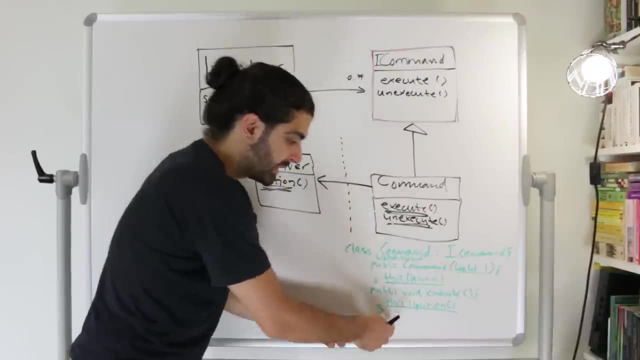 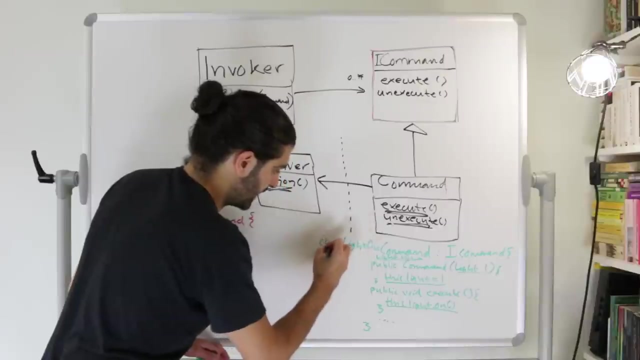 have another command which is light off command, which has the inverse of this, so the light off command. upon execute would say this dot light, dot off. and upon unexecute would say this dot, light, actually add the light here. so we'll say light on command and it's a class. sorry about the mess. 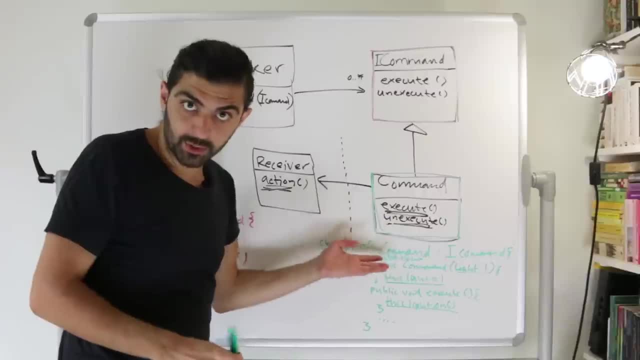 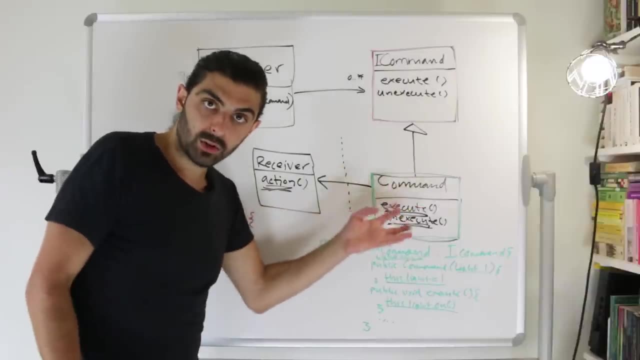 and that's that. so that's the concrete command and key point. we might have multiple concrete commands. we might also not have multiple concrete commands. again, we might do this even if we have a single concrete command, just so that we are able to sort of batch the execution of this command. and this is 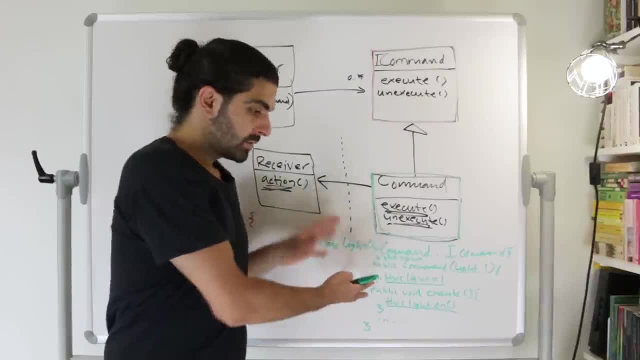 why in the book they were talking about queues. for example, like you might construct commands and put the commands in a queue so that you can execute the command in a queue, so that you can execute the command in a queue, so that you can execute the command in a queue, so that you can execute them. 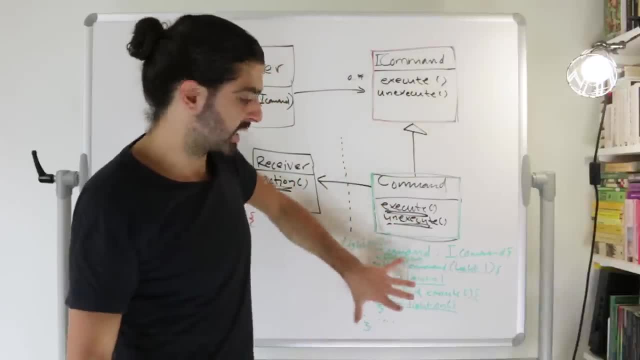 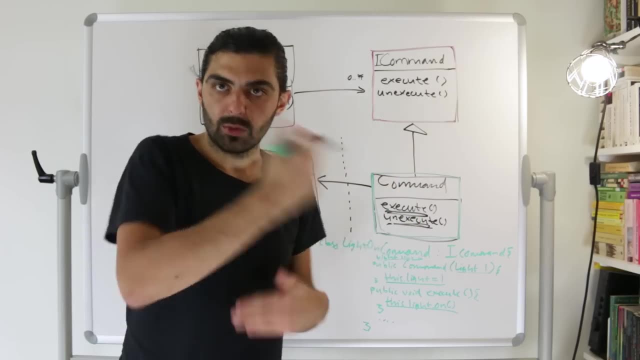 one by one or in batches, right, like, let's say, this was an expensive operation and you want to batch them. so you want to say: i have a series of commands and every 30 seconds i execute 10 of them. right, so like you would throttle, even if you are pushing more commands into the queue. you're sort of only. 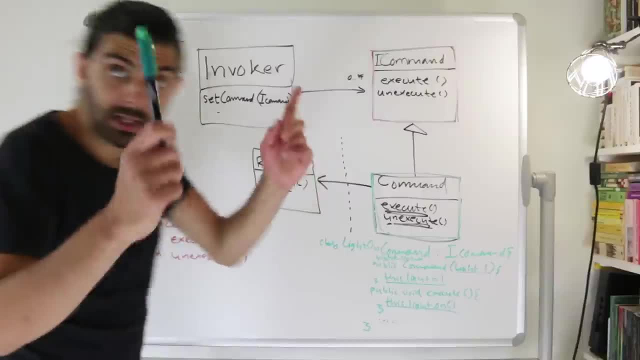 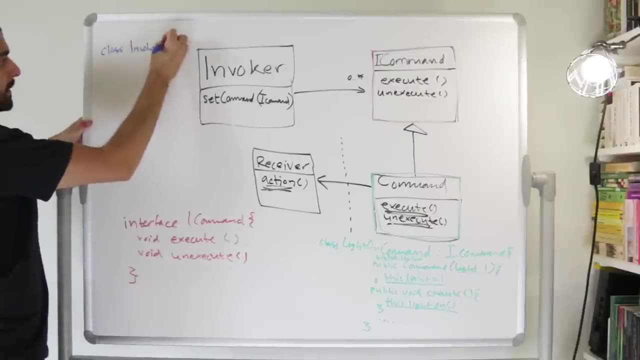 taking 10 at a time, every 30 seconds, or something like that. lastly, let's look at the invoker. so what would the invoker look like? so the invoker is a class and what it does is that it somehow keeps track of commands. remember now that this is not necessarily a part of the of the pattern, actually. 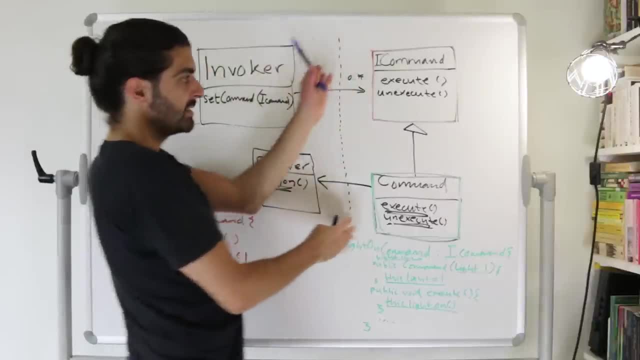 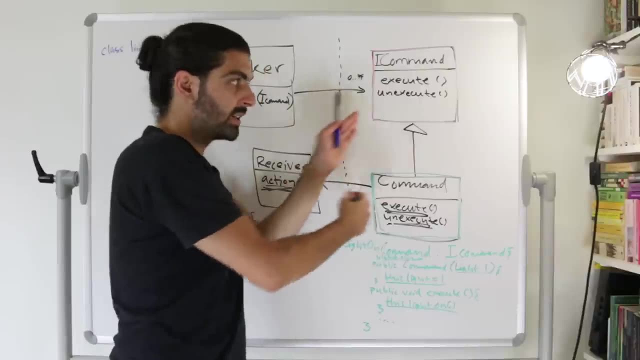 we could probably extend this line and say that this stuff, this is really the key portion of this pattern which might look a lot like strategy pattern, which might make you wonder, well, what's actually the difference between this and strategy pattern? and i would guess that probably the only 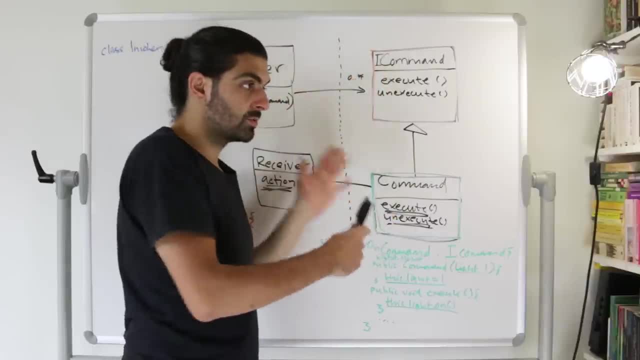 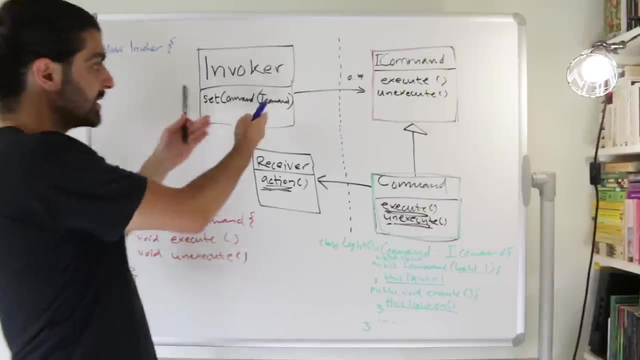 difference is really the intent. like here, we're treating the strategies as commands, but if you have more questions about that, please raise that as a question and then we'll dig into that some other time. so, in other words, the invoker, just like the receiver, is specific to the scenario in which 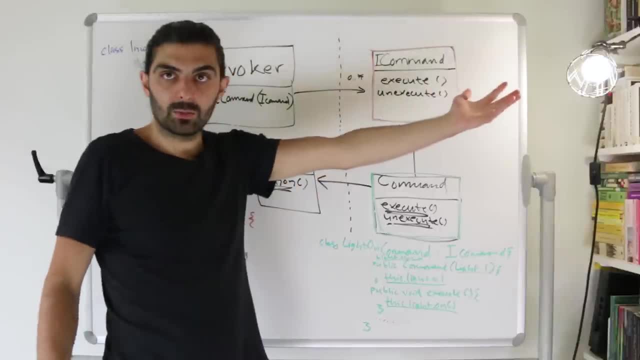 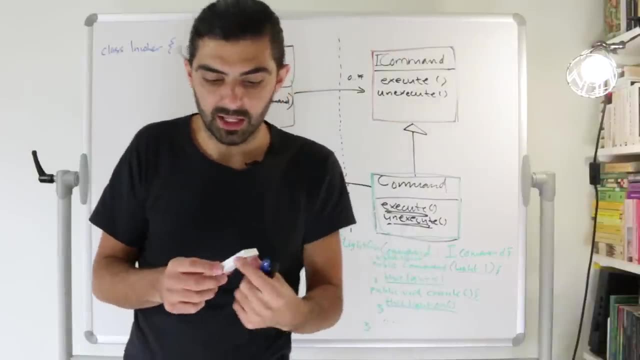 you're operating. it's specific to your context. here we have lights that were receivers right and invoker for us was this thing, but the invoker in your scenario could be any particular thing. so actually, even in your scenario, you might have multiple invokers that have multiple different. 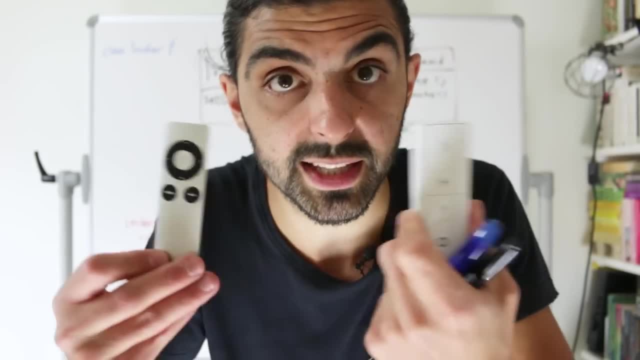 interfaces. so like you'd have this invoker and you'd have this invoker, and then they have completely different interfaces and, in regards to this pattern, they don't necessarily need to share an answer. so you could have this invoker and you'd have this invoker, and then they have. 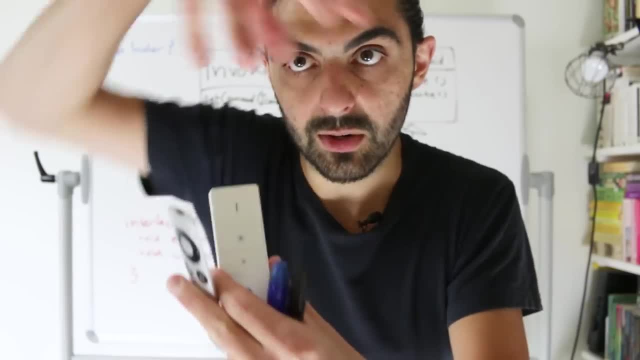 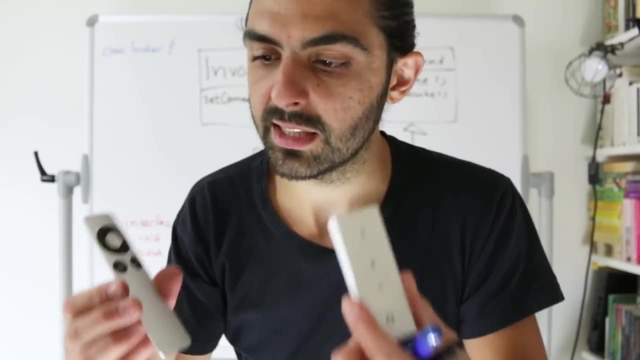 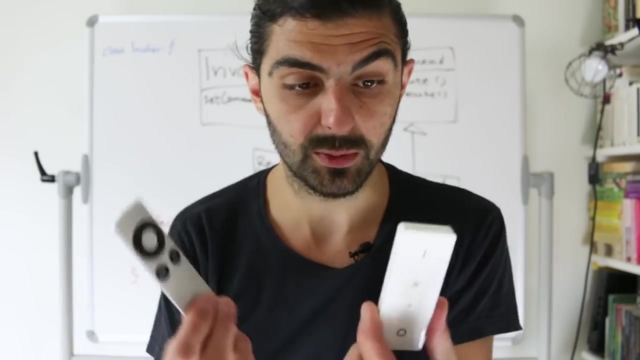 a common ancestor. these can be concrete classes that don't share a common ancestor. they can be different classes with different interfaces because, in regards to command pattern, the only thing that they need to do is that they need to support the adding of i commands. of course, depending on your scenario, it might make sense to share a common ancestor between these so that you 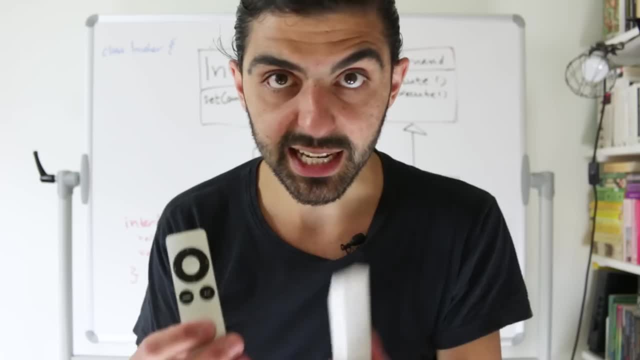 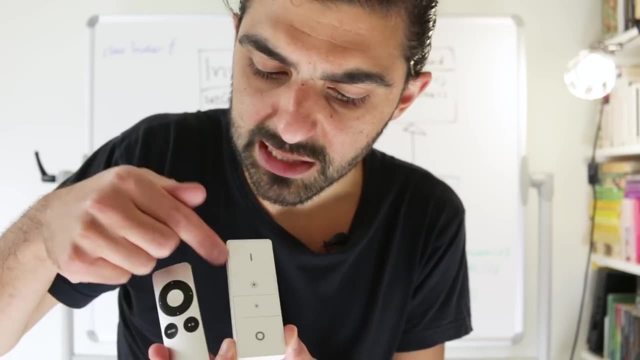 could share these so you could treat them the same way. but again, that that completely depends on your scenario, if you just think about it. i mean, this control has four buttons and actually, like semantically, you can't share a common ancestor between these. so you can't share a common ancestor. 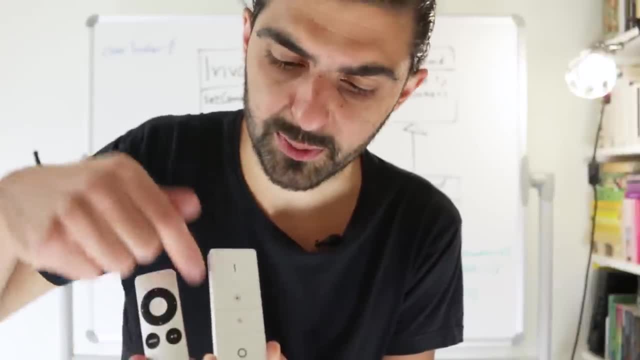 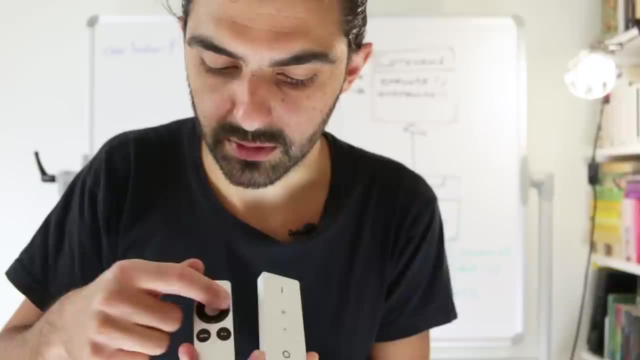 between these, so you can't share a common ancestor, between these, so you can't share a common ancestor. it's like these buttons have some kind of meaning. so, like from the user's perspective, you'd expect that these different buttons behave in sort of different ways, and this control has one, two, three. 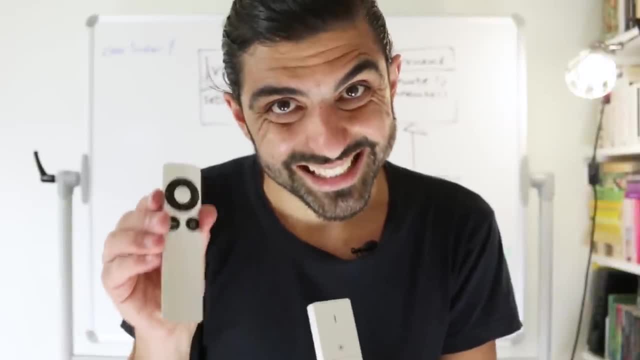 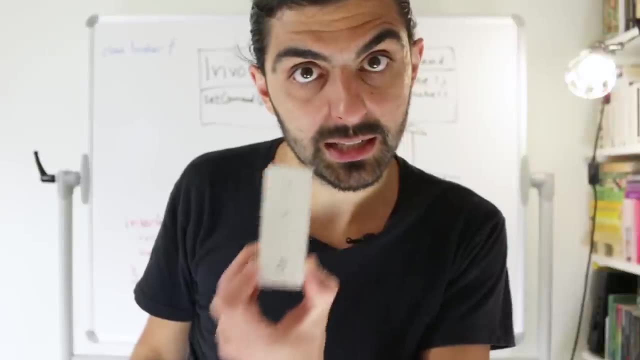 four, five, six, seven buttons. so this one necessarily needs seven commands to function properly, unless we're sort of loading one with a no command command. this one necessarily needs four commands to operate sensibly, again, unless we load one of the buttons with a no command command. and and this: 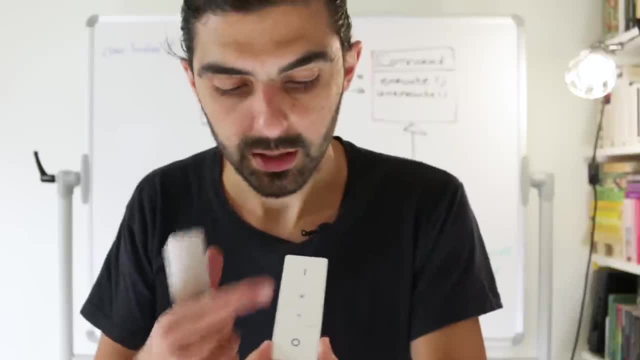 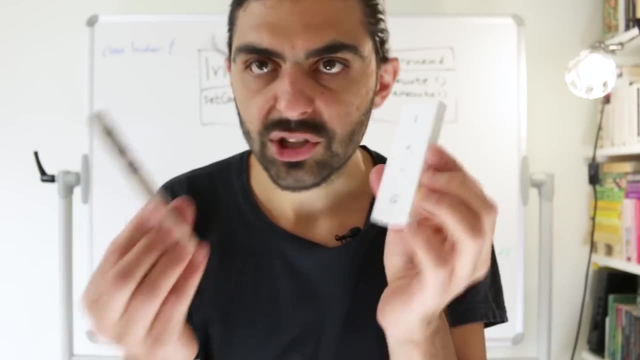 particular control. if you would try to load it with a no command command, it would be a no command command with more than four commands. that wouldn't really make any sense. similarly for this one if you go beyond what it supports, so like they're actually completely different things that we want to. 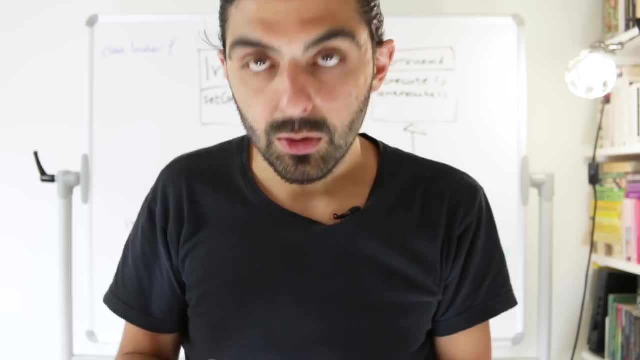 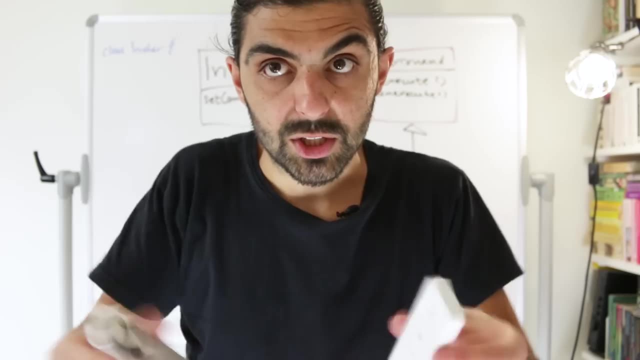 interact with in completely different ways, but the key point is that the notion of a command we make the same, so we load these things with commands and then the commands can be shared across these different invokers, even though the invokers have completely different interfaces. hopefully now you 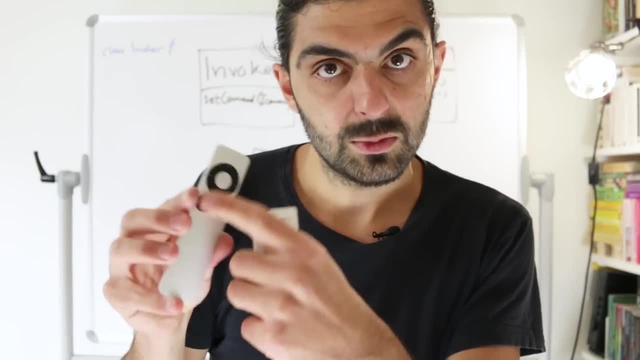 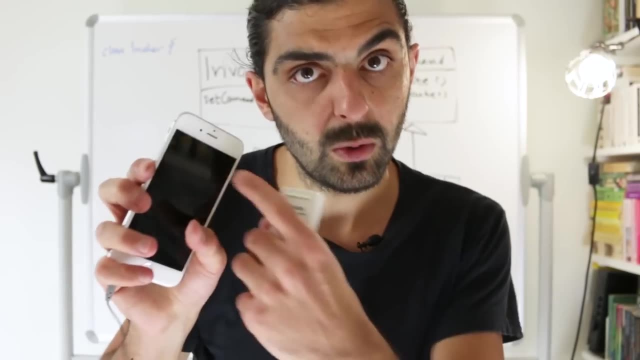 can actually see that that makes a lot of sense because i mean, it would be kind of sweet if this would also function as your home automation control and this would function as your home automation control and you could use the same software in your phone to program both of these. 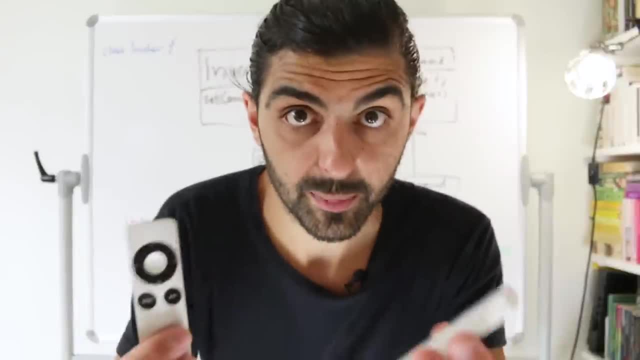 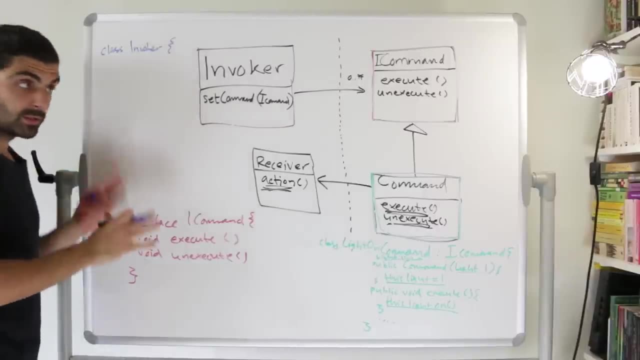 devices or a multitude of other devices again, command pattern is actually massively powerful. so back here. this is why we're saying that the invoker is a class and not an interface, because so far we haven't really had a need to make the invoker an interface. it's not something that needs. 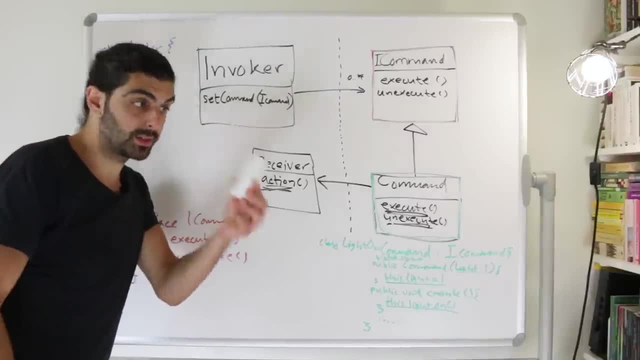 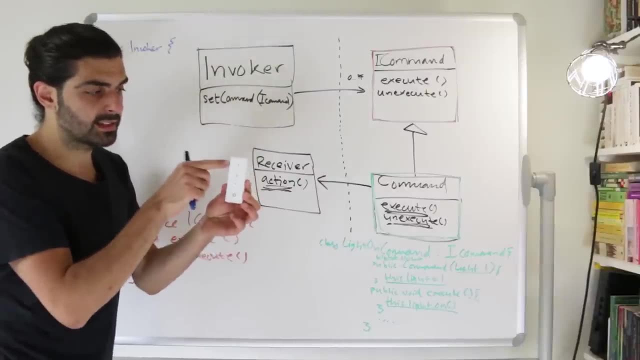 to be shared. so let's say that the invoker, concretely, is this particular device. then we have four buttons and i would actually, rather than put these commands in a list, i would probably make these separate. i would probably say that this is the on button, off button, dim up and dim down. right. 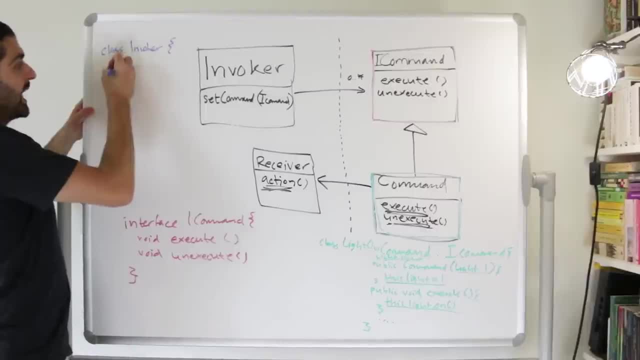 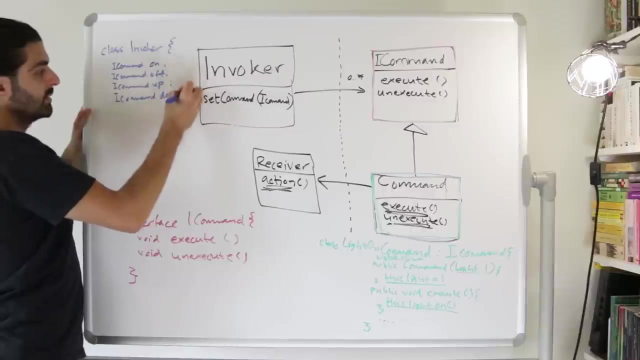 so let's add those as instance variables. so like we have an i command- and actually let me just use a shorter name on, i command on and we have i command off and we have i command, let me just say up and i command down, and these are instance variables. so i should have expressed this in. 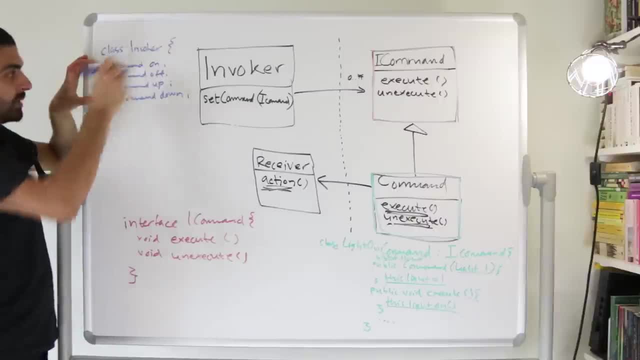 the same order as the buttons on this device for simplicity, but we now express them this way. so we have the instance variable on, which represents the on button, the instance variable off, which represents the off button, and the instance variable up, which represents the dim up button, and the instance variable down, which represents 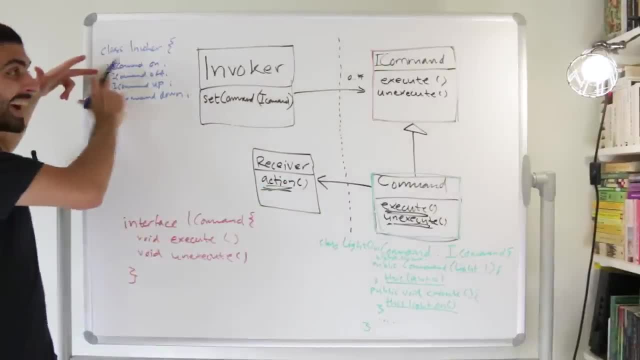 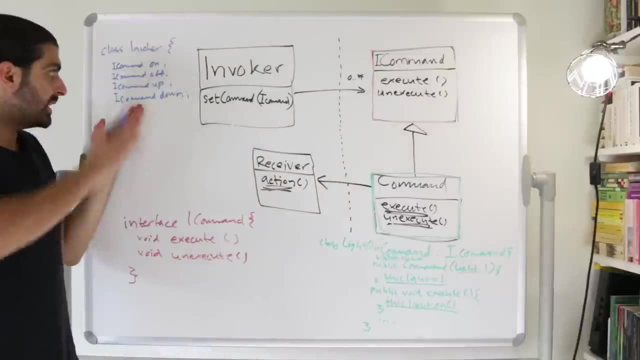 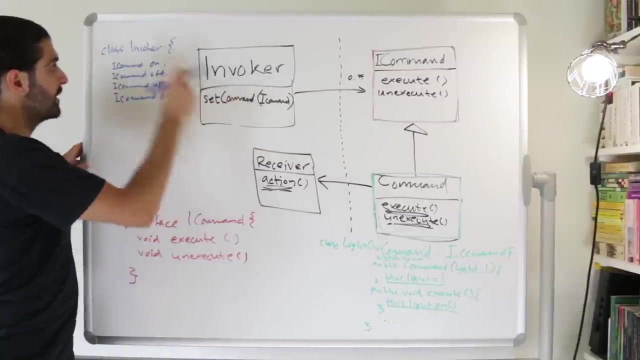 the dim down button and, as you probably noticed, the type of these instance variables is i command. super importantly, they the type is i command, because these represent what we want to do whenever that button is pressed. so in the book they use this set command method. so the the invoker. 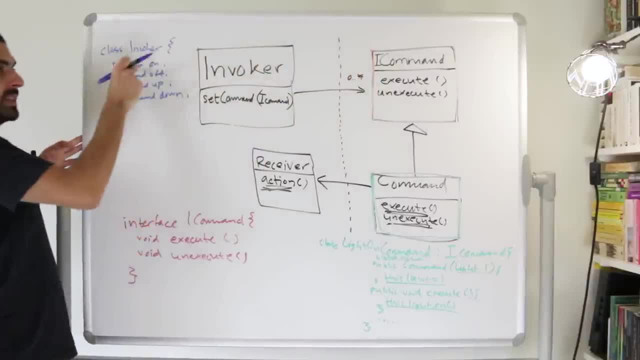 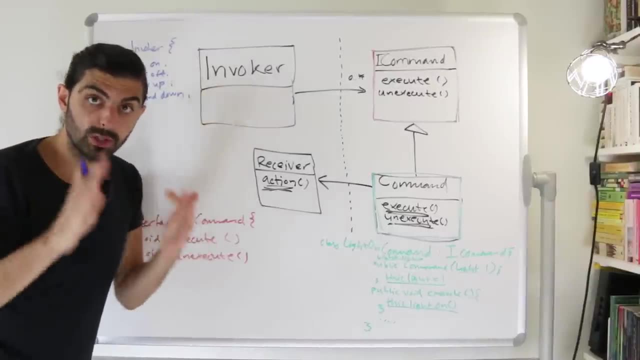 class has a set command method which takes a command and then puts it in one of these places. i actually think that that's a really bad idea from this perspective. if you can avoid mutation, always try to avoid mutation. i see no reason yet for why the invoker should have to have a set. 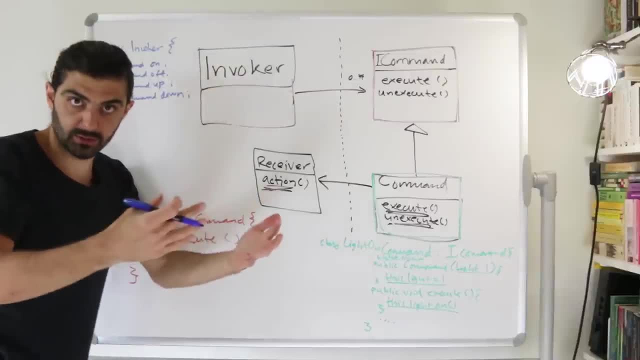 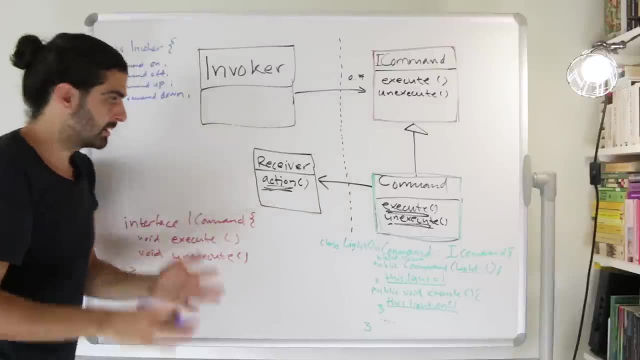 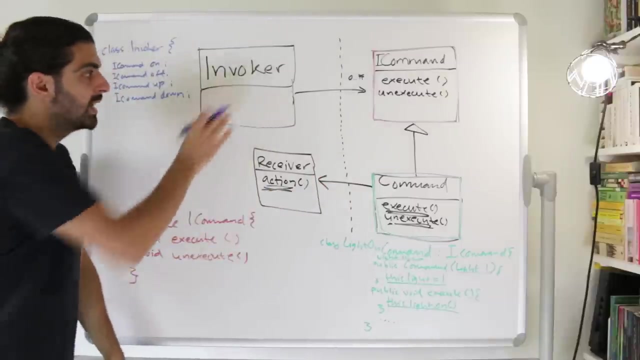 command method. i would rather pass the commands through the constructor. the invoker necessarily needs four commands. so an invoker with three commands doesn't make any sense in our case. so the invoker should be instantiated, and upon instantiation we pass it four commands. now, of course. i mean you could argue. 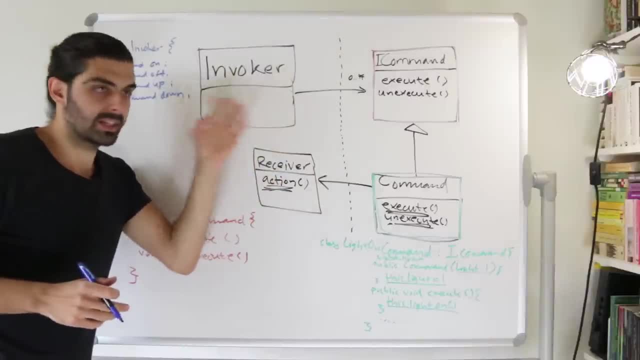 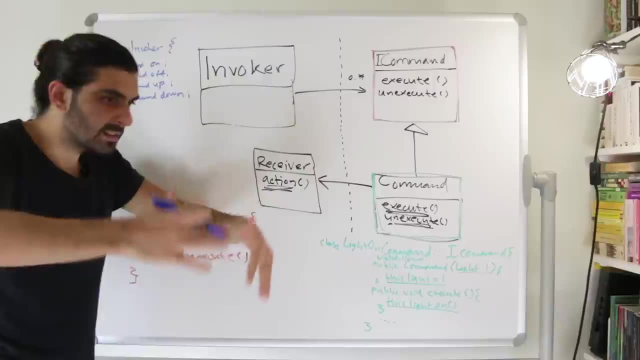 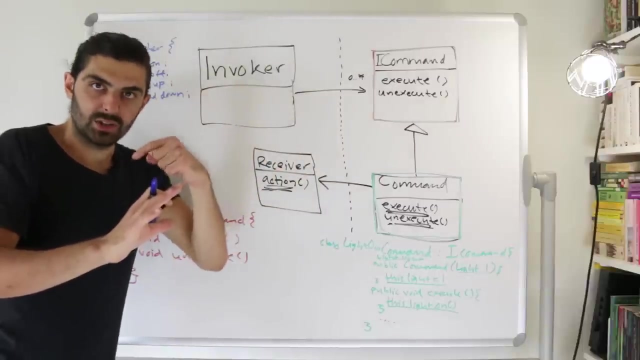 that when you're building a queue, for example, you would probably want set command, because then you have your invoker is add to queue, right, you add a command to the queue and then you actually need to mutate the queue unless you have a queue that when you say add, you get a new queue back which 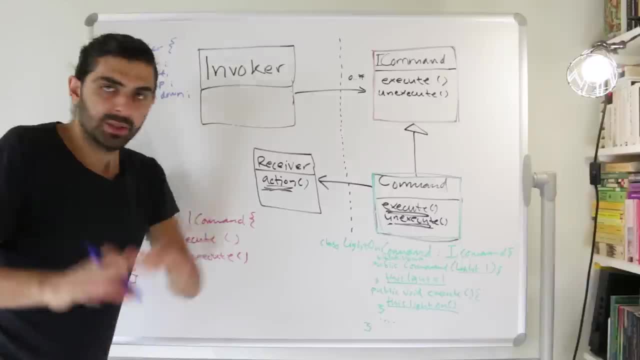 contains all of the commands that you need to add to the queue, and then you actually need to add a new queue back which contains all of the old commands plus the new command. but this is a long and completely different story and if you're interested in that discussion, i would recommend. 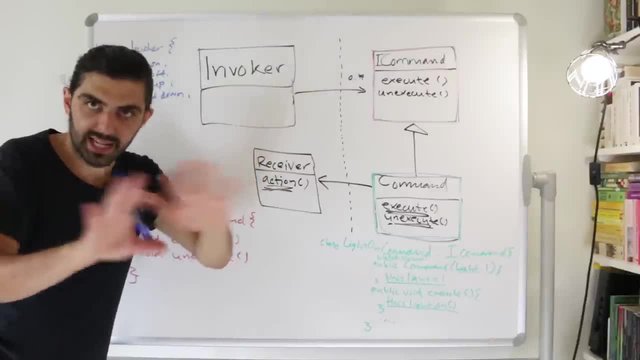 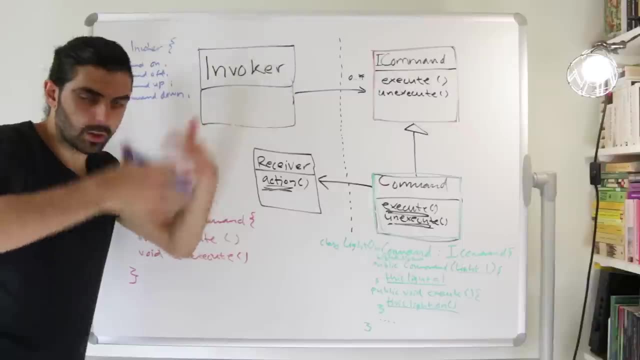 that you check out gary bernard's talk boundaries, but that has nothing to do with what we're doing here. but the point here is that we can avoid the mutation. we can avoid, uh, changing the the contents of the invoker as the program is running. we could rather just create new invokers whenever we need. 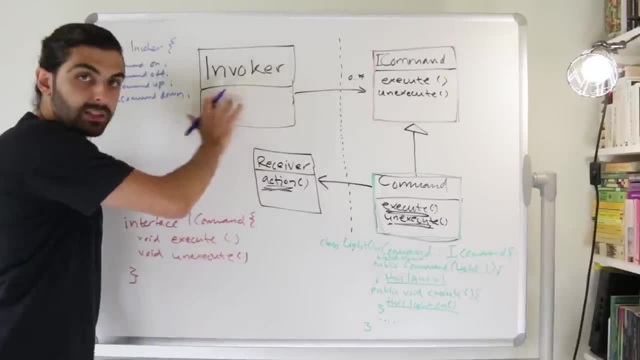 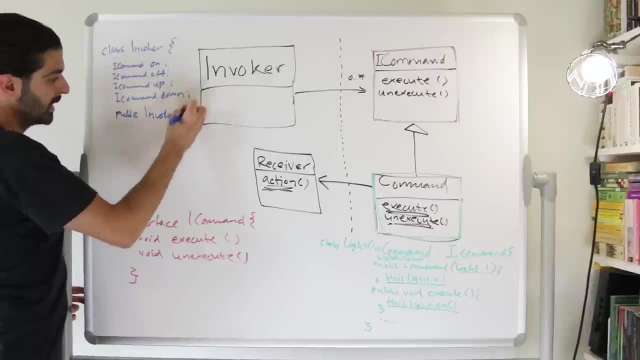 an invoker, which i would argue makes more sense, which is why we remove the set command method and instead we just say that the invoker needs to have a constructor, so let's say public invoker. i'm just going to use two lines here and it will take four arguments. it 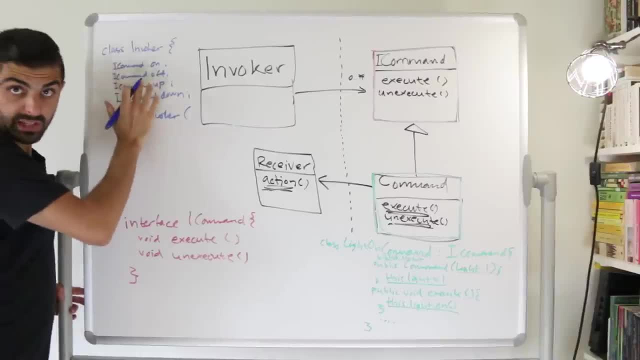 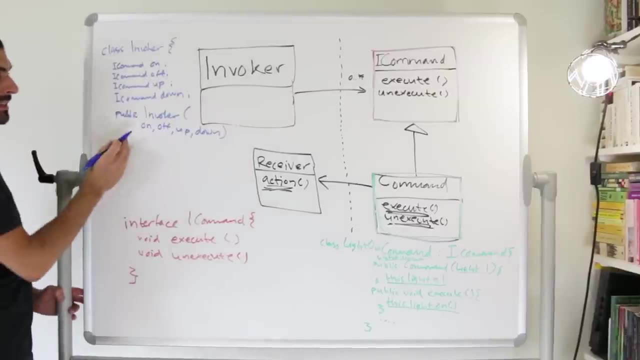 will take all of these four as arguments. so it will take. in order to save space, let me just not express the types here. but it would take an on, an off, an up and a down. i'm not expressing the types, but this should say: i command on, i command off, i command up, i command down. so the invoker takes. 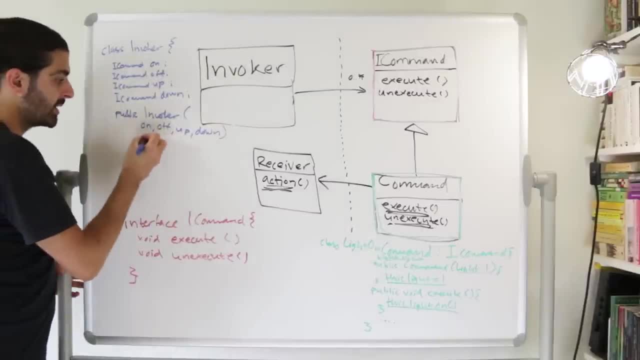 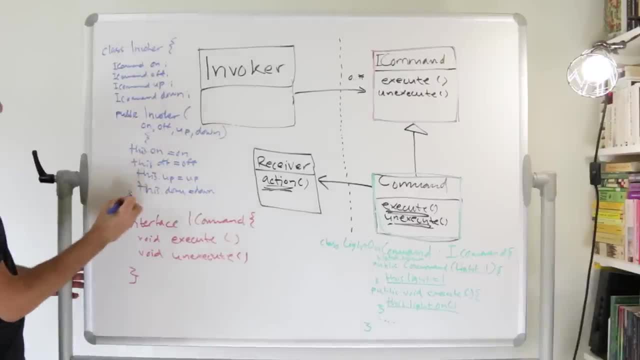 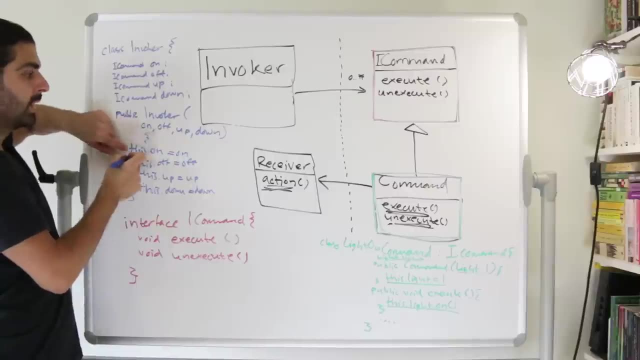 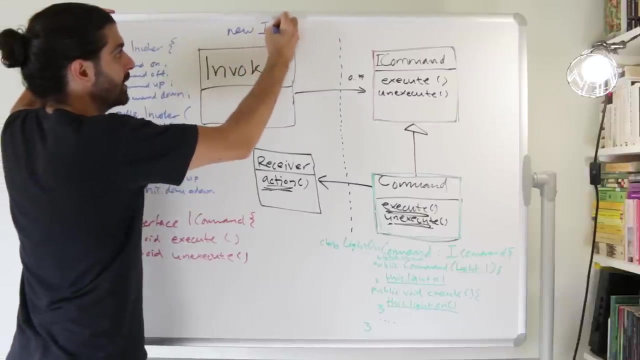 for up and for down and then we close the constructor. so whenever we instantiate the invoker, it now has access to- in this instance, variable- a command that represents the on action. so whenever we say new, let's actually do that. let's say new invoker, we pass it a bunch of. 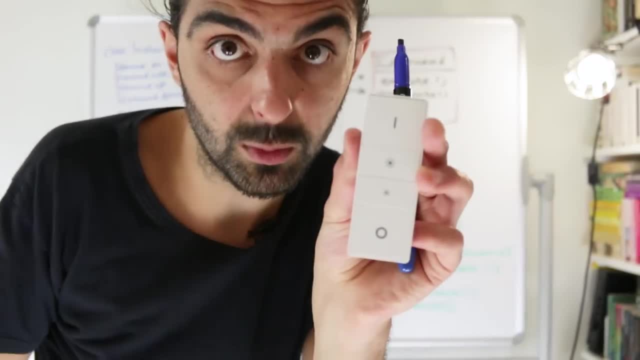 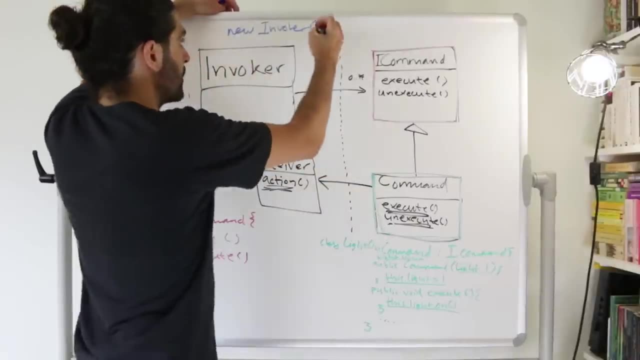 commands and for the on button. we probably want an on button, so we pass it a bunch of commands as an on command, like an light on command. so let's, then we would say we would use this one, the light on command, so we would say new invoker and then we pass a new light on command and to 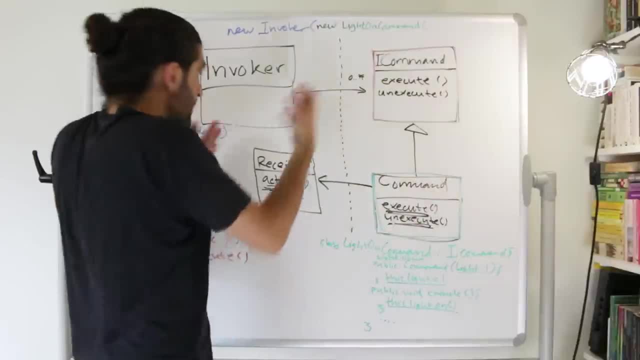 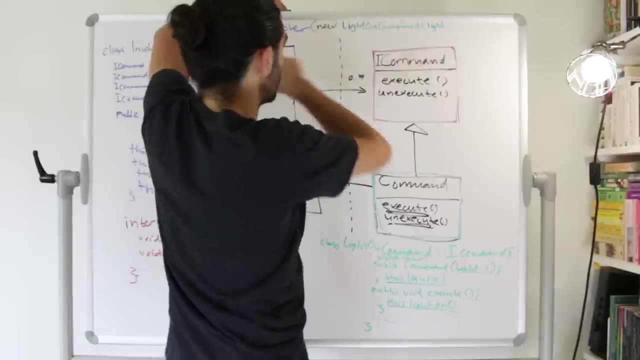 that we would have to pass the light, this light, and now we don't have that. but let's assume that we have a light called a light with a lowercase l in in the scope where we're at, when we're calling this particular, when we're executing this particular line, and then we close that. so the new 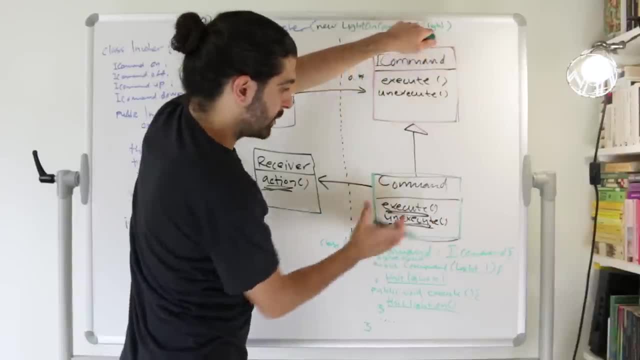 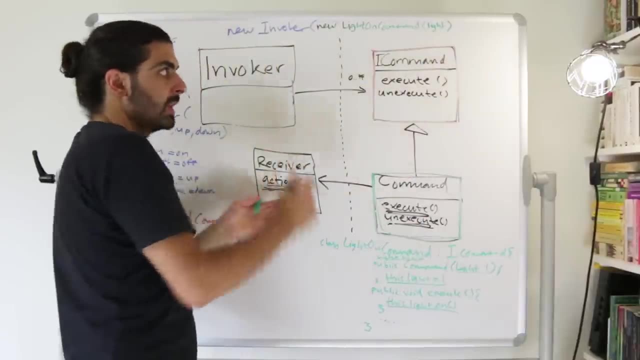 light on command gets passed a light because, in order to avoid that, we have to pass a light on. to be a proper command, this command, this light on command, needs to have access to a light that it's operating on and that light is a receiver. 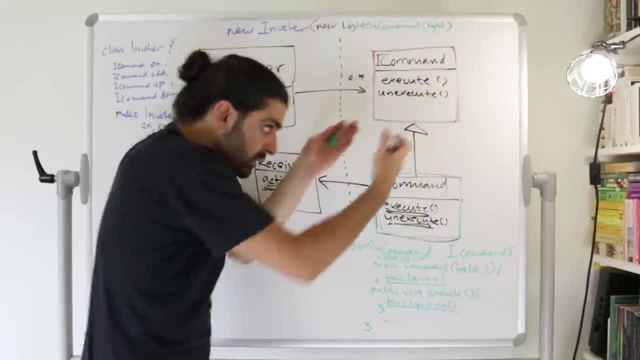 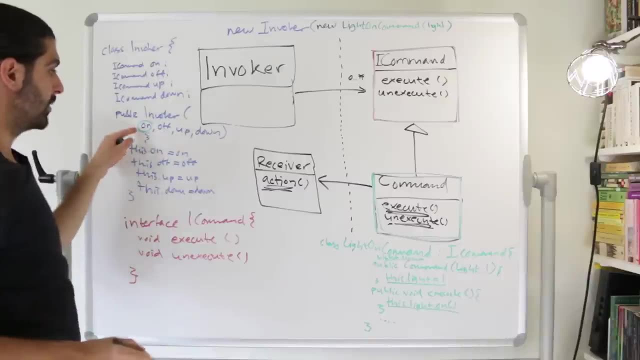 So we're passing that light to the light on command, and then we're taking that light on command and we're passing it to the invoker. To the invoker as its first argument, because its first argument is the on command. So then when the invoker will call, execute. 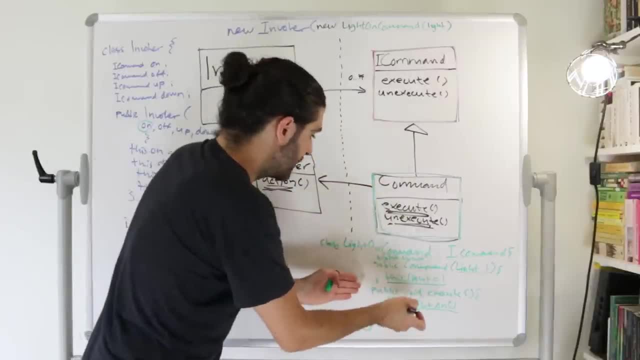 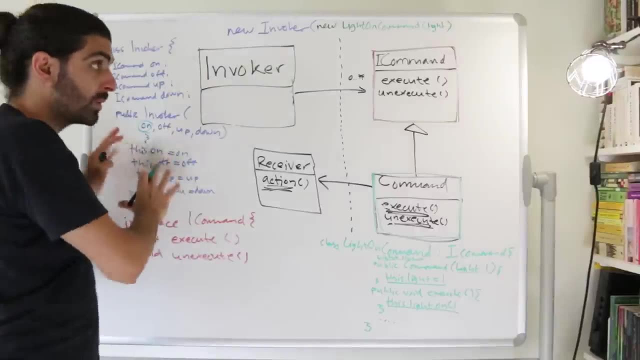 on the on command, we will execute the light on command which will call on on the receiver which will turn the light on. So, again by proxy, the invoker has the capability of turning this light on. And then, of course, up here, 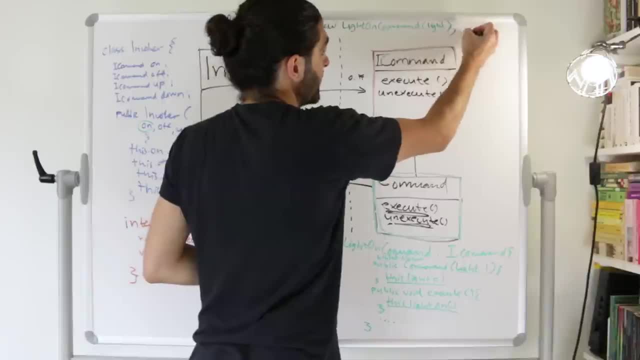 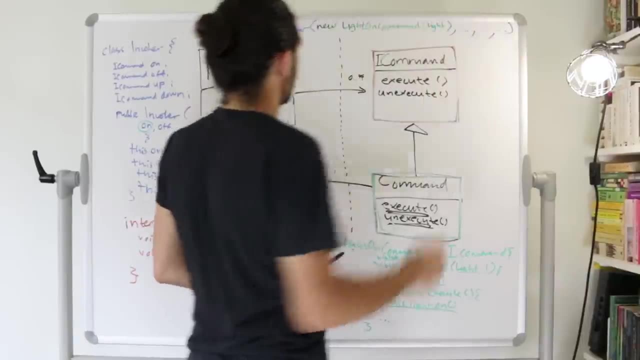 when we instantiate the invoker, we would have to pass the next command and the next command and the next command, one, two, three, four, which is on off, up and down, and then we can close that. 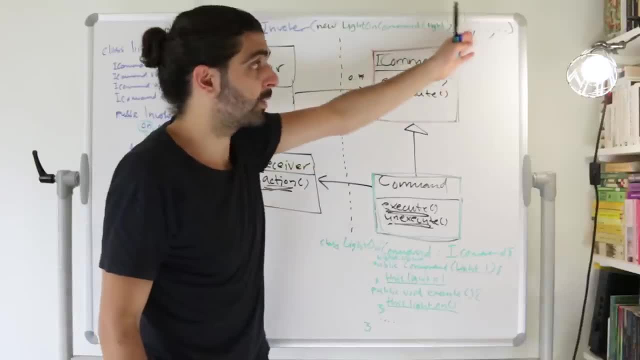 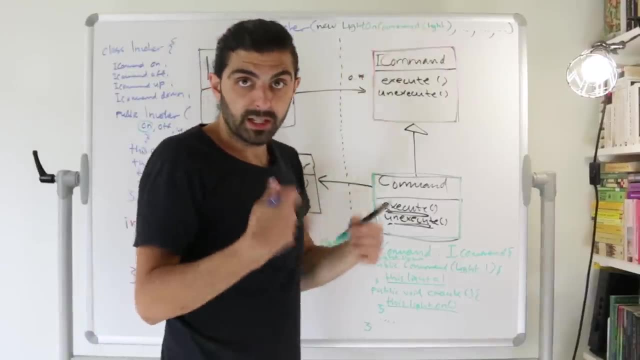 because then we have a complete invoker. Now we haven't constructed commands for off and up and down, but I think you can see sort of how we would do that. But again, that's also the point of moving this set command or removing this set command method. 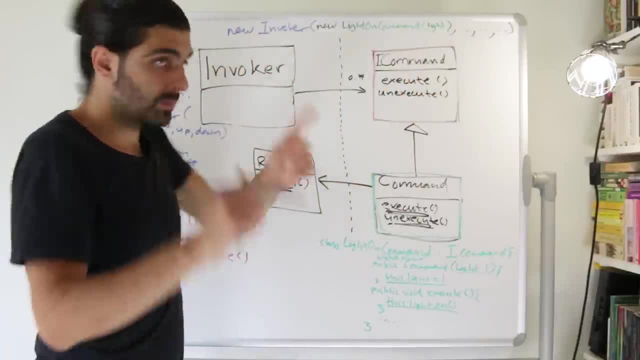 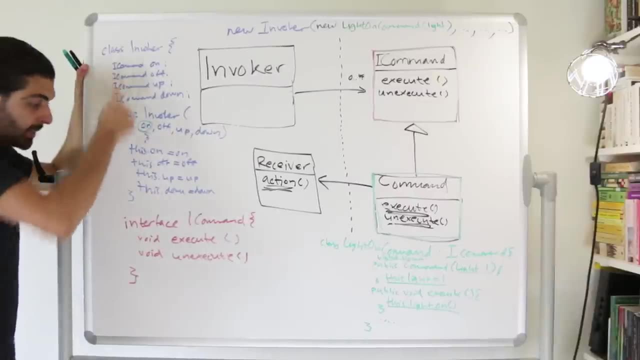 and making it part of the constructor instead, because that means that it's now impossible to create an invoker which doesn't have all the commands it needs. So, in order to finish this invoker code, let me just remove this. the interface code. 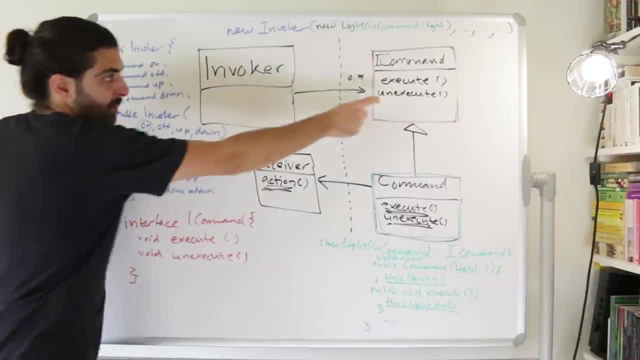 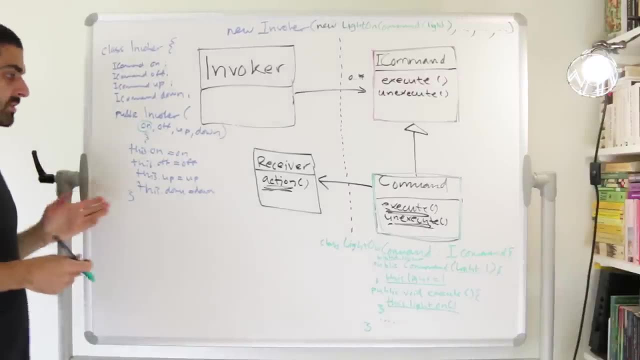 because I think you can remember it and also you can see it here. I mean, this code just represents this interface, So let's remove that and then let's think about this: What is missing here? Well, of course, the invoker needs to be able. 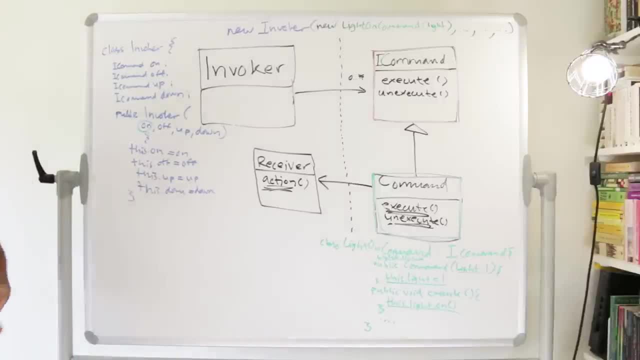 to actually have buttons that are pressed, So probably it needs an on method public void. and, to be super explicit and to make sure that we don't confuse these with the instance variables, let's call them click on and click off, right. 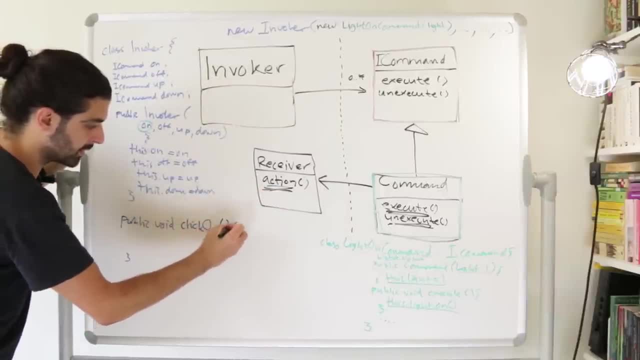 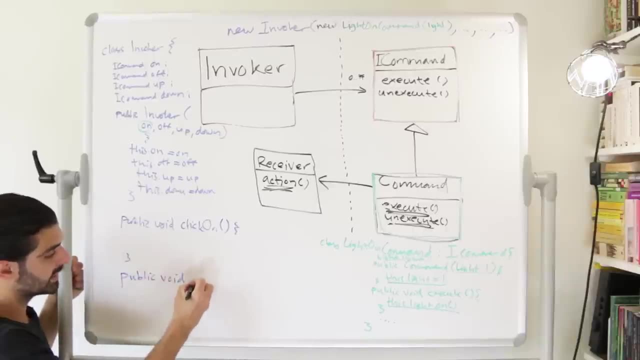 So if we click on, that would be a method that takes no arguments, has some implementation, and we'd have another method called- that's also a public method- returning void, and it is called click off. Should probably have called this pressed, but whatever. 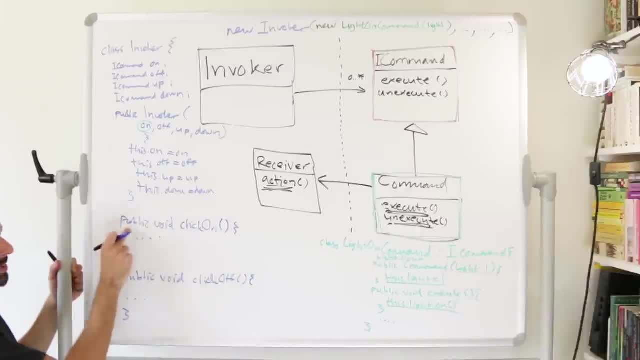 And then what's the implementation here and what's the implementation here and et cetera? because now we just created the two methods, click on and click off, but we also need to have click up and click down. But click on super simple would essentially just say: 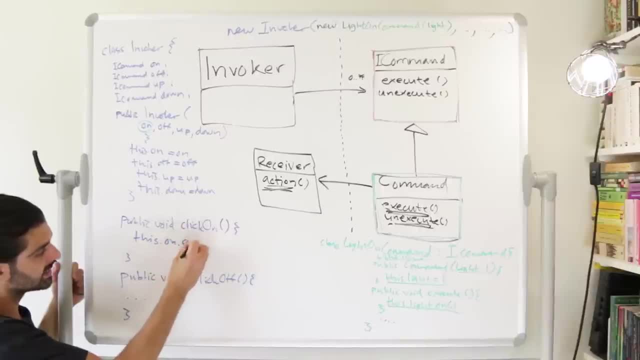 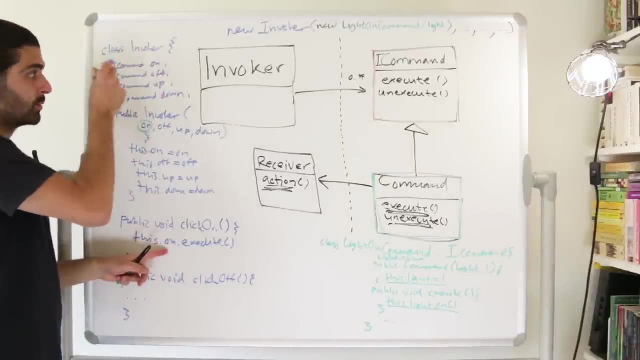 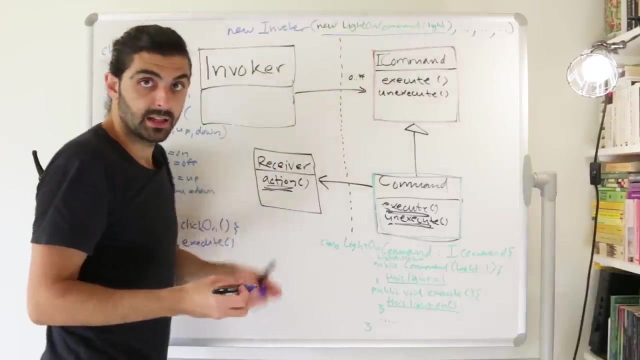 this dot on dot execute, In other words, in this instance, variable on. we have stored a command. In our example here we happen to store the new light on command which is past the light. So whenever we call execute on this particular on command. 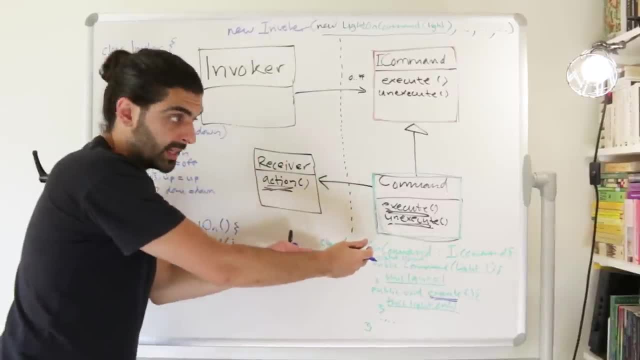 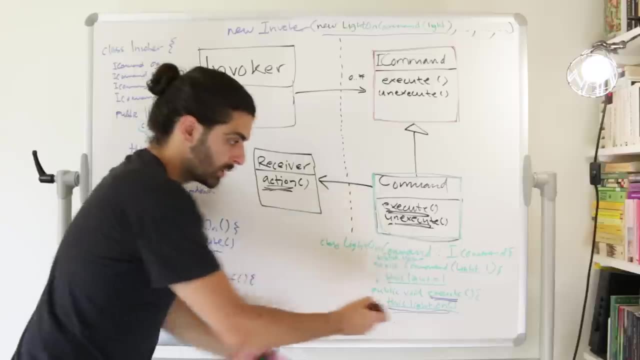 we will do whatever is in this execute method of that light on command. And in our case it happened to be that the body of that method says that we will do this, dot, light, dot on. In other words, that the light on command calls the method. 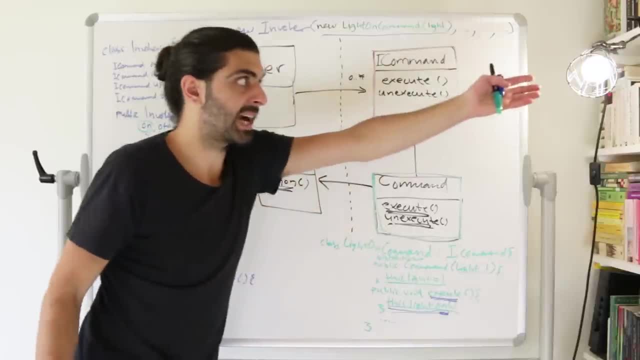 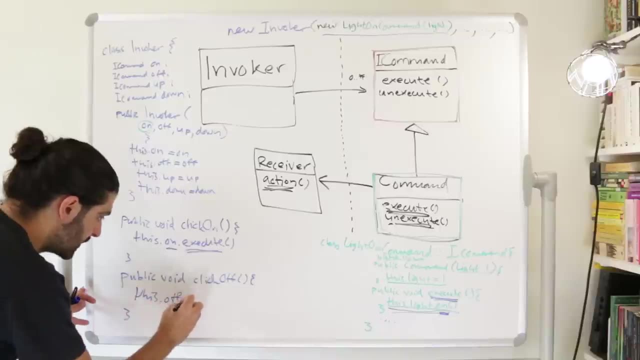 on on the light that it has in its scope, And that light happened to be this light. And that's all for click on. And then the same thing we do for click off. So we would say this: dot off, dot, execute, And exactly the same thing happens. 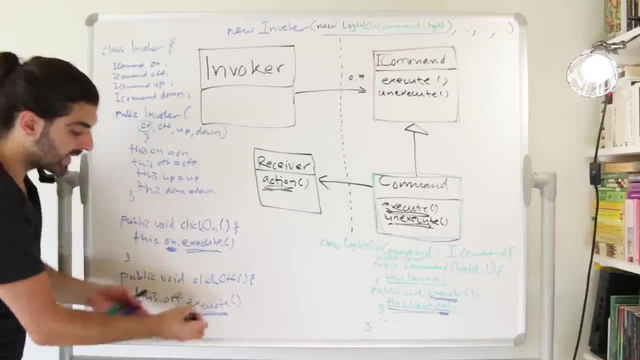 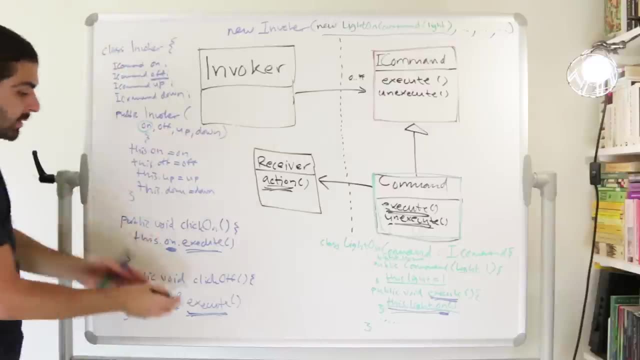 but instead of that we call execute on the on command. we now call execute on the off command. So we also have an instance variable which is called off in our scope And that off command. we then call execute on that off command, which would be this command: 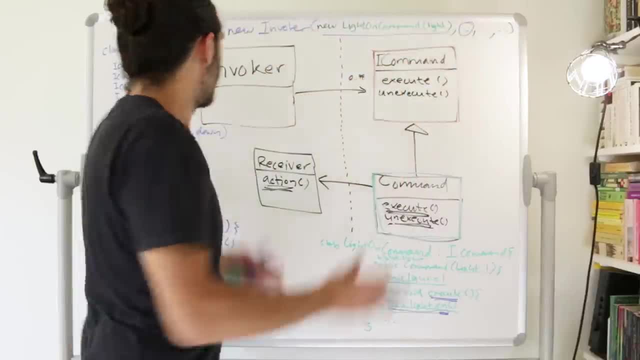 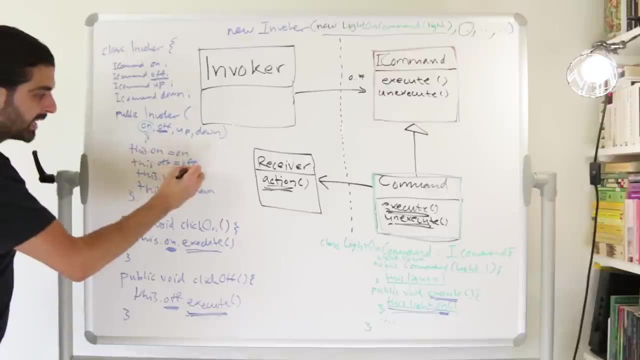 that we passed here, But we haven't actually specified what this command is. But that would be the second argument that we've passed to the invoker, Because the second argument of the constructor was the off command. That's the thing that we hear saved off. 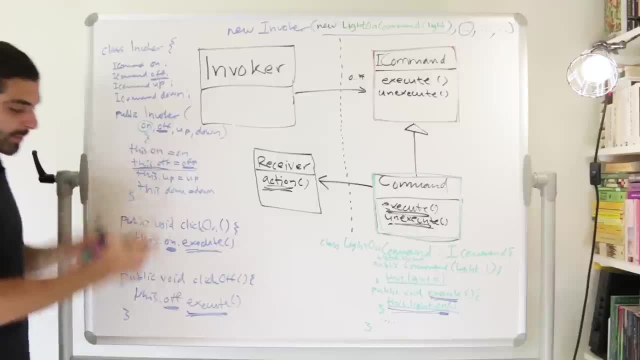 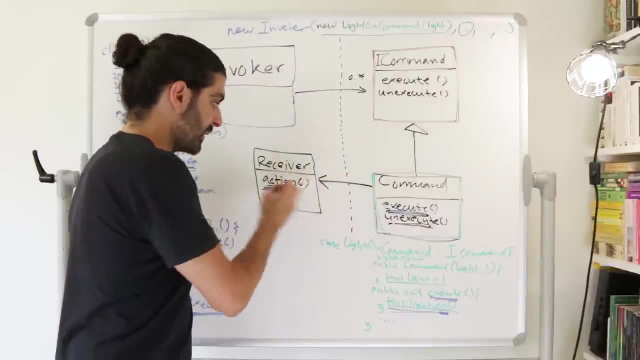 into the instance variable called off. So we would then call execute And again that would mean that we call execute on that particular command which then would act upon some particular receiver by, for example, calling some particular action. So if we imagine it would be a light off command. 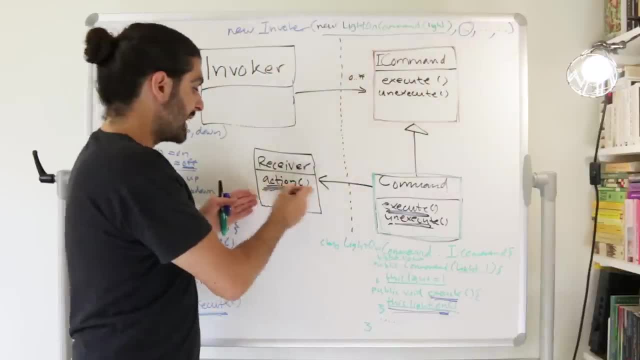 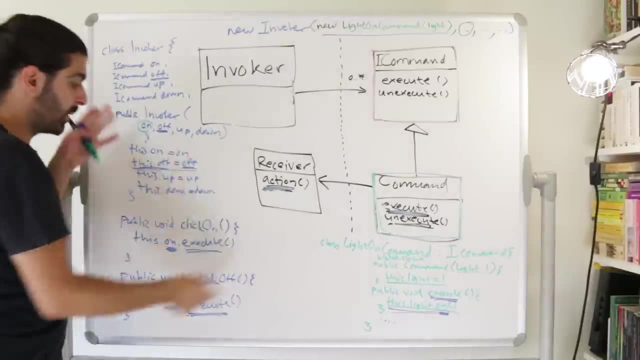 and we would also pass a light and we would pass this light. then the action would probably be to call off on this particular light And that's it. Now. we just keep on going like this. We just keep on creating invokers and stacking commands. 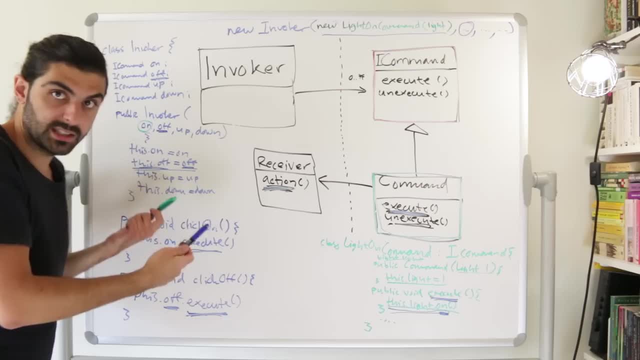 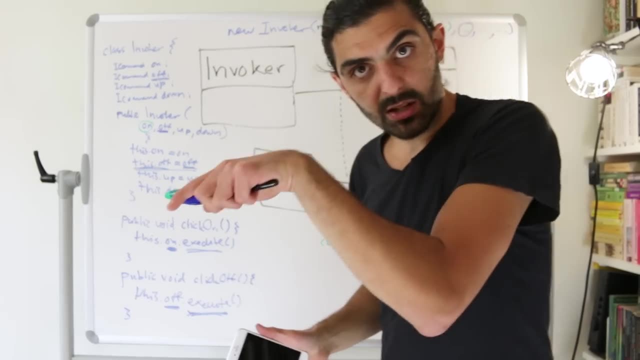 And the key point is that, of course, at runtime we don't want to bury these commands. So if you're building an application, if you're actually building the app that users use to say that when I press this particular button. 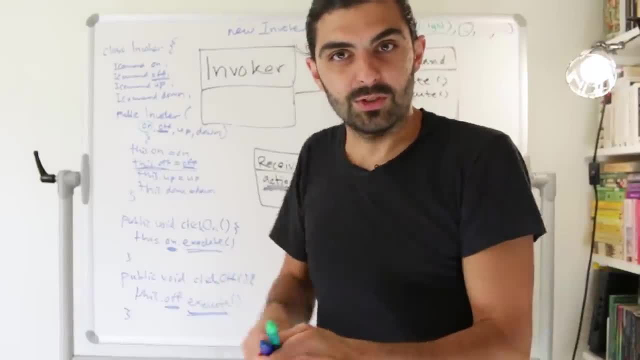 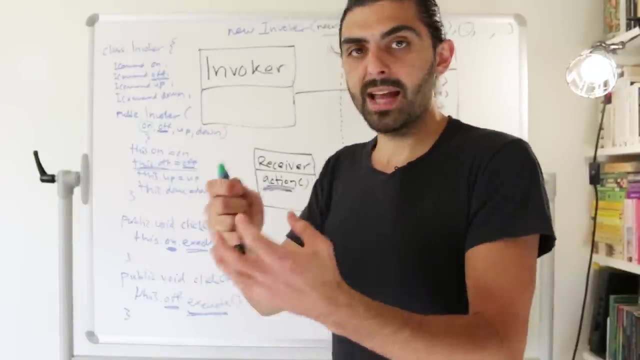 I want this particular series of commands to be executed. you can then give the user a bunch of different commands and then let the user choose which command should be coupled to which button or which command should be put onto which button so that when the user presses that button, 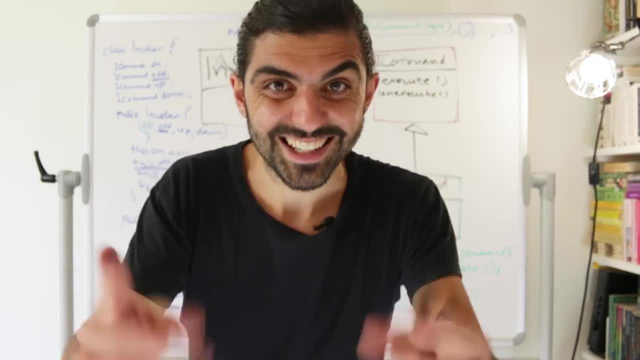 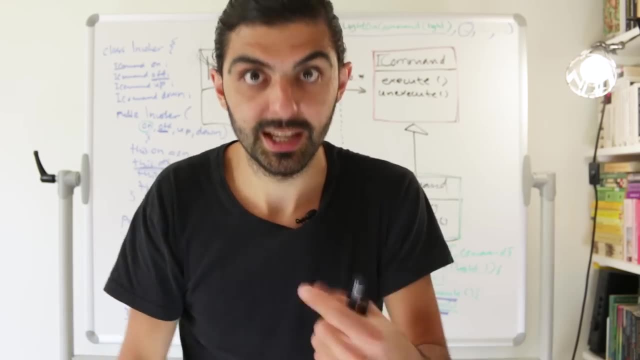 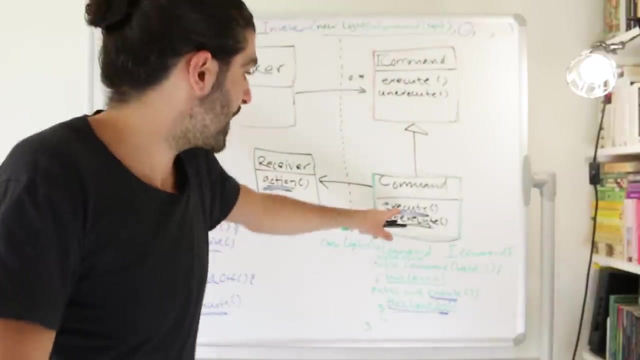 you actually execute that command. And then two points. One: undoing becomes super easy because every command now has an unexecute method. And two: you can now construct macro commands because you can now have commands that contain multiple commands. So if the command, when you call, execute, 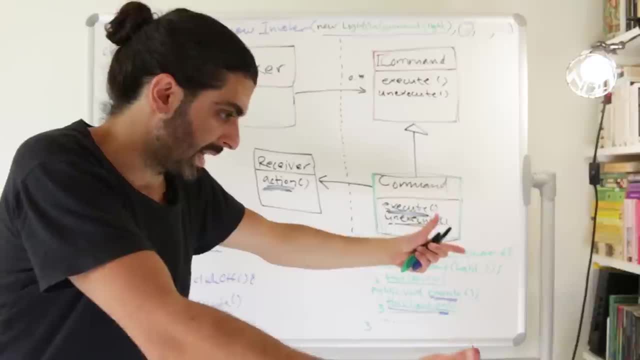 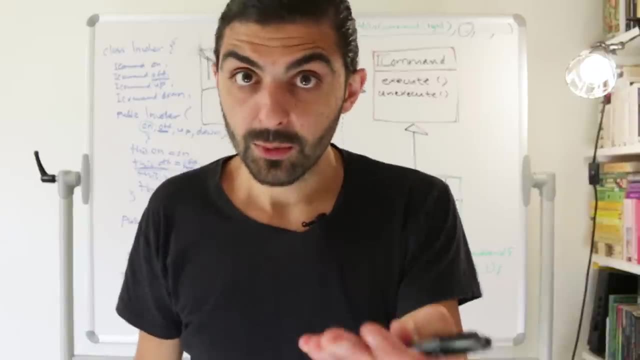 if it doesn't immediately act on a receiver, but rather it has multiple commands that it calls execute upon, then that command would be like a macro command that can do multiple things, And this is one way in which you could implement the whole notion about turning on or off multiple lights. 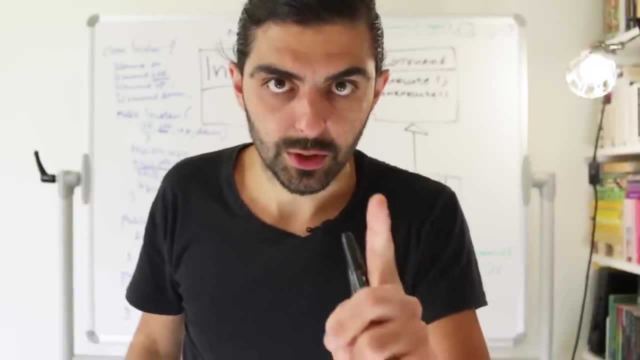 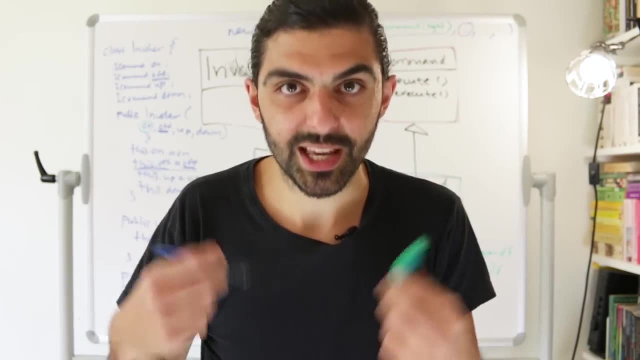 instead of a single light. To wrap up, let's talk about this whole undo notion. So this really clicked for me when I started to think about Photoshop. Think about the image editing application Photoshop. In Photoshop, you have a long series of undo history. 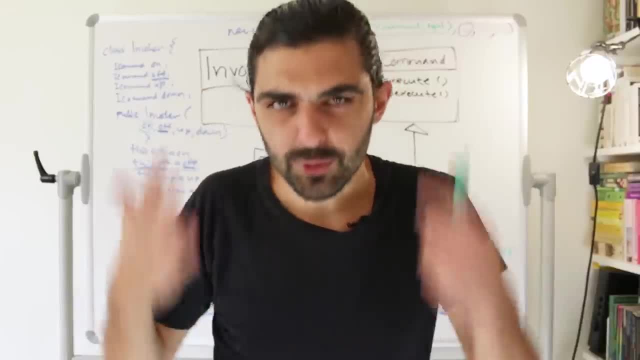 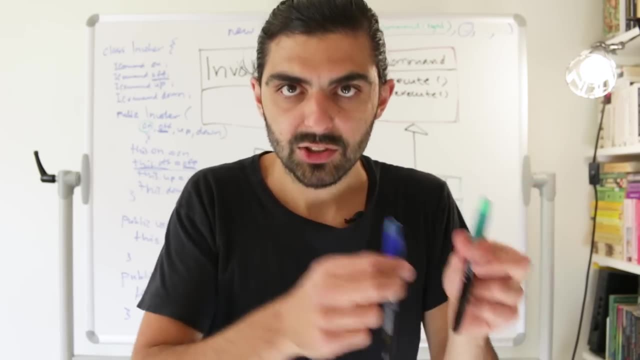 So you can actually go. you can roll backwards a super long way, And if you just think about how you would build that programmatically it would probably not be super easy. But if you think about it this way, what if every action that you perform upon your picture? 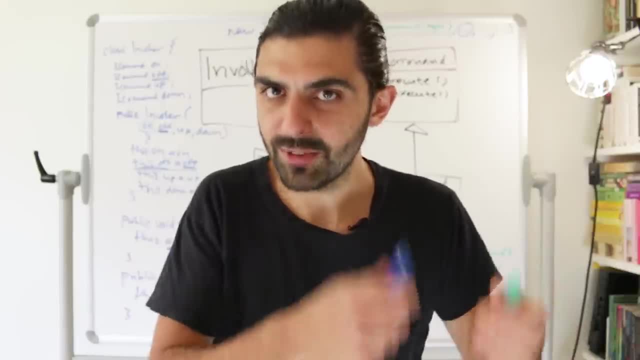 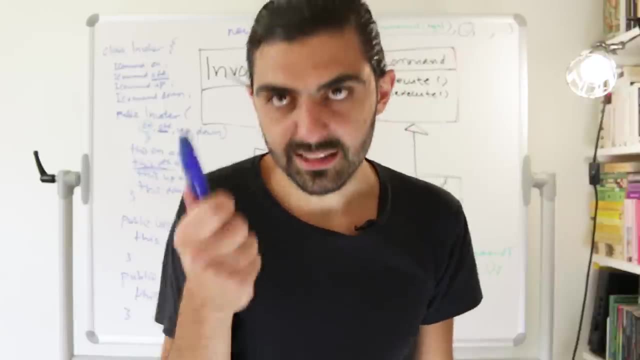 every action that you perform upon your document is a command. What if everything is a command? And what if all of these commands are rollbackable right? What if all of these commands have execute and unexecute? What if you can do the command? 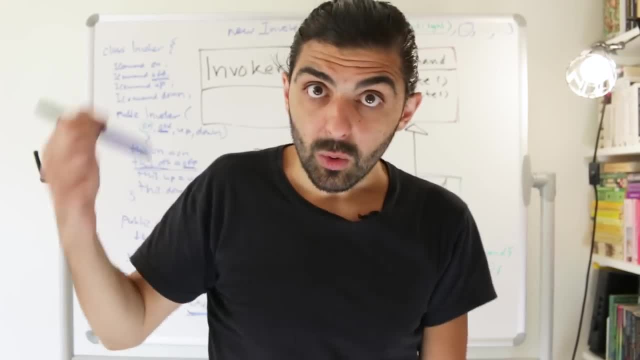 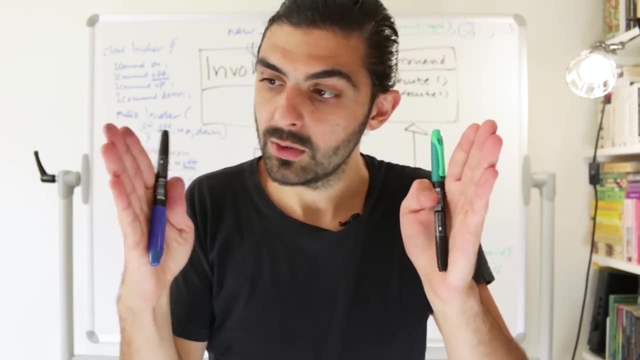 and then you can undo the command. And what if you then just stack all of the commands that the user performs to a document into a list And then, whenever a user wants to undo, you just do unexecute on the last command and pop it off the list? 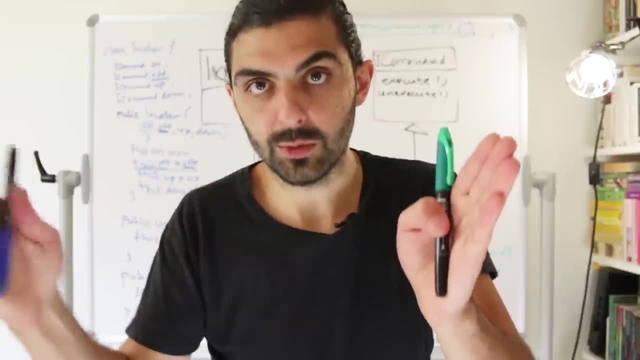 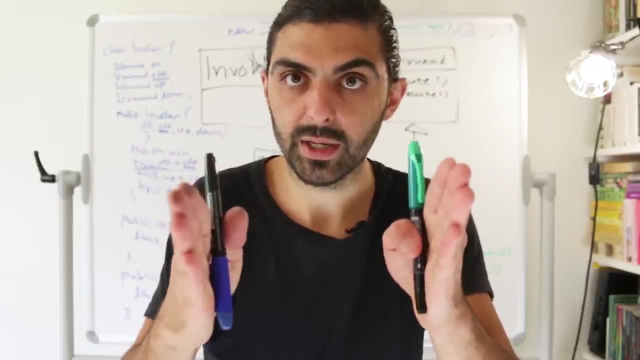 Or if you don't pop it off the list, you would just call execute again to redo right. So you say undo, You unexecute the last command And then you undo again, You unexecute the command. after that You undo again. 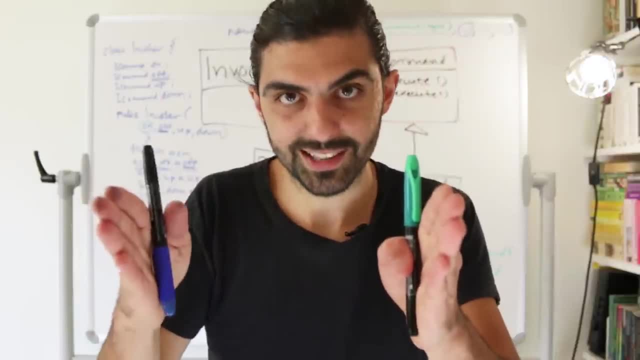 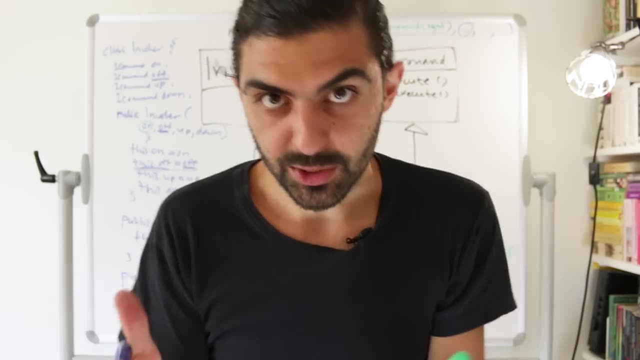 You unexecute the command. after that Then you redo, Then you execute that last command that was unexecuted, And so forth. Then you can go back and forth in history kind of trivially. I'm not saying at all it would be trivial to build Photoshop. 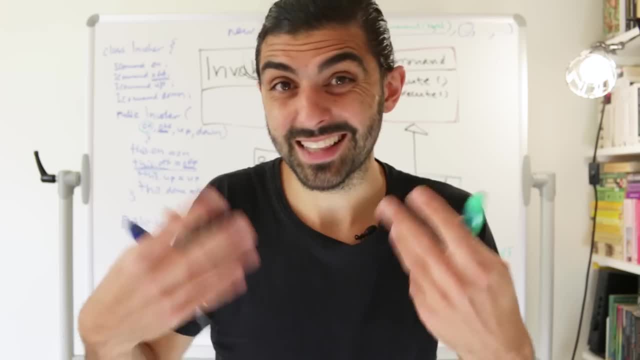 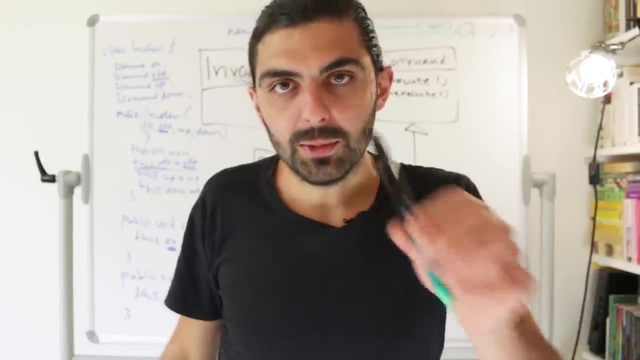 because the more difficult parts is of course to figure out what would actually happen in that execution. But the whole notion about doing and undoing would then be kind of trivial, And I would actually say that this is kind of an elegant way of structuring your programs. 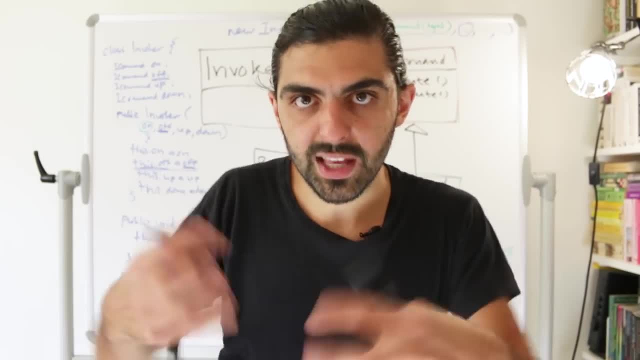 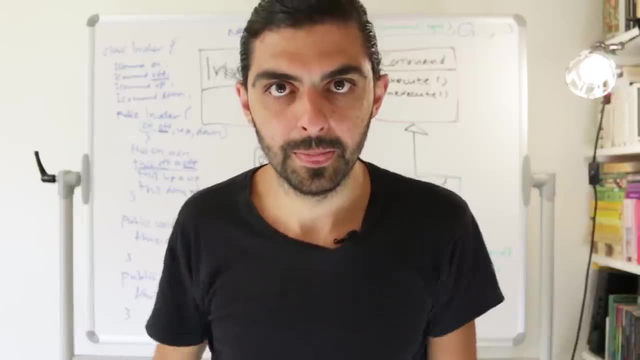 So instead of just performing some action, you wrap the action that you want to perform in some particular command and you make sure that that particular action is undoable. So this was the command pattern. I hope that helps. Please make sure to ask in the comments. 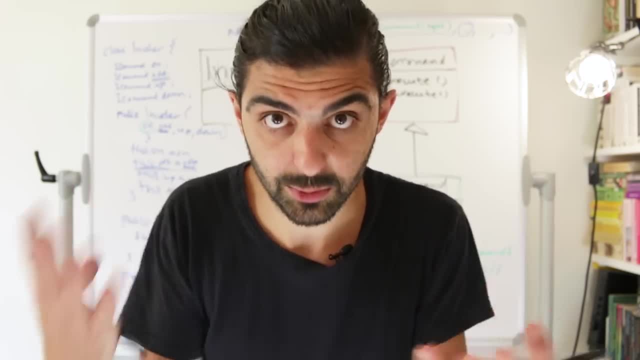 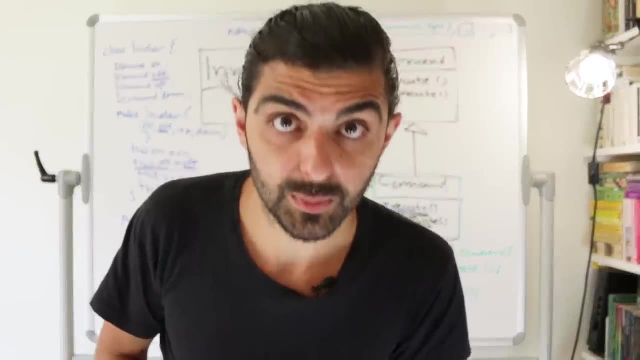 if you have any sort of questions or comments, or just share your thoughts and ideas. if you have something to share, It'd be massively appreciated. Beyond that again, if you're new to design patterns, get this book, And if you want a reference book for design patterns,